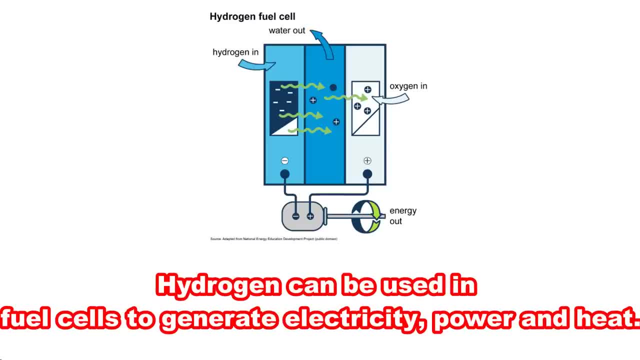 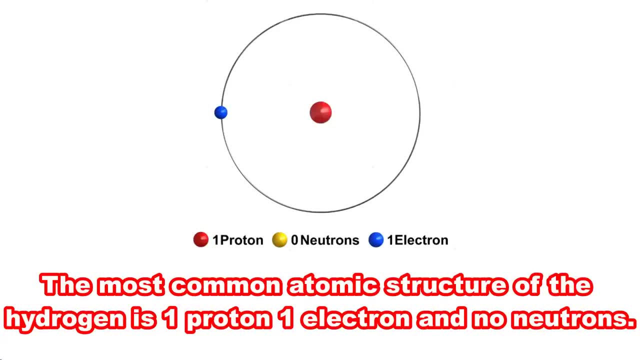 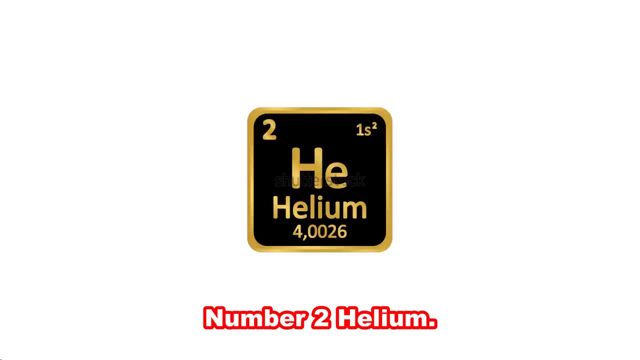 matter. Hydrogen can be used in fuel cells to generate electricity, power and heat. The most common atomic structure of the hydrogen is one proton, one electron and no neutrons. The price of hydrogen is about two dollars per kilogram. Number two: Helium. Helium is a colorless and odorless noble gas. It is the second. 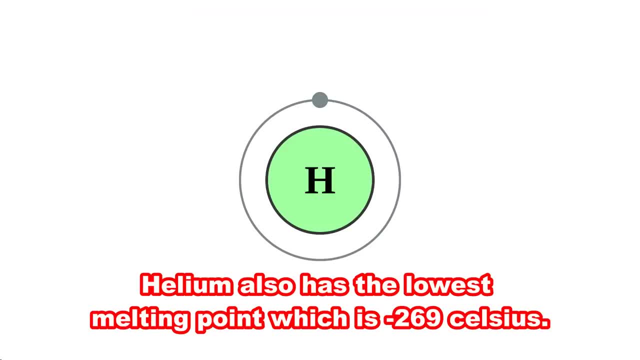 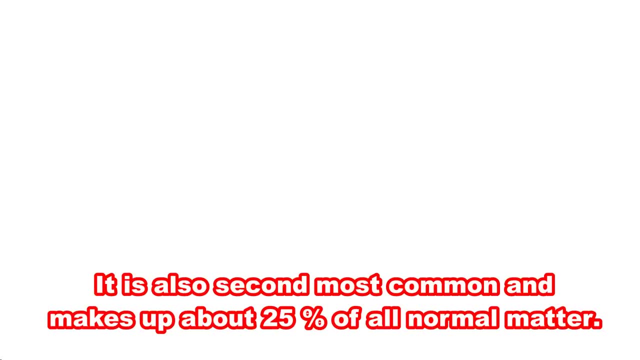 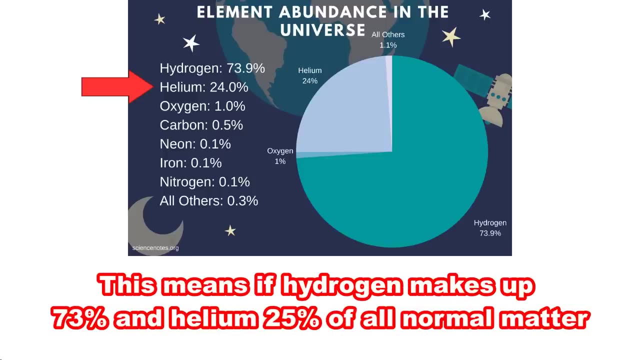 lightest, which makes sense. Helium also has the lowest melting point, which is minus 269 Celsius. Not only is it the second lightest, it is also second most common and makes up about 25% of all normal matter. This means, if hydrogen makes up 73% and helium 25% of all normal matter, only 2%. 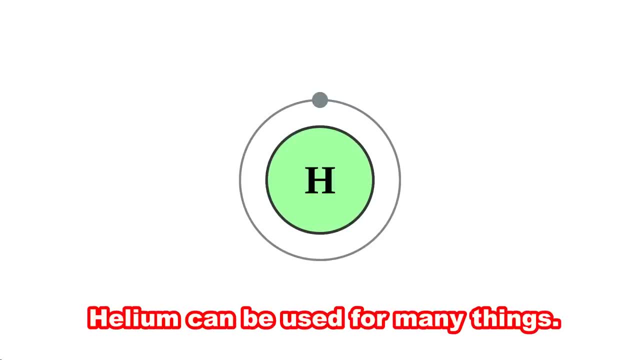 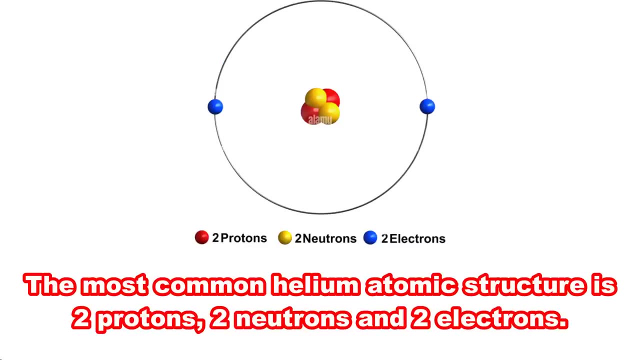 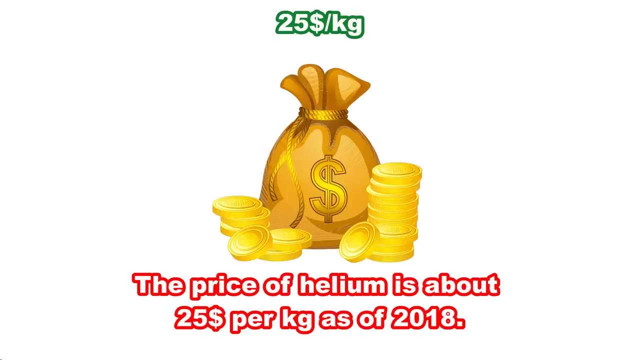 is left for all the other 116 elements. Helium can be used for many things, But probably the most known thing is balloons. The most common helium atomic structure is two protons, two neutrons and two electrons. The price of helium is about 25 dollars per kilogram. 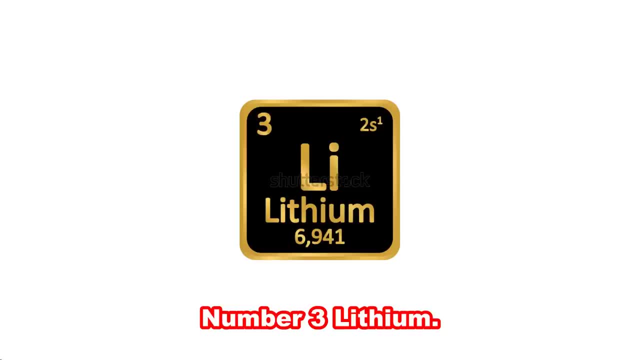 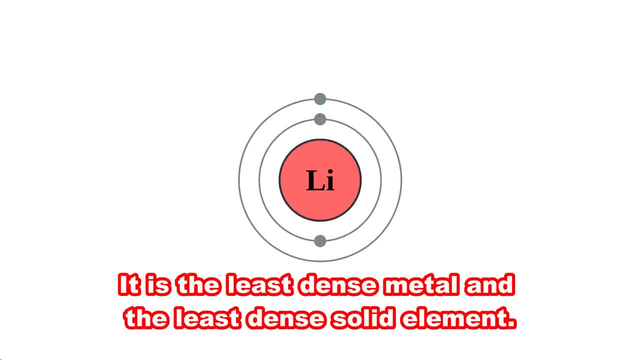 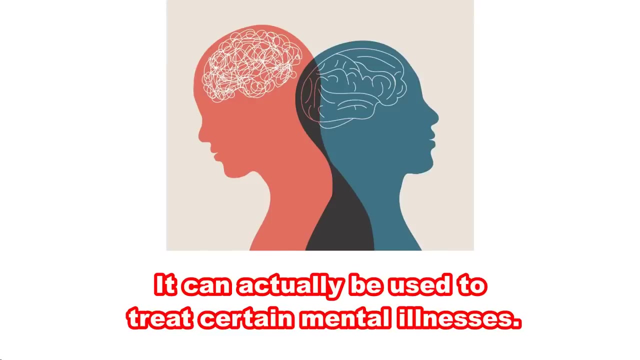 as of 2018.. Number three: Lithium. Lithium is a soft silvery white alkali metal. It is the least dense metal and the least dense solid element. It is highly reactive and flammable. It can actually be used to treat certain mental illnesses The most. 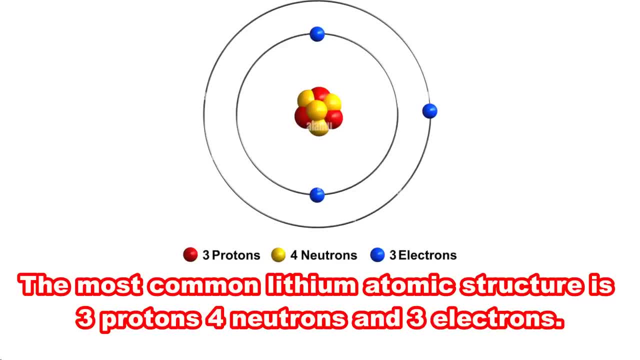 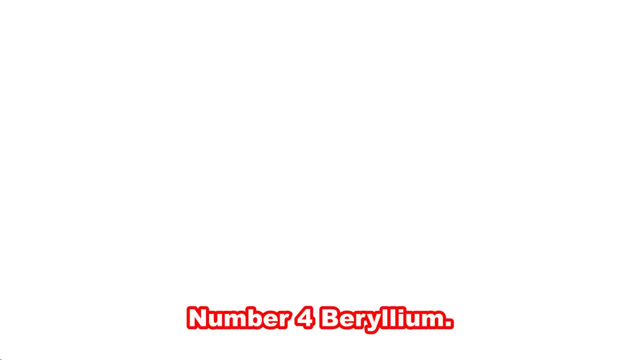 common lithium atomic structure is three protons, four neutrons and three electrons. The price of lithium is about 80 dollars per kilogram as of 2020.. Number four: Beryllium. Beryllium is a steel gray, strong, light and breakable alkaline. 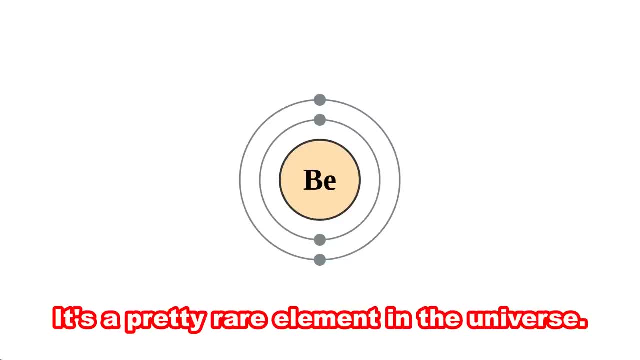 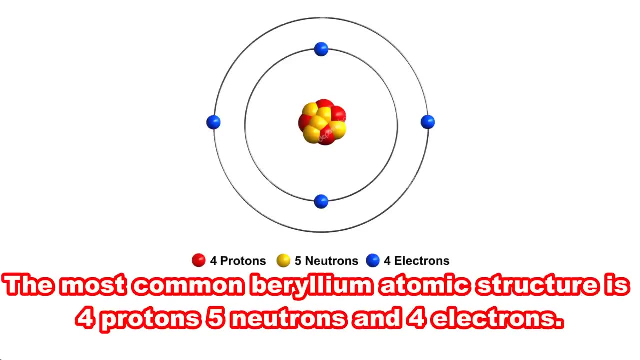 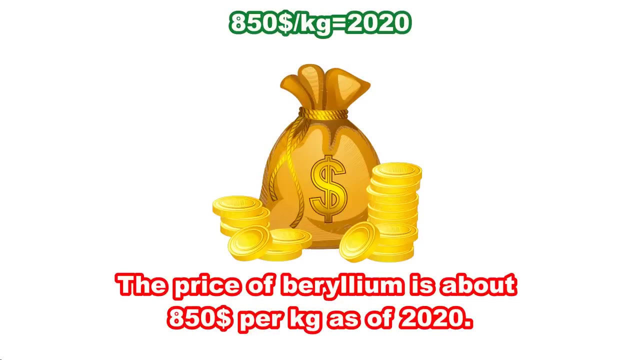 earth metal. It's a pretty rare element in the universe. Beryllium is used for gears and cogs. The most common beryllium atomic structure is four protons, five neutrons and four electrons. The price of beryllium is about 850 dollars per kilogram as of 2020.. 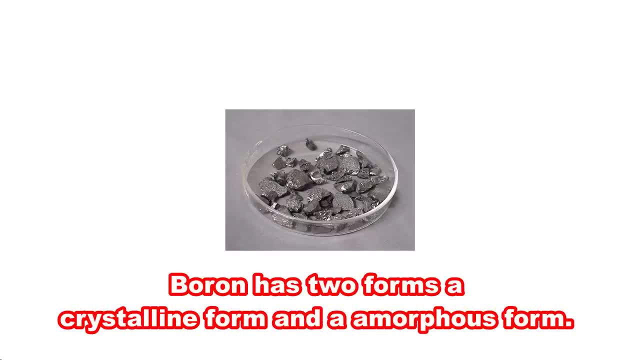 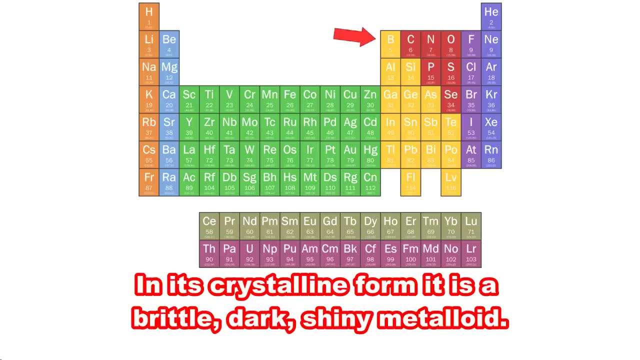 Number five: Boron. Boron has two forms: a crystalline form and a amorphous form. In its crystalline form it is a brittle, dark, shiny metalloid, and in its amorphous form it is a brown powder. Boron is good at building up the human body. 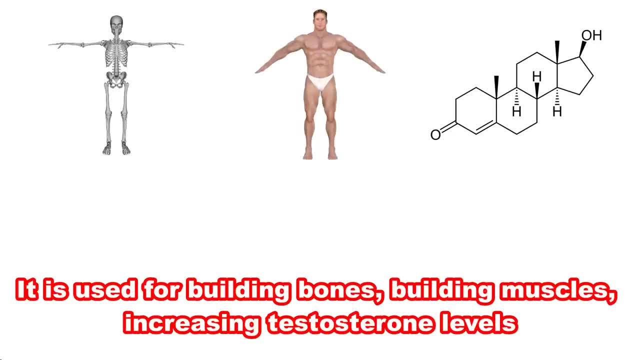 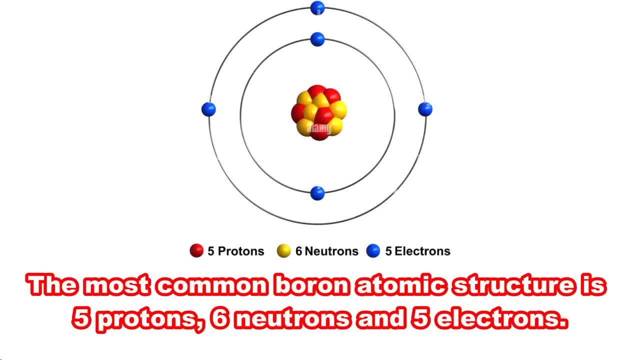 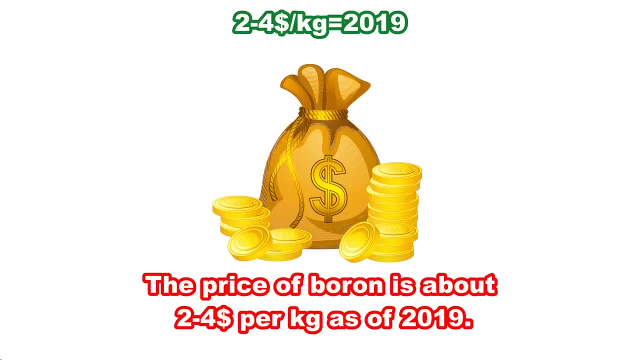 It is used for building bones, building muscles, increasing testosterone levels and for improving skills. The most common boron atomic structure is five protons, six neutrons and five electrons. The price of boron is about 2 to 4 dollars per kilogram as of 2019.. 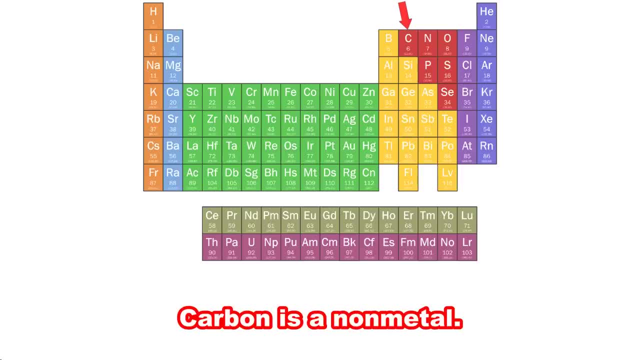 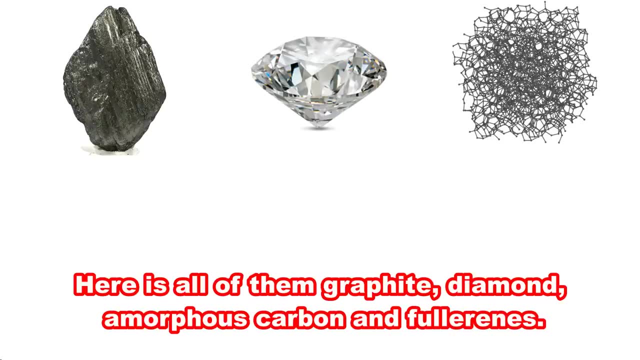 Number six: Carbon. Carbon is a non certeza metal. Carbon has many different forms. Here is all of the graphite, diamond, amorphous carbon and fullerenes. Carbon is a common element. Daddy. that's the fourth most common element you are dealing with. You know you. 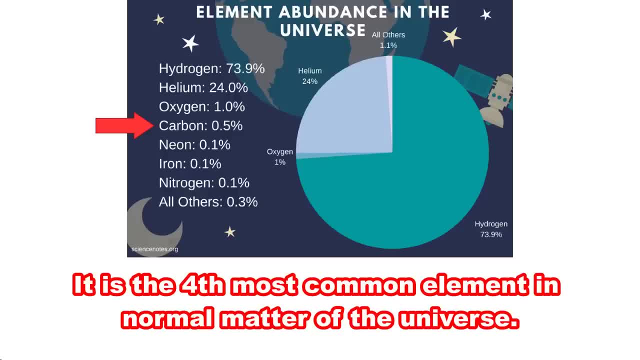 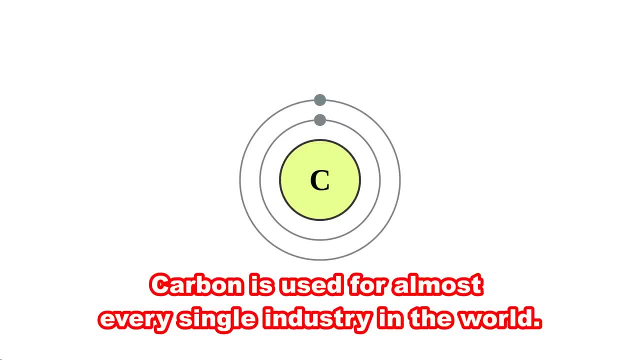 can interact with each other and you are always getting paid a billion times over That. your common element in normal matter of the universe And also second most common element in the human body, Carbon, is used for almost every single industry in the world. It is used for fuel in. 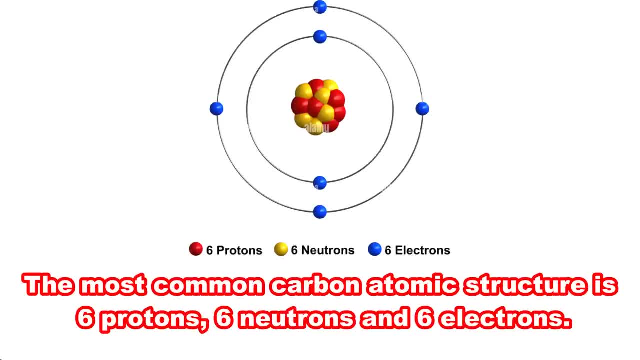 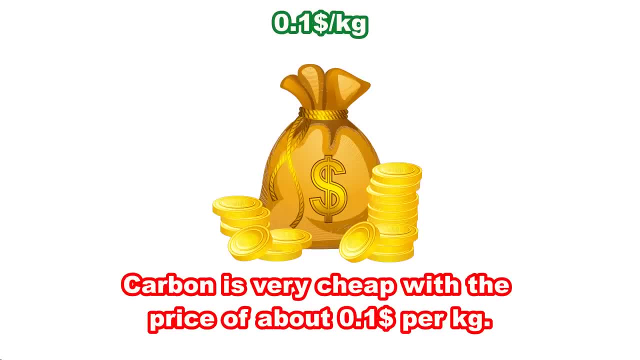 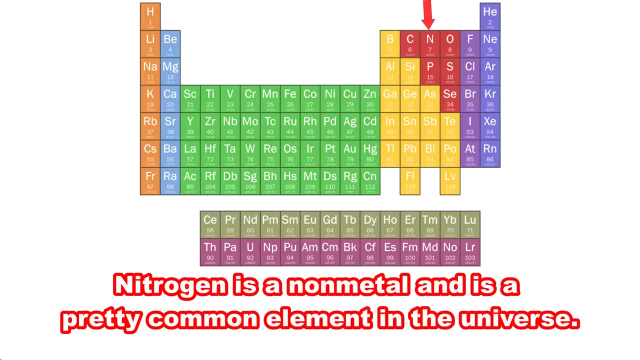 the form of coal, methane gas and crude oil. The most common carbon atomic structure is 6 protons, 6 neutrons and 6 electrons. Carbon is very cheap, with the price of about 10 cents per kilogram. Number 7. Nitrogen: Nitrogen is a non-metal and is a pretty common element in the universe. 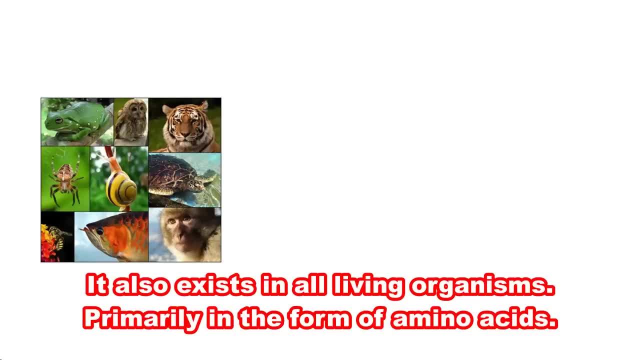 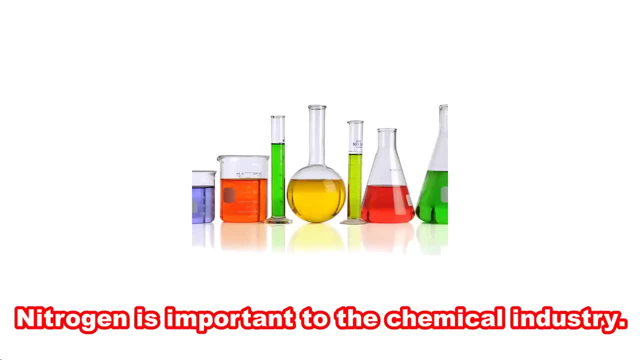 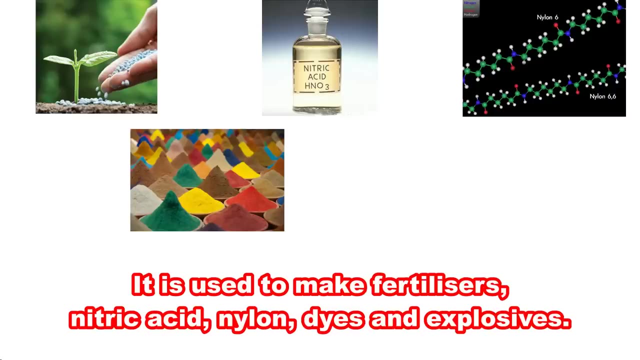 It is a colorless, odorless, diatomic gas. It also exists in all living organisms, Primarily in the form of amino acids. Nitrogen is important to the chemical industry. It is used to make fertilizers, nitric acid, nylon dyes and explosives. The most common nitrogen atomic 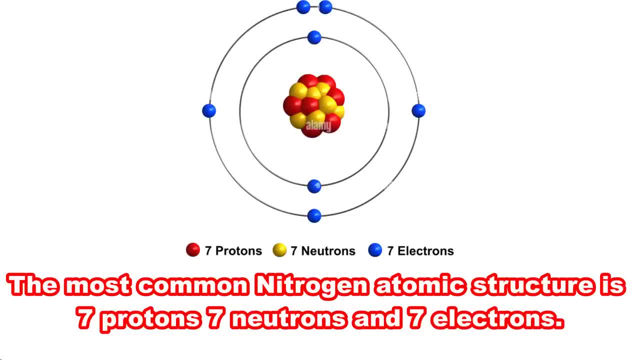 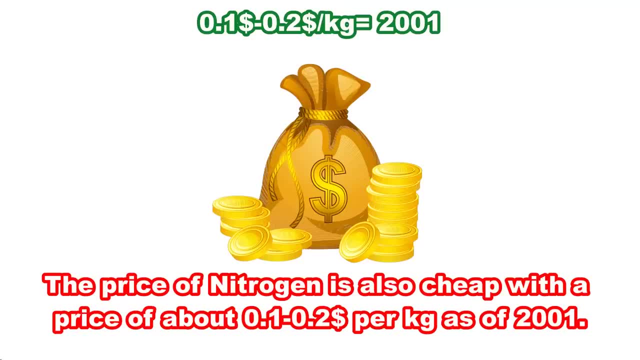 structure is 6 protons, 6 neutrons and 6 electrons. It is used for fuel in the form of 7 protons, 7 neutrons and 7 electrons. the price of nitrogen is also cheap, with a price of about 10 cents to 20 cents as of 2001.. number eight: oxygen. oxygen is a colorless, odorless gas which 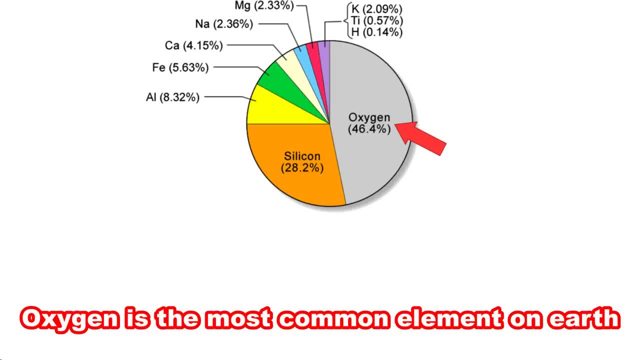 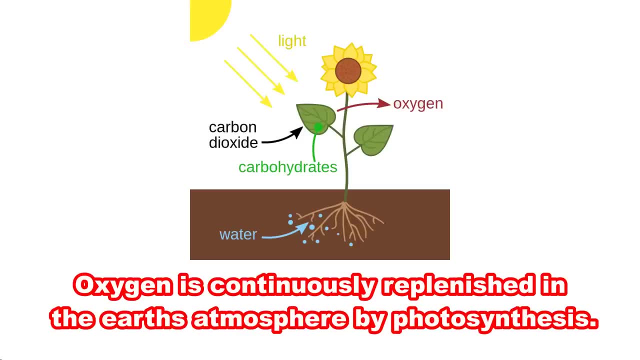 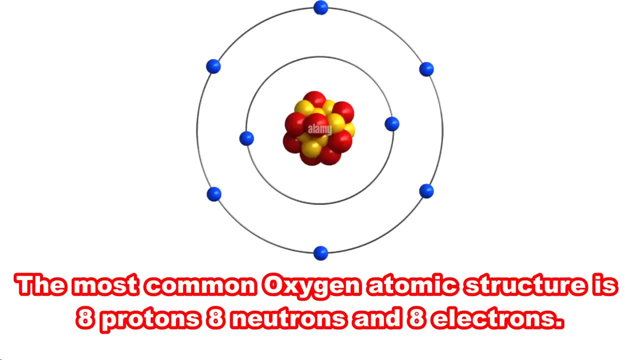 is a highly reactive non-metal. oxygen is the most common element on earth and the third most common element in the universe. oxygen is essential for all life. oxygen is continuously replenished in the earth's atmosphere by photosynthesis. the most common oxygen atomic structure is 8 protons- 8. 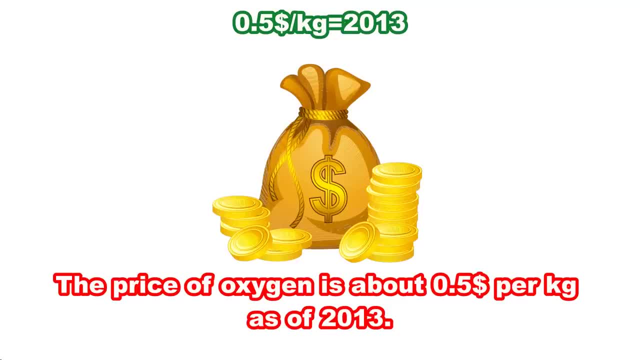 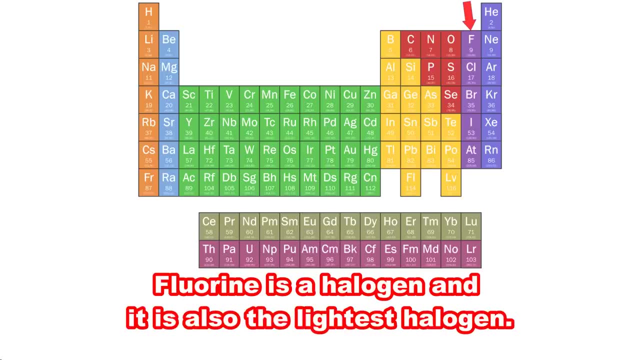 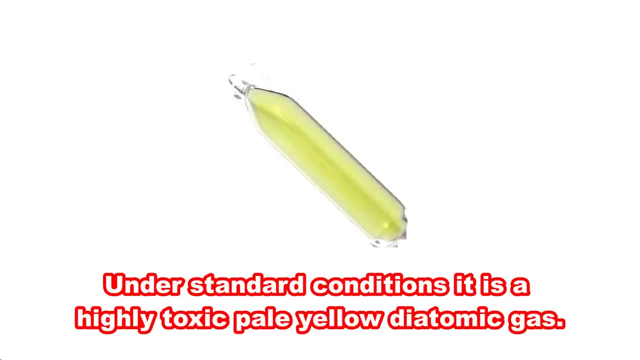 neutrons and 8 electrons. the price of oxygen is about 50 cents per kilogram as of 2013.. number 9: fluorine. fluorine is a halogen and it is also the lightest halogen. under standard conditions it is a highly toxic, pale yellow diatomic gas. it is used for nuclear power plants and for the 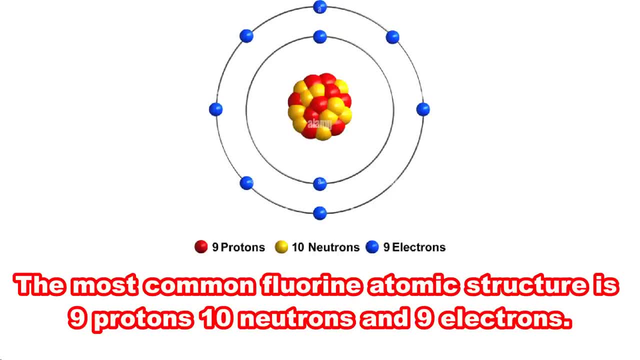 insulation of published studies. it is not likely to become alot of oxygen due to excessBUG. Independence Project's increasing demand for hydrogen Fluorine uses chlorine to irrigate biotopics and reduce electricity environment erasmus towers. the most common fluorine atomic structure is nine protons, ten neutrons. 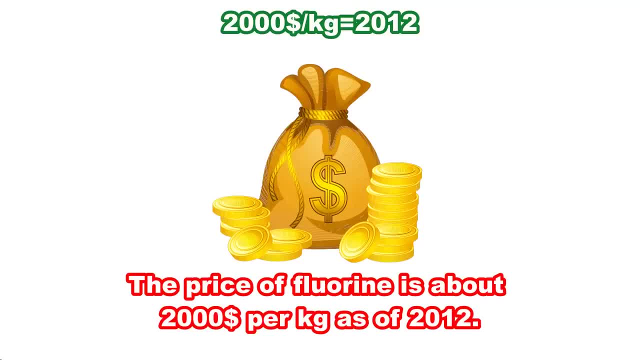 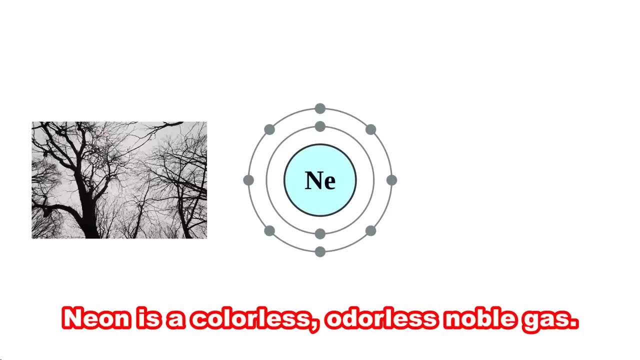 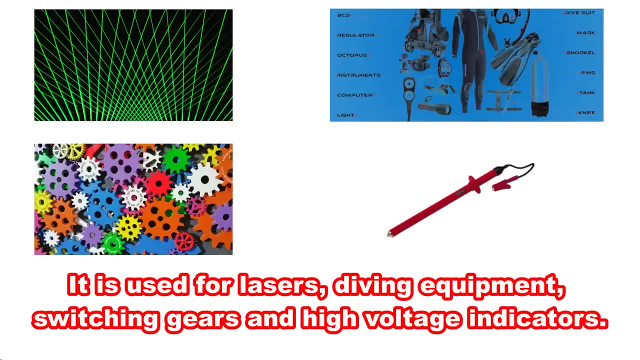 and nine electrons. the price of fluorine is about $2,000 per kilogram as of 2012. number 10: neon. neon is a colorless, odorless, noble gas. it is used for lasers, diving equipment, switching gears and high voltage indicators, the most common. 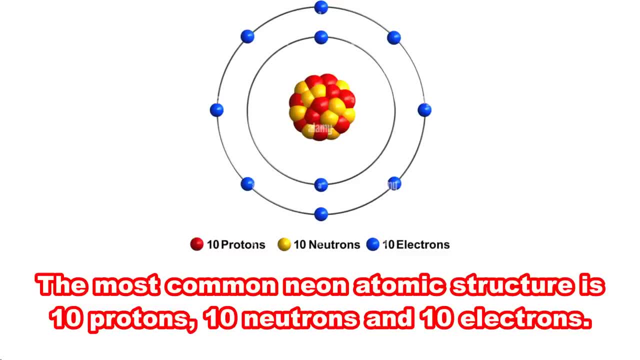 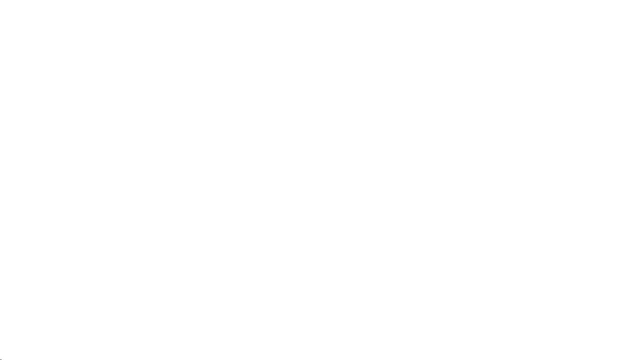 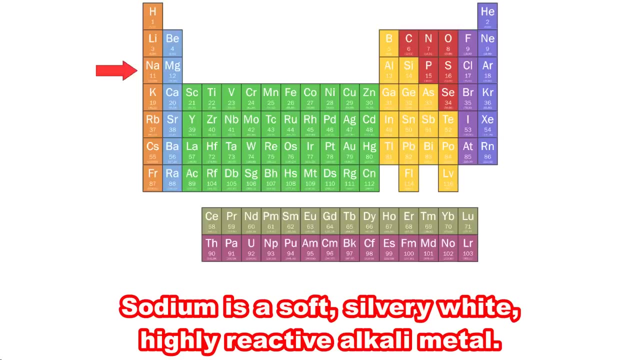 neon atomic structure is ten protons, ten neutrons and 10 electrons. the price of neon is about $630 per kilogram as of 2016. number 11: sodium: sodium is a soft silvery white, highly reactive alkali metal. sodium is also an essential 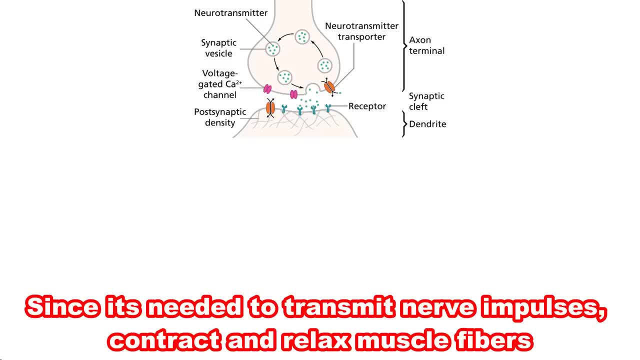 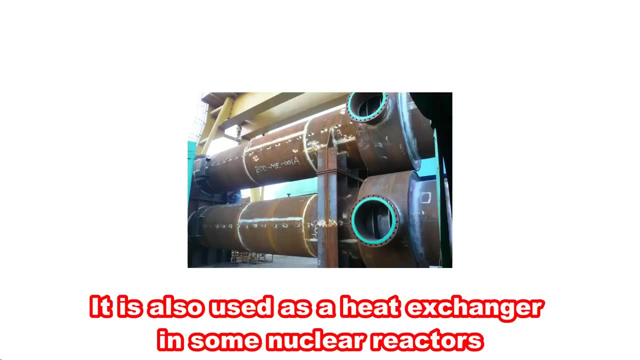 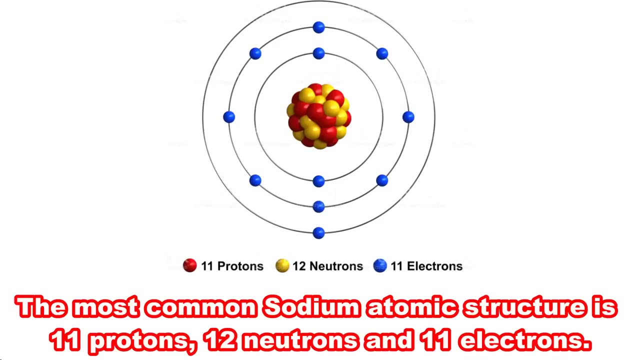 element for all life, since it's needed to transmit nerve impulses, contract and relax muscle fibers and maintain a proper balance of water and minerals. you It is also used as a heat exchanger in some nuclear reactors and as a reagent in the chemical industry. The most common sodium atomic structure is 11 protons, 12 neutrons and 11 electrons. 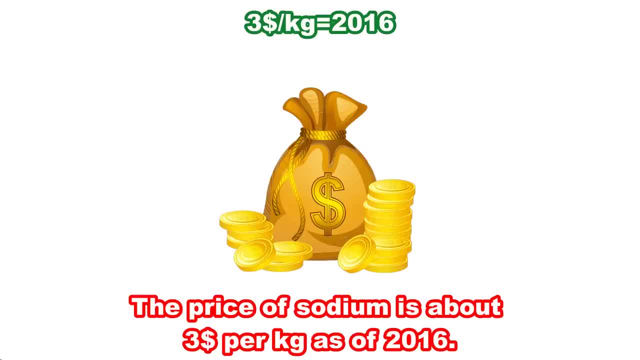 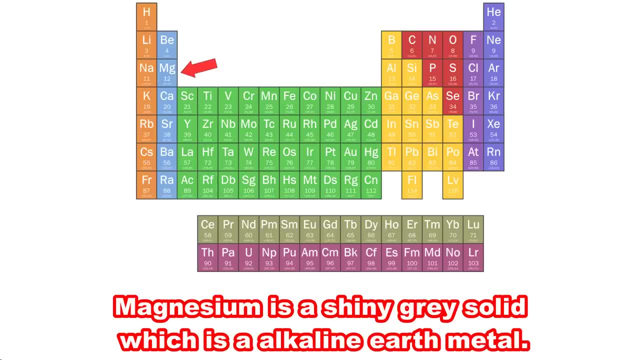 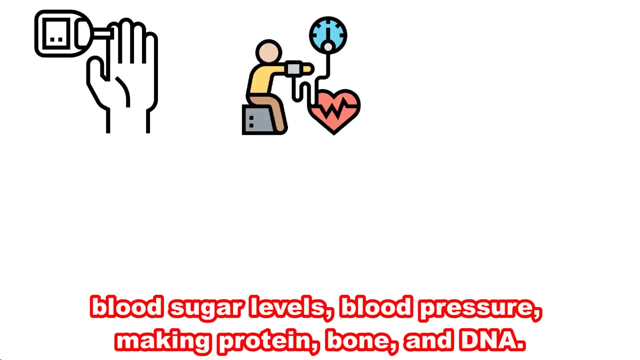 The price of sodium is about $3 as of 2016.. Number 12. Magnesium. Magnesium is a shiny gray solid which is a alkaline earth metal. Magnesium is used for regulating muscle and nerve function, blood sugar levels, blood. 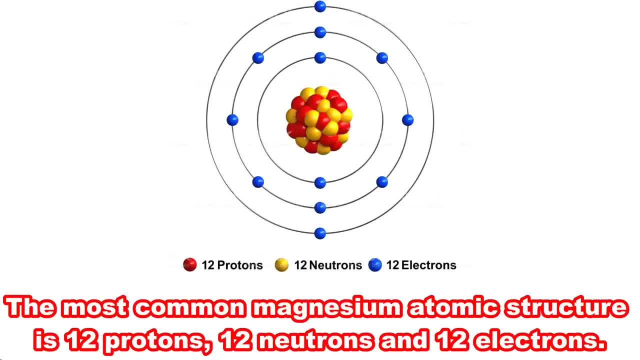 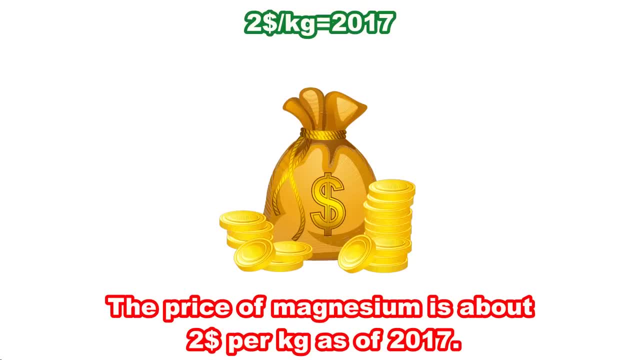 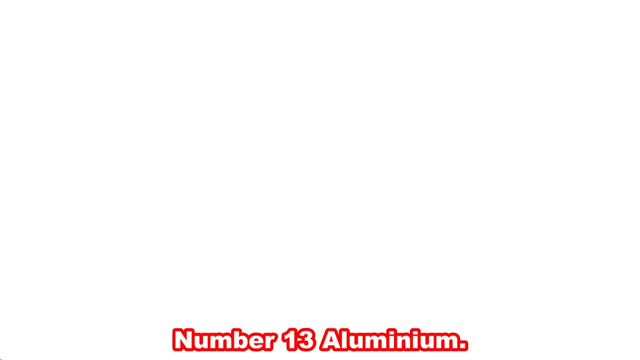 pressure making protein, bone and DNA. The most common magnesium atomic structure is 12 protons, 12 neutrons and 12 electrons. The price of magnesium is about $2 per kilogram as of 2017.. Number 13. 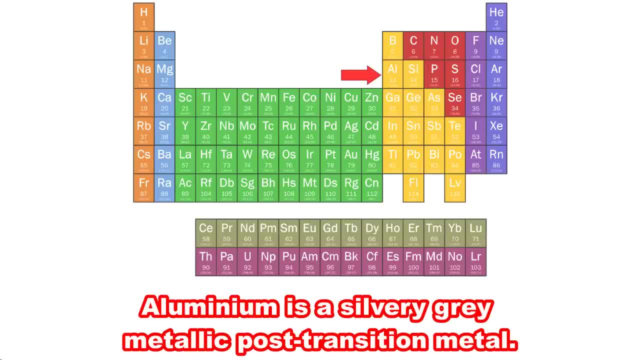 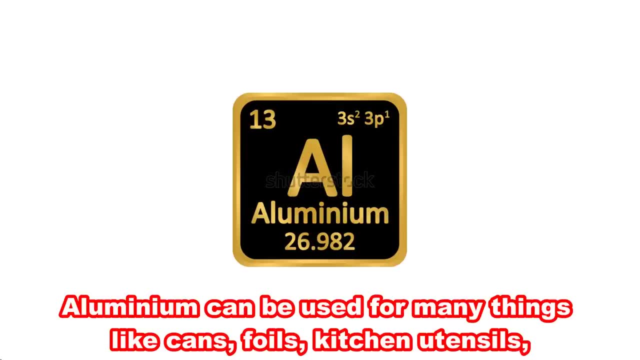 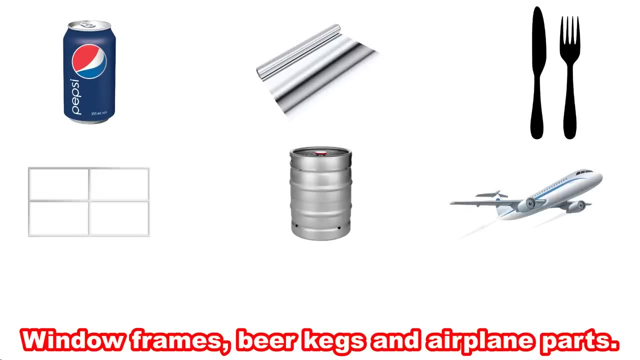 Aluminium. Aluminium is a silvery gray, metallic post-transition metal. Aluminium has a low density Compared to other metals. Aluminium can be used for many things like cans, foils, kitchen utensils, window frames, beer kegs and airplane parts. 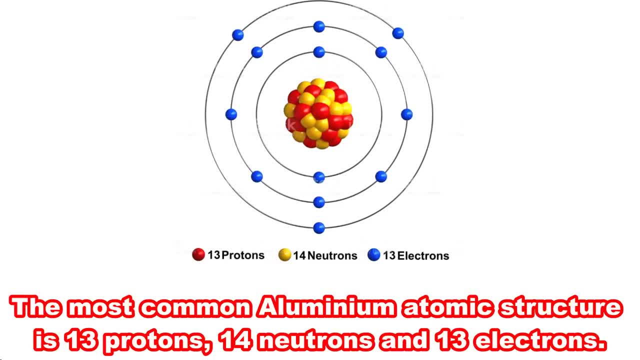 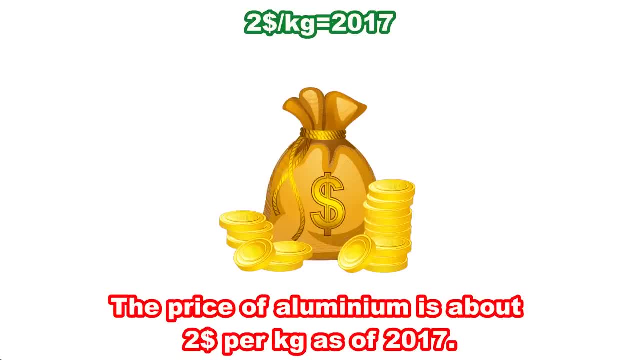 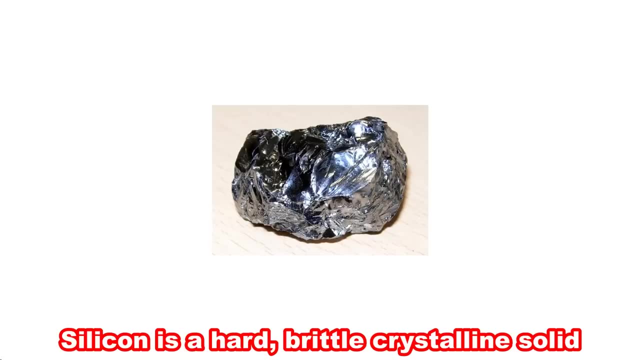 The most common aluminum atomic structure is 13 protons, 14 neutrons and 13 electrons. The price of aluminum is about $2 per kilogram as of 2017.. Number 14. Silicon. Silicon is a hard brittle crystal. 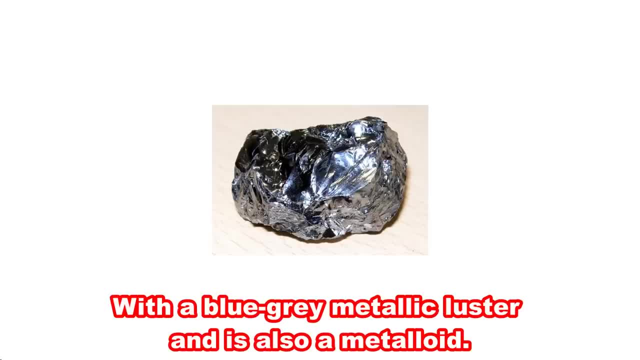 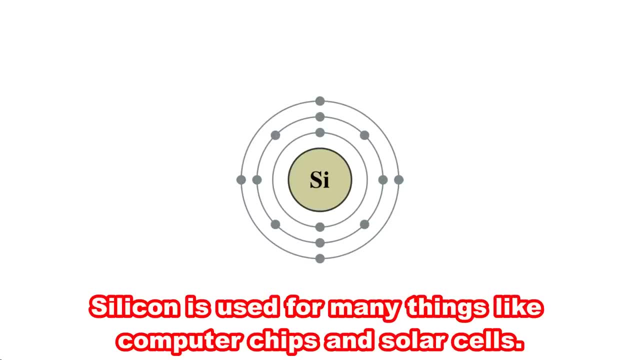 It is a hard, brittle crystal. It is a crystalline solid with a blue-gray metallic luster and is also a metalloid. It is the second most common element in the earth's crust. Silicon is used for many things, like computer chips and solar cells. 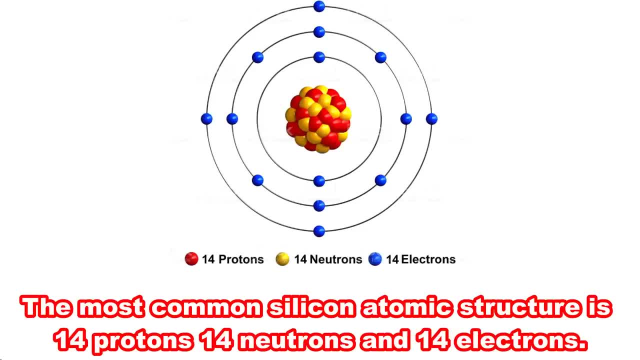 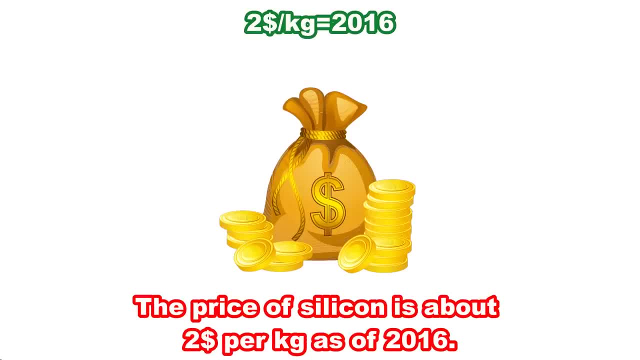 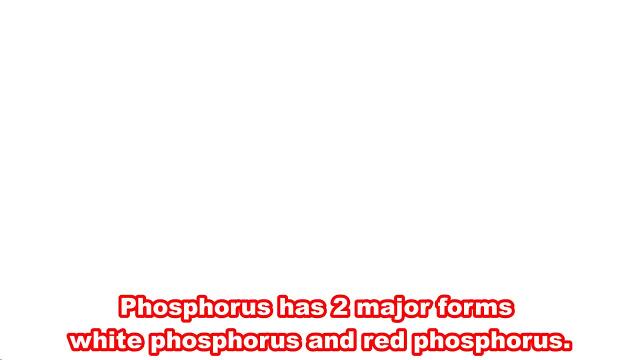 It is also a semiconductor. The most common silicon atomic structure is 14 protons, 14 neutrons and 14 electrons. The price of silicon is about $2 per kilogram as of 2016.. Number 15. Phosphorus. 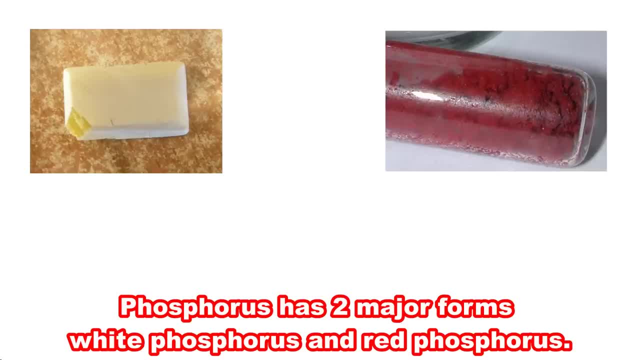 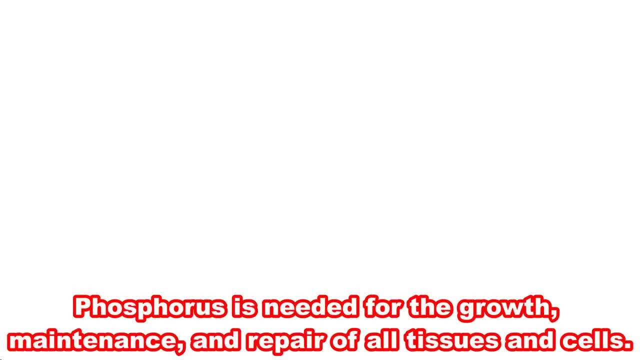 Phosphorus has two major forms: white phosphorus and red phosphorus. It is highly reactive and it is a non-metal. Phosphorus is needed for the growth, maintenance and repair of all tissues and cells and for the production of the genetic building blocks, DNA and RNA. 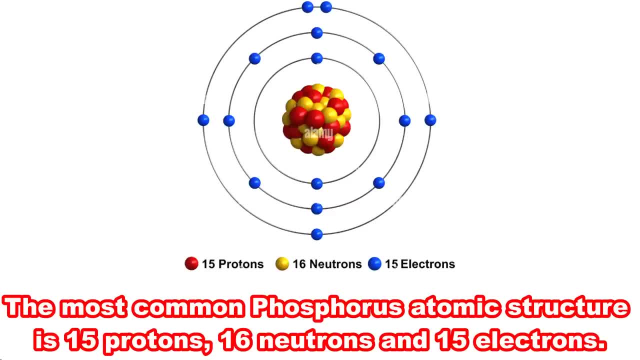 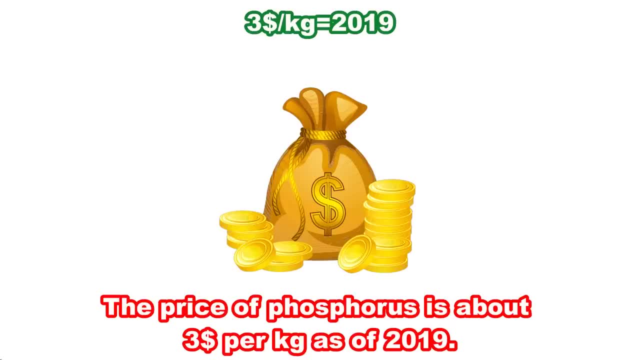 The most common phosphorus atomic structure is 15 protons, 16 neutrons and 15 electrons. The price of phosphorus is about $3 per kilogram as of 2017.. Number 16. Aluminium Silicon is used for the growth, maintenance and repair of all tissues and cells and for 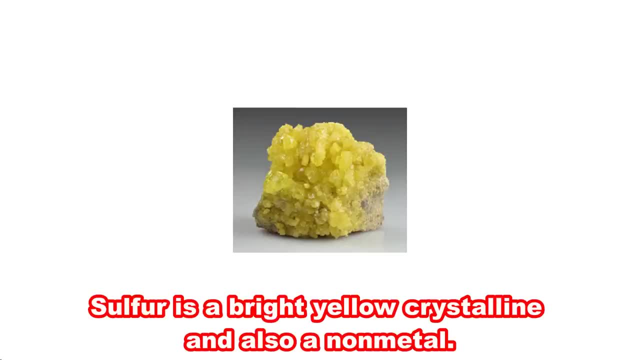 the production of the genetic building blocks, DNA and RNA. Phosphorus is needed for the growth, maintenance and repair of all tissues and cells and for the production of the genetic building blocks, DNA and RNA. The price of phosphorus is about $3 per kilogram as of 2016.. 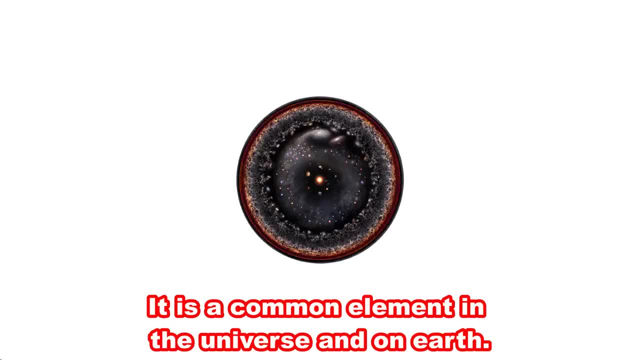 The price of silicon is about $3 per kilogram as of 2017.. Number 16. Sulfur. Sulfur is a bright yellow crystalline and also a non-metal. It is a common element in the universe and on earth. 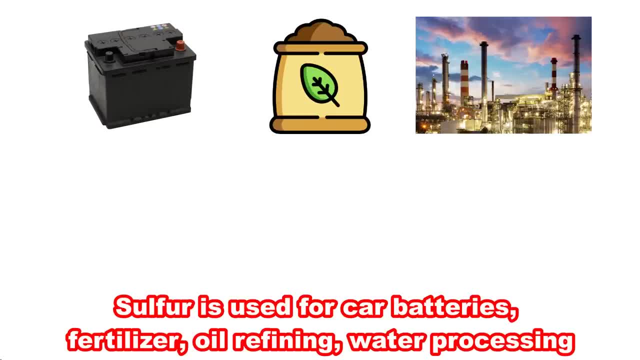 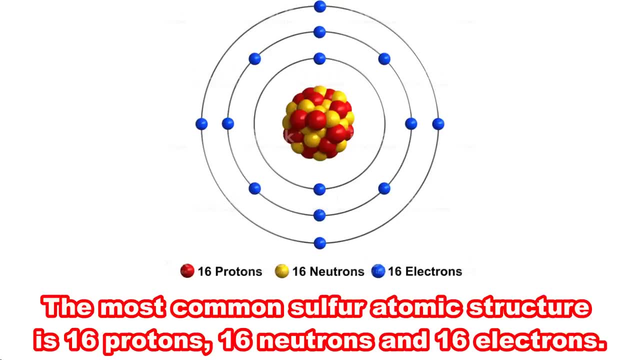 Sulfur is used for car batteries, fertilizer, oil refining, water processing and mineral extraction. The most common sulfur atomic structure is 16 protons, 16 neutrons and 16 electrons. Sulfur is very cheap, with a price of 10 cents per kilogram as of 2016.. 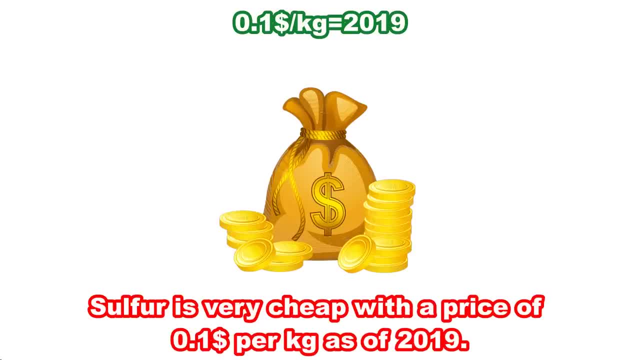 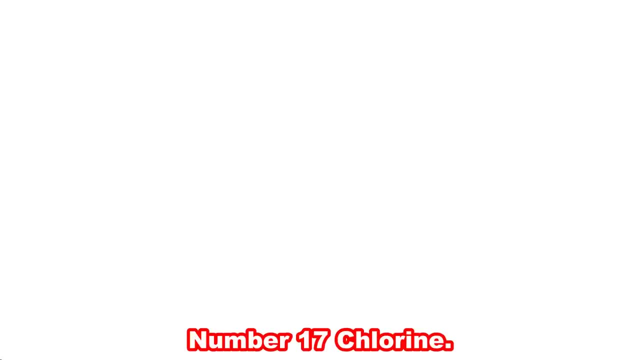 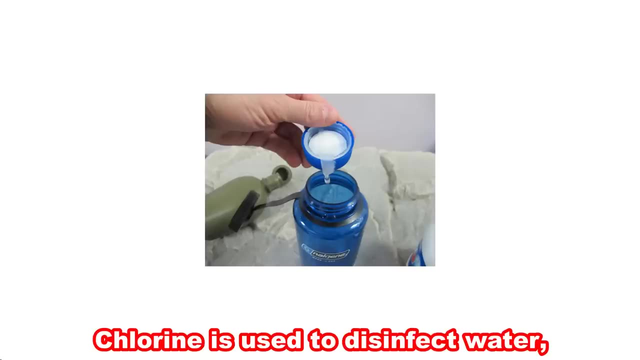 16 neutrons and 16 electrons. sulfur is very cheap, with a price of 10 cents per kilogram as of 2019. number 17: chlorine. chlorine is a light halogen. it is a pale yellow green gas. chlorine is used to disinfect water. bleach in the manufacture of paper and cloth, make pesticides, rubber and 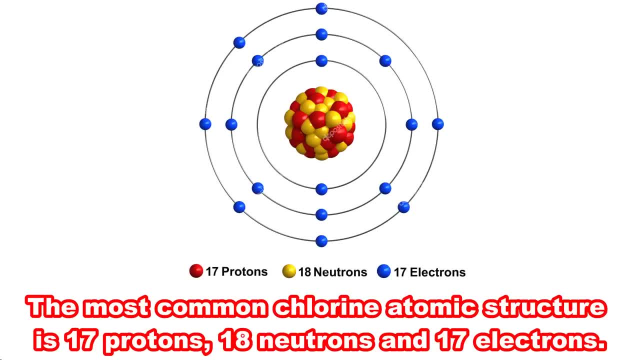 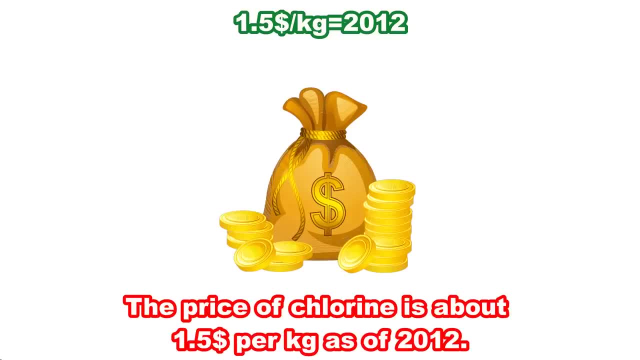 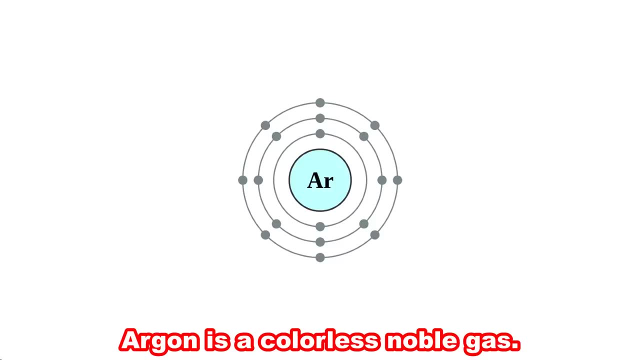 solvents. the most common chlorine atomic structure is 17 protons, 18 neutrons and 17 electrons. the price of chlorine is about 1.50 per kilogram as of 2012.. number 18, argon. argon is a colorless 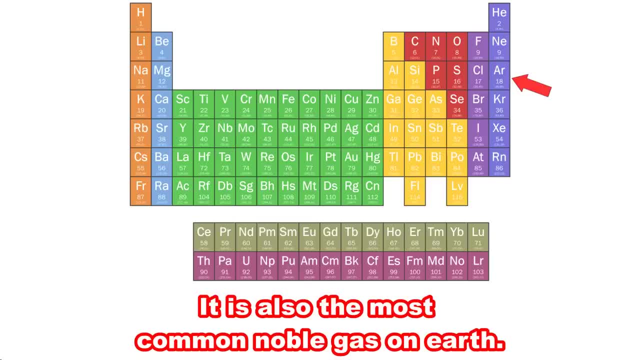 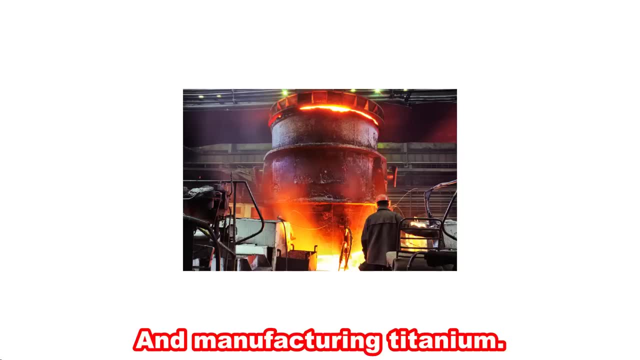 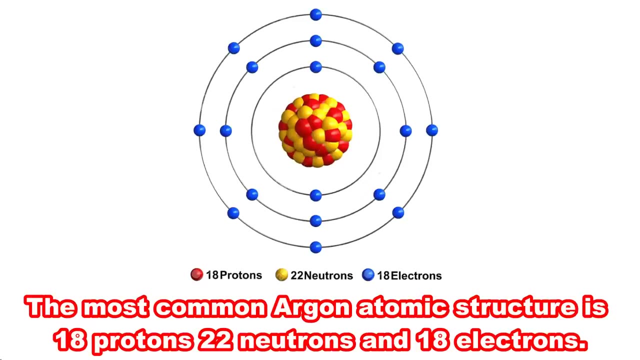 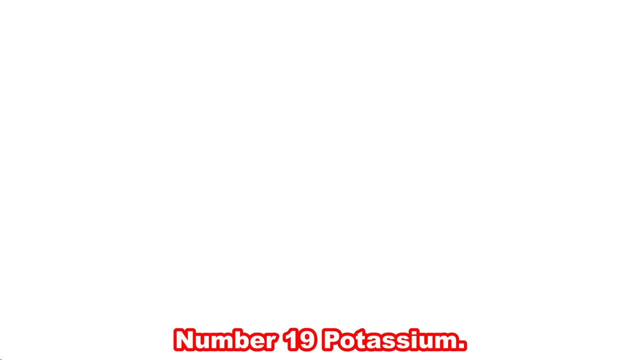 noble gas. it is also the most common noble gas on earth. argon is used for welding and casting industries, especially in the making of specialty alloys and manufacturing titanium. the most common argon atomic structure is 18 protons, 22 neutrons and 18 electrons. the price of argon is about 1 per kilogram as of 2019. number 19: potassium. 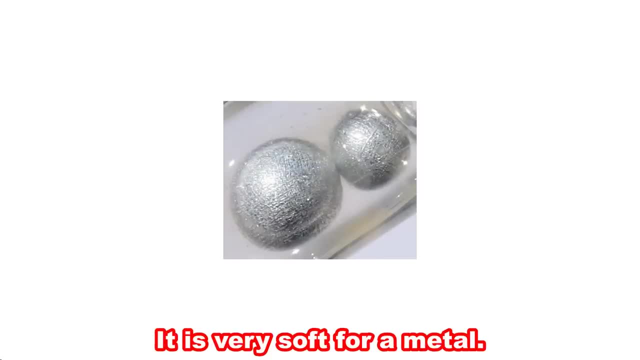 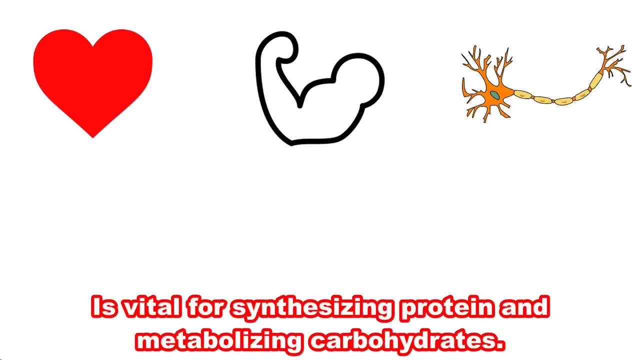 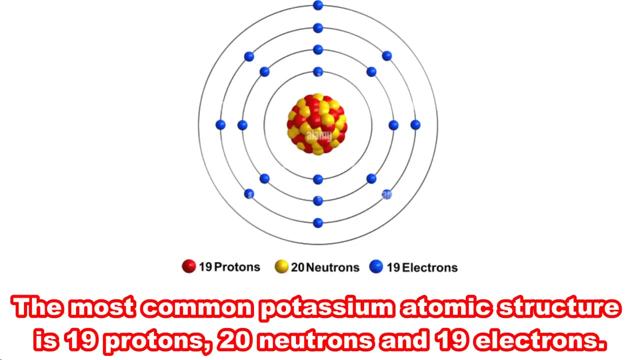 potassium is a silvery, white, alkaline metal. it is very soft for a metal. potassium regulates the heartbeat, ensures proper function of the muscles and nerves, is vital for synthesizing protein and metabolizing carbohydrates. The most common potassium atomic structure is 19 protons, 20 neutrons and 19 electrons. 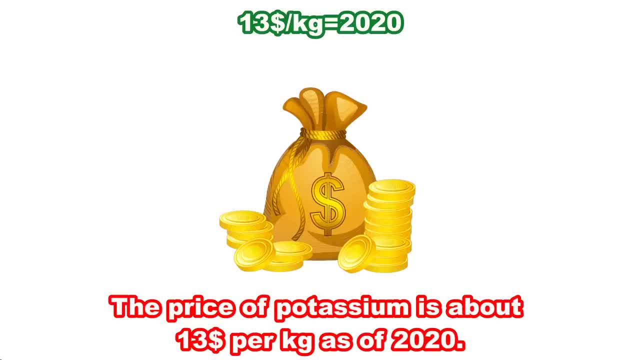 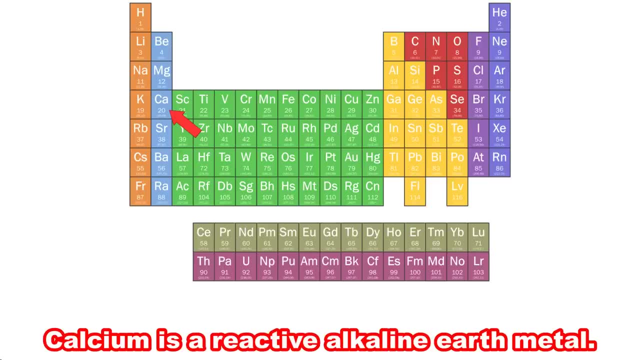 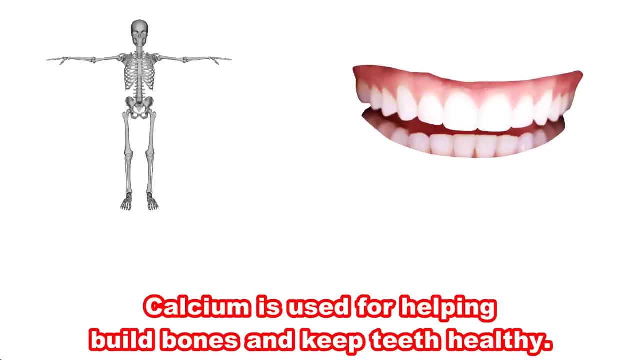 The price of potassium is about $13 per kilogram as of 2020.. Number 20. Calcium: Calcium is a reactive alkaline earth metal. It is silvery with a pale yellow tint. Calcium is used for helping build bones and keep teeth healthy. 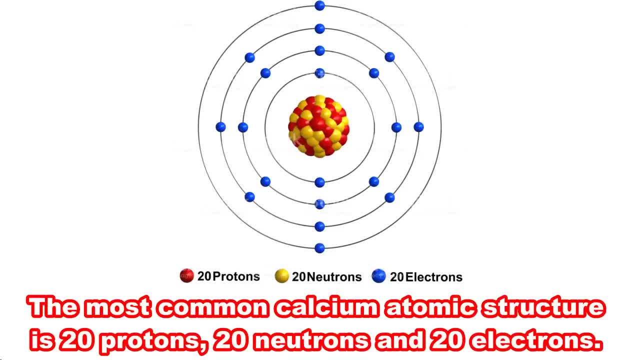 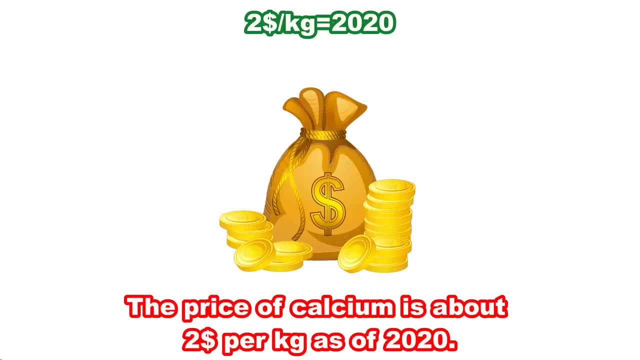 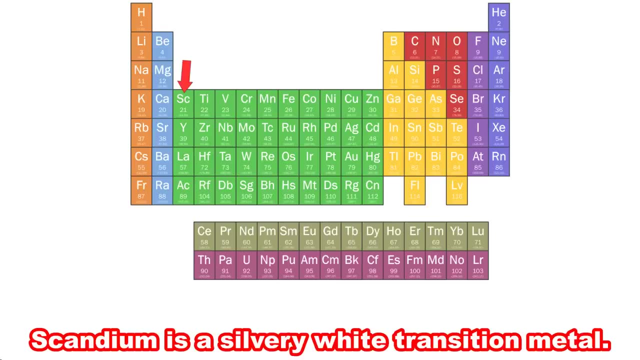 The most common calcium atomic structure is 20 protons, 20 neutrons and 20 electrons. The price of calcium is about $2 per kilogram as of 2020.. Number 21. Scandium: Scandium is a silvery white transition metal. 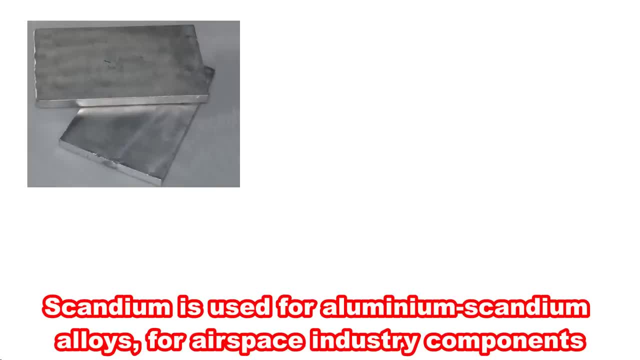 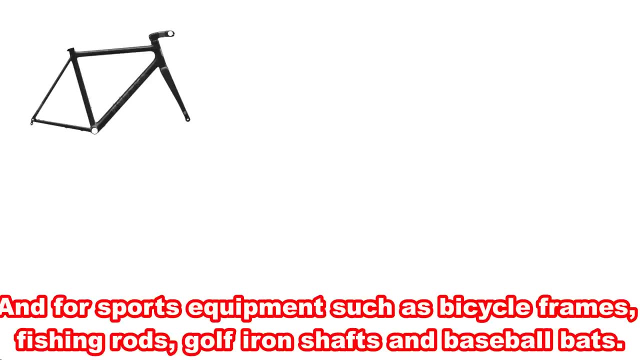 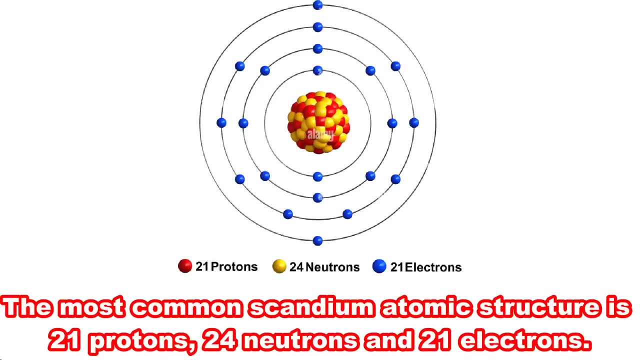 It is a pretty rare earth element. Scandium is used for aluminum, scandium alloys, for air space industry components and for sports equipment such as bicycle frames, fishing rods, etc. Golf ironshafts and baseball bats. The most common scandium atomic structure is 21 protons, 24 neutrons and 21 electrons. 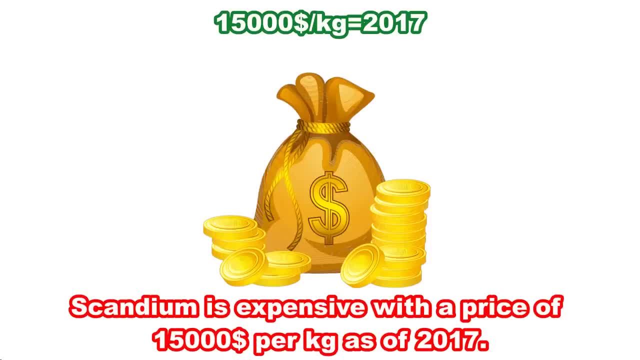 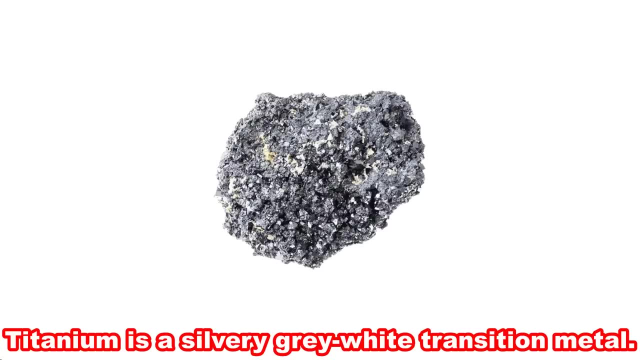 Scandium is expensive, with a price of $15,000 per kilogram as of 2017.. Number 22. Titanium: Titanium is a silvery gray, white transition metal. It is a strong metal. Titanium is used for jewelry, prosthetics, tennis rackets, goalie marks, etc. 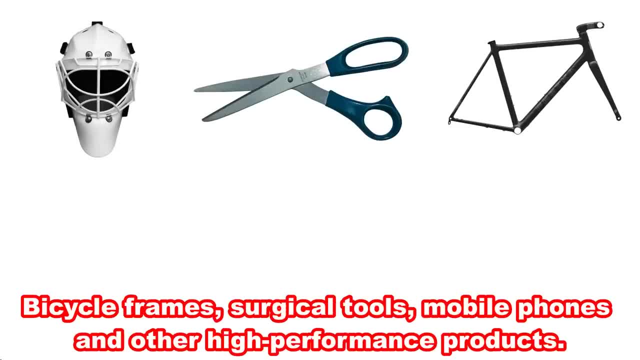 The most common titanium atomic structure is 21 protons, 24 neutrons and 21 electrons. Scandium is expensive, with a price of $15,000 per kilogram as of 2017.. Scandium is used for jewelry, masks, scissors, bicycle frames, surgical tools, mobile phones. 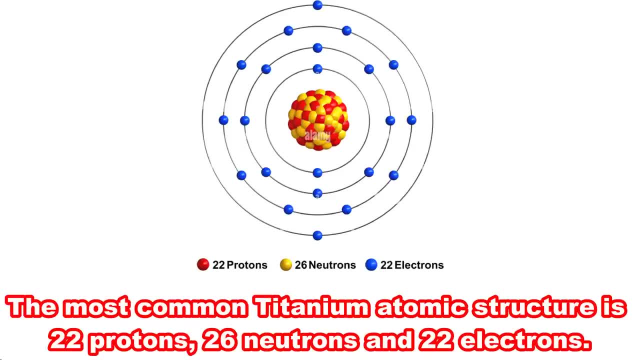 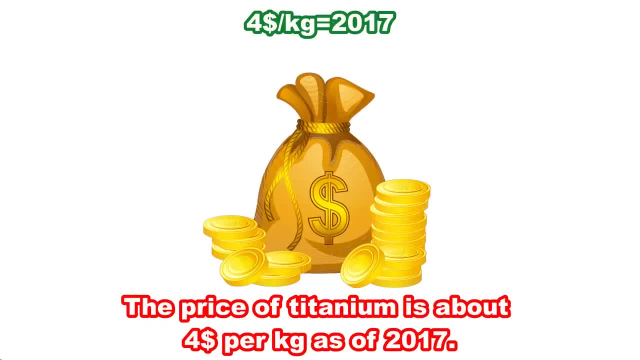 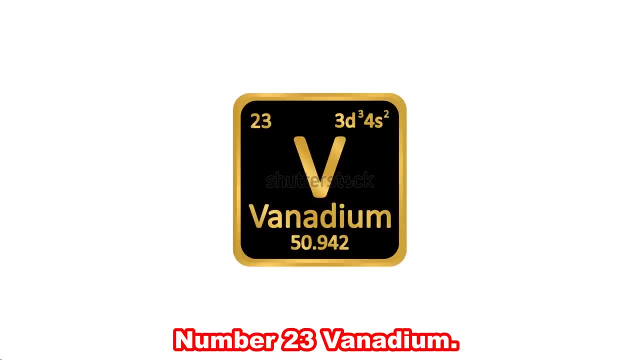 and other high-performance products. The most common titanium atomic structure is 22 protons, 26 neutrons and 22 electrons. The price of titanium is about $4 per kilogram as of 2017.. Number 23. Vanadium. 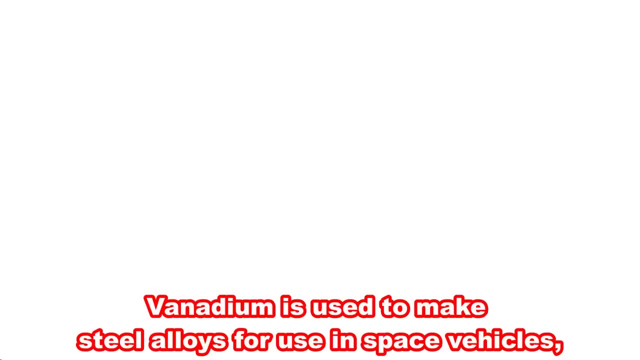 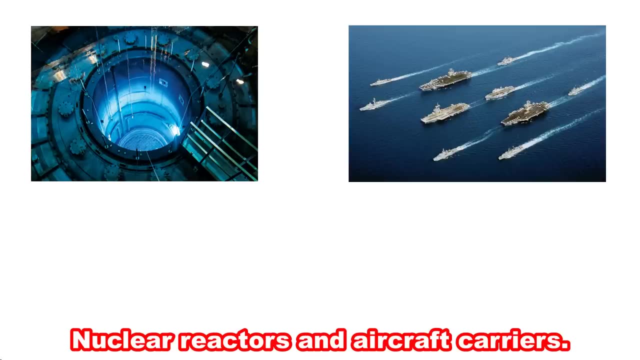 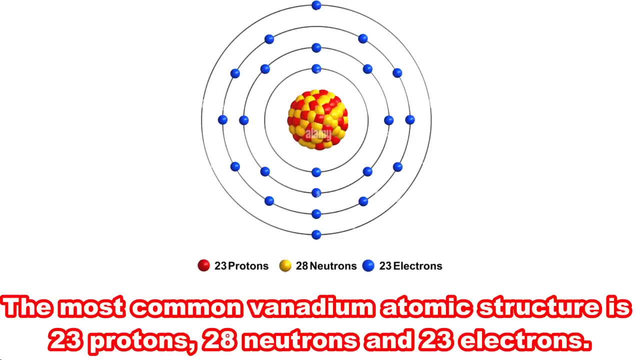 Vanadium is a hard, silvery- gray transition metal. Vanadium is used to make steel. Vanadium is used to make steel alloys for use in space vehicles, nuclear reactors and aircraft carriers. The most common vanadium atomic structure is 23 protons, 28 neutrons and 23 electrons. 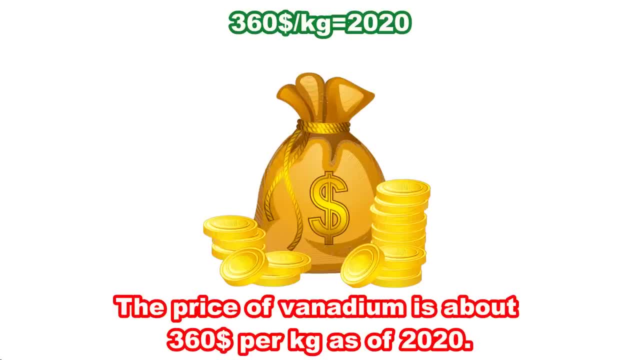 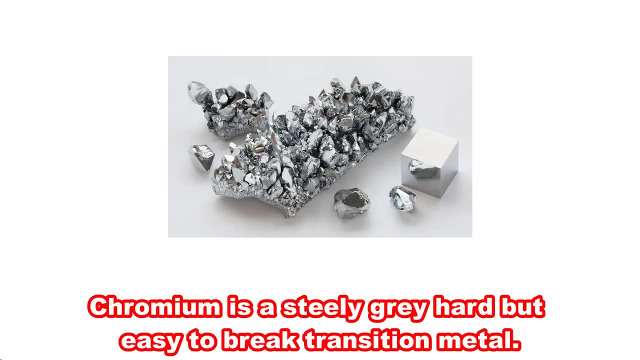 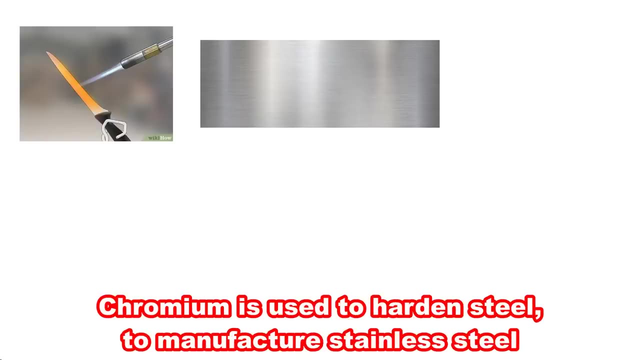 The price of vanadium is about $360 per kilogram as of 2020.. Number 24. Chromium: Chromium is a steely gray, hard but easy to break. transition metal. Vanadium is used to harden steel, to manufacture stainless steel and to produce several alloys. 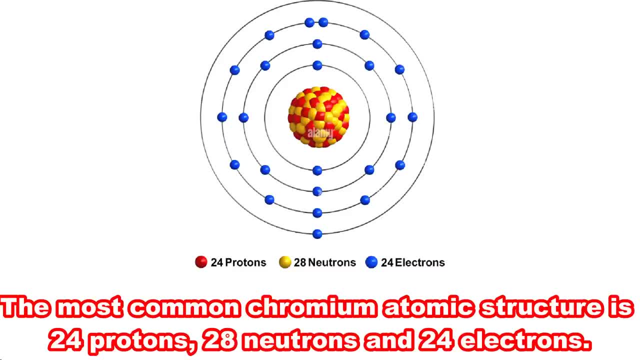 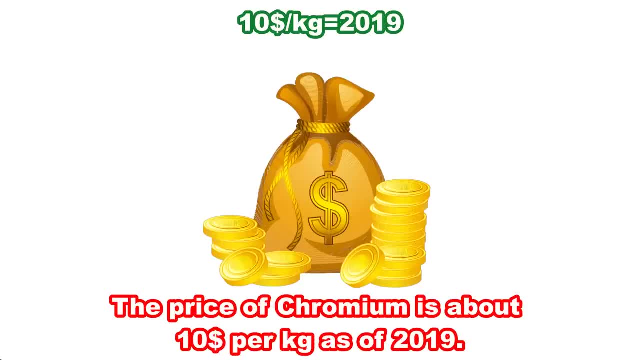 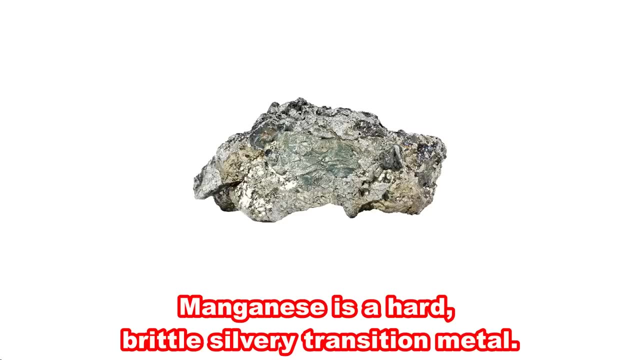 The most common chromium atomic structure is 24 protons, 28 neutrons and 24 electrons. The price of chromium is about $10 per kilogram as of 2019.. Number 25. Manganese. Manganese is a hard, brittle, silvery transition metal. 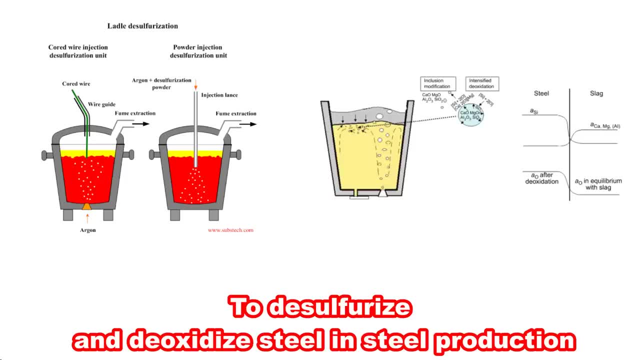 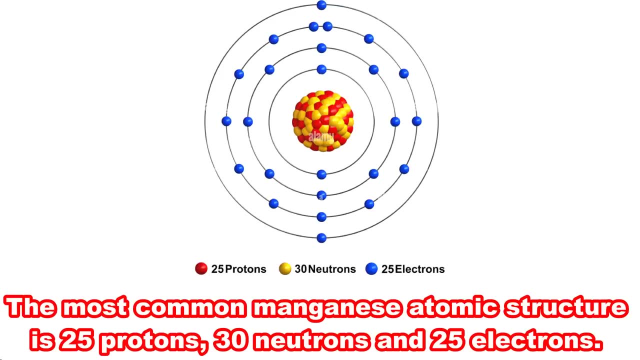 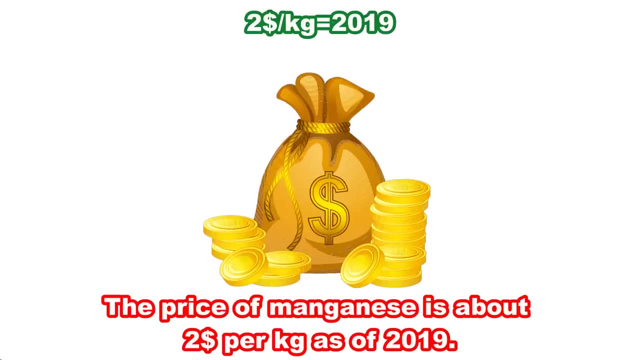 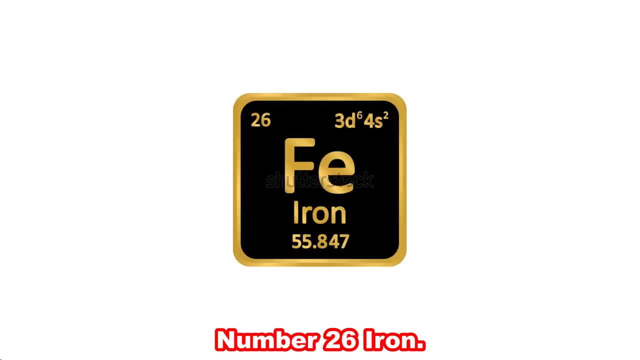 Manganese is used to make clear glass, to de-sulfurize and to make glass. The most common chromium atomic structure is 24 protons, 28 neutrons and 24 electrons. The price of manganese is about $. Vanadium is used to recommend marine gas products, which Xiao. 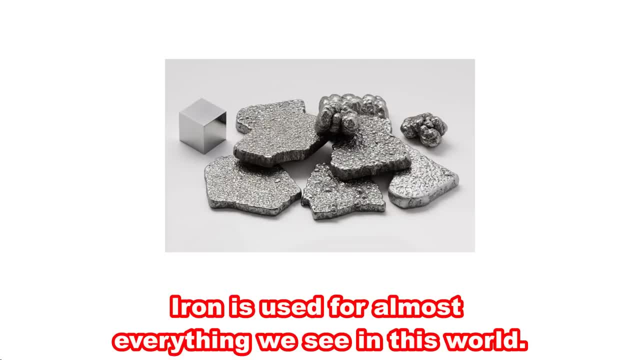 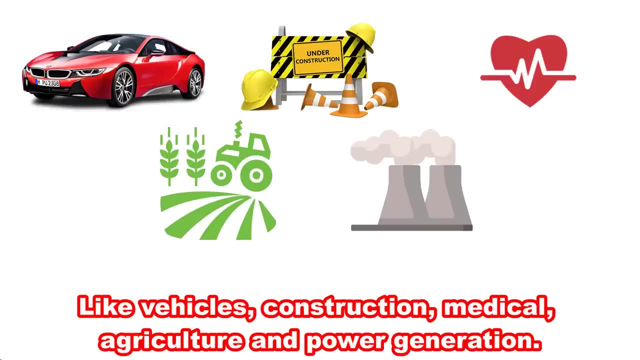 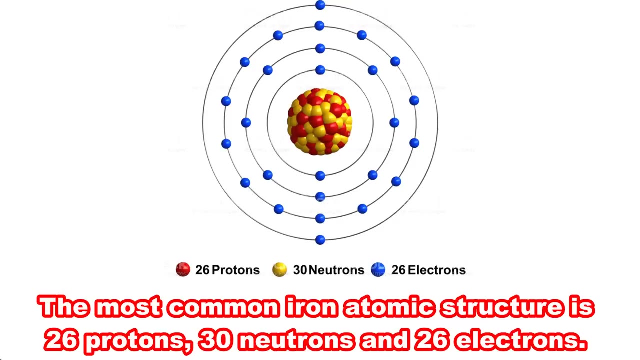 steel companies. name Cante all each other. Iron is used for almost everything we see in this world, Like vehicles, construction, medical, agriculture and power generation. Iron is also used to make steel. The most common iron atomic structure is 26 protons, 30 neutrons and 26 electrons. 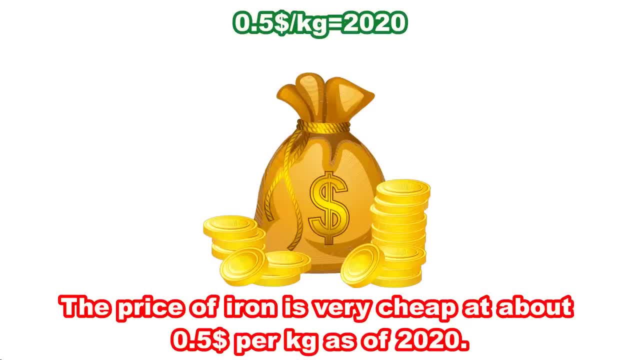 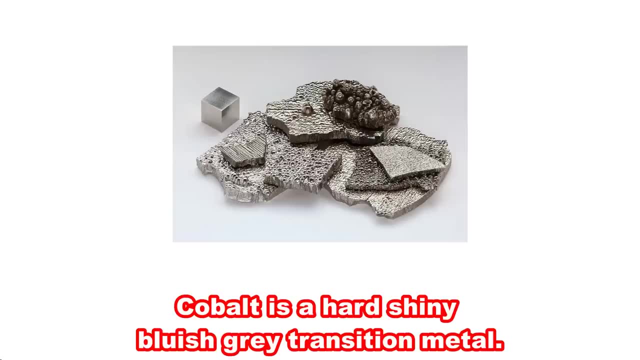 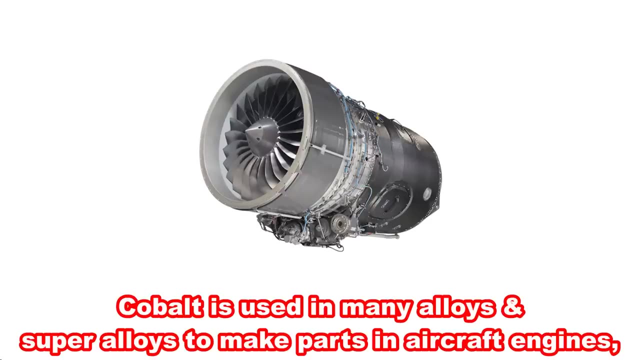 The price of iron is very cheap, at about 50 cents per kilogram as of 2020.. Number 27. Cobalt: Cobalt is a hard, shiny, bluish, gray transition metal. Cobalt is used in many alloys and super alloys to make parts in aircraft engines, gas turbines. 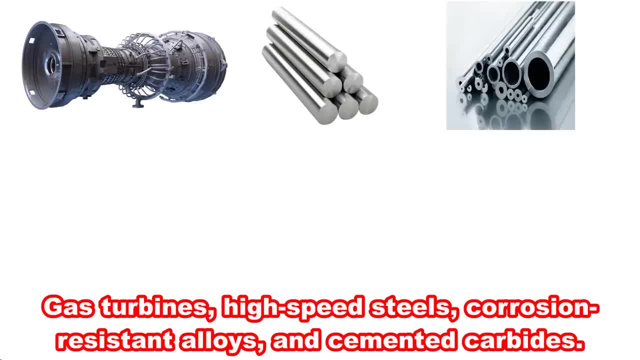 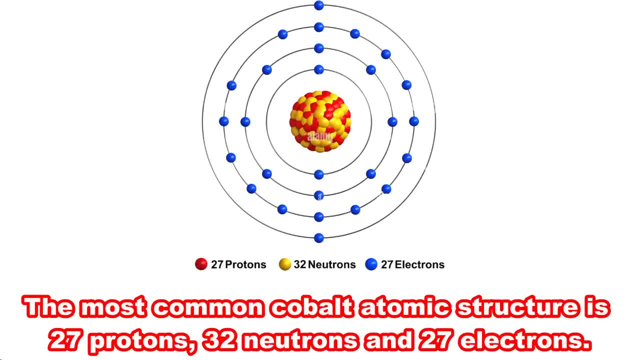 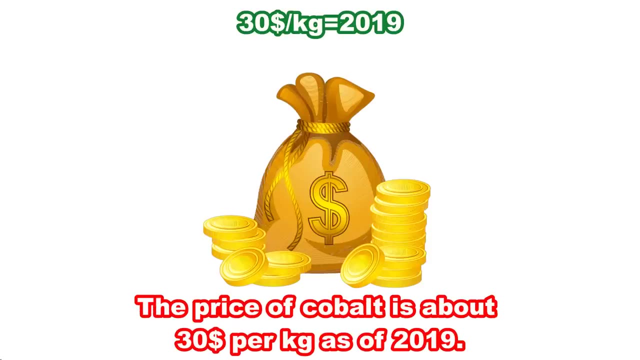 high speed steels, corrosion resistant alloys and cemented carbides. The most common cobalt atomic structure is 27 protons, 32 neutrons and 27 electrons. The price of cobalt is about 30 dollars per kilogram as of 2019.. 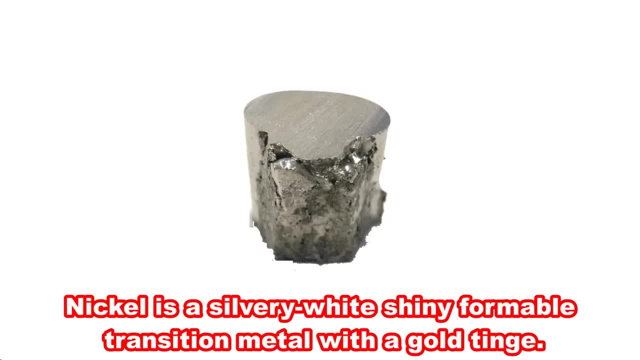 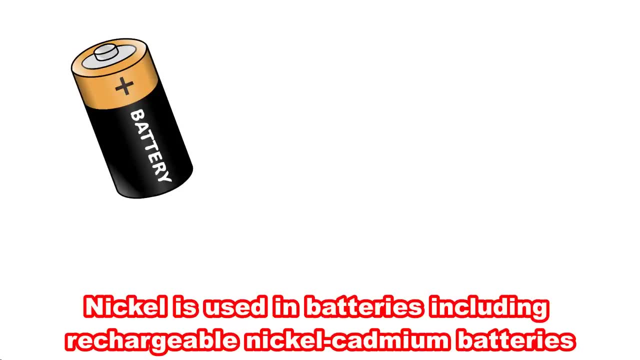 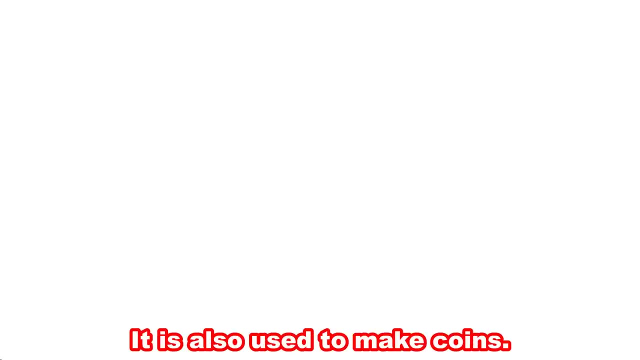 Number 28. Nickel: Nickel is a silvery, white, shiny formable transition metal with a gold tinge. Nickel is used in batteries, including rechargeable nickel cadmium batteries and nickel metal hydride batteries used in hybrid vehicles. It is also used to make coins. 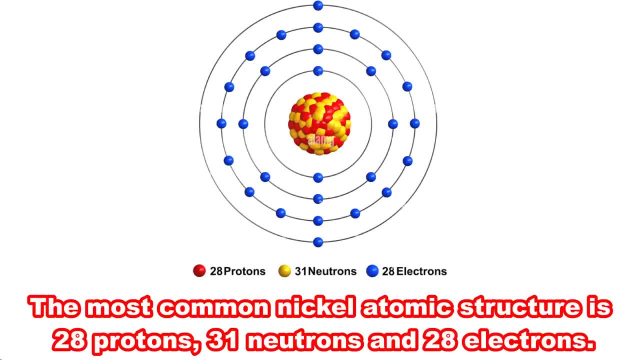 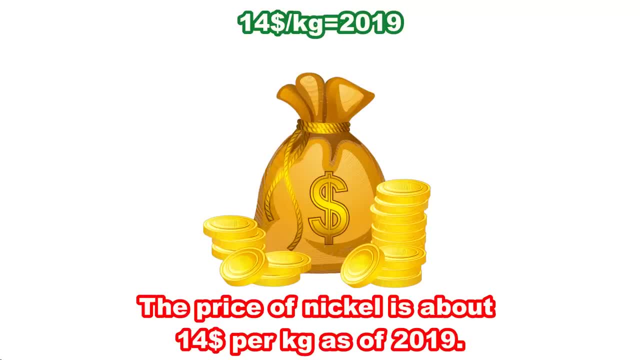 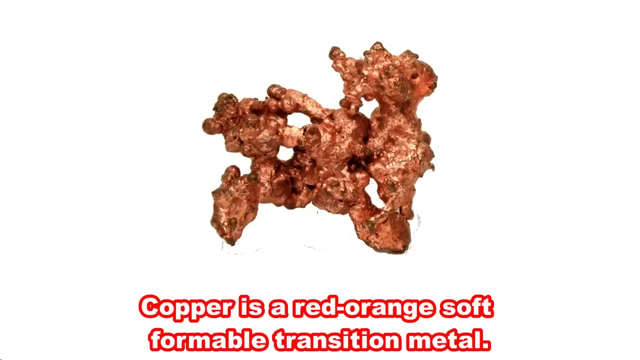 The most common nickel atomic structure is 28 protons, 31 neutrons and 28 electrons. The price of nickel is about 14 dollars per kilogram as of 2019.. Number 28. Copper: copper is a red orange, soft formable transition metal. 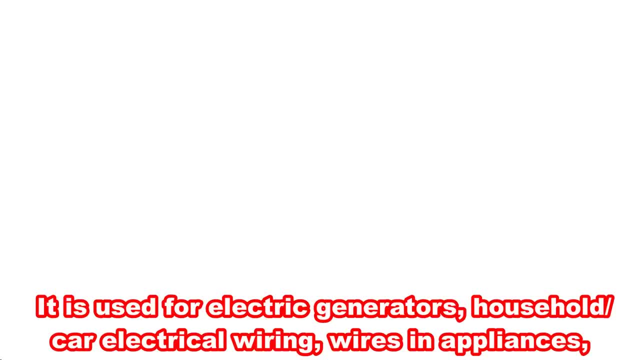 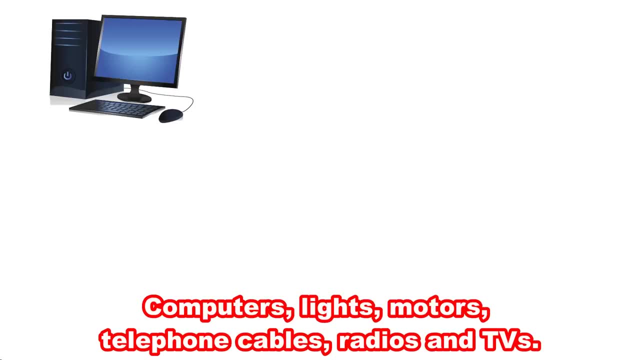 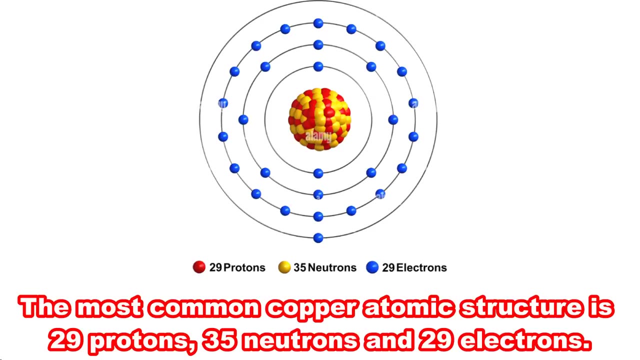 Copper is one of the best conductors. It is used for electric generators, household slash, car electrical wiring, wires in appliances, computers, lights, motors, telephone cables, radios and TVs. The most common copper atomic structure is 29 protons, 35 neutrons and 29 electrons. 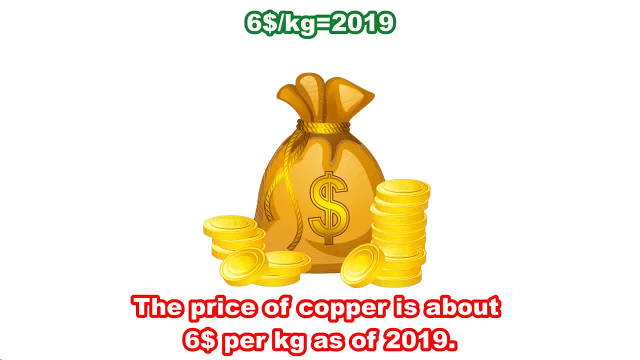 The most common copper atomic structure is 26 protons, 32 neutrons and 29 electrons. The most common copper atomic structure is about 25 protons, 32 neutrons and 27 electrons- electrons. the price of copper is about six dollars per kilogram as of 2019. 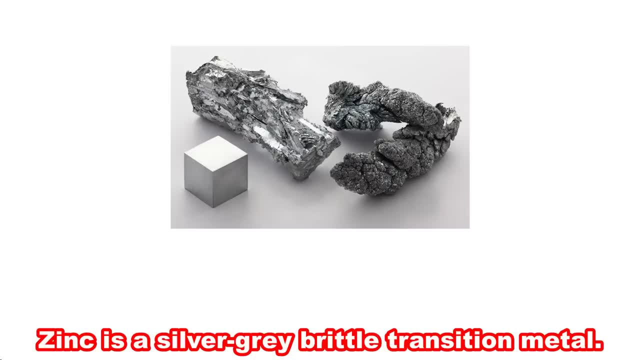 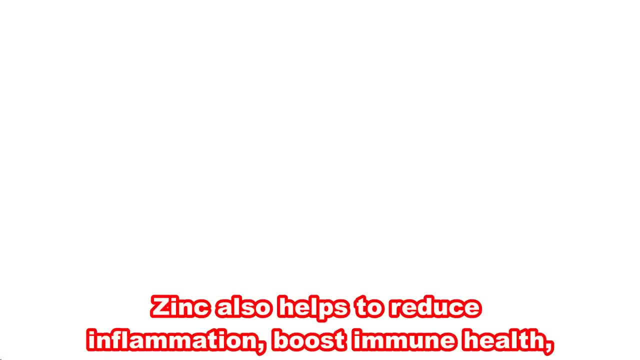 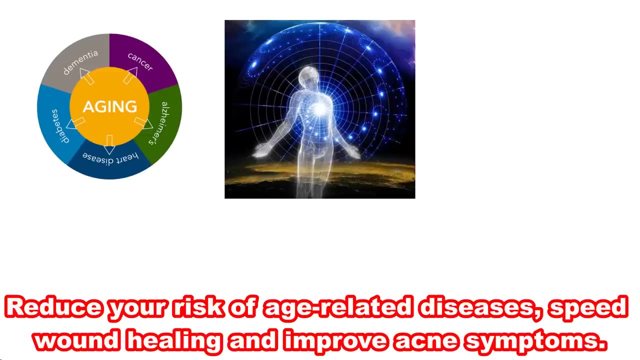 number 30, zinc. zinc is a silvery, gray, brittle transition metal. zinc is used to prevent other metals from rusting. zinc also helps to reduce inflammation, boost immune health, reduce your risk of age-related diseases, speed wound healing and improve acne symptoms. the most common zinc atomic structure is 30. 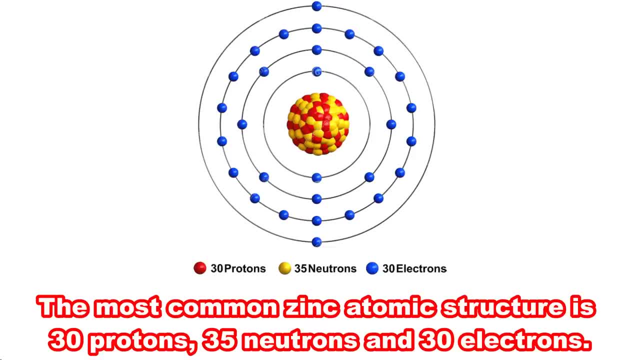 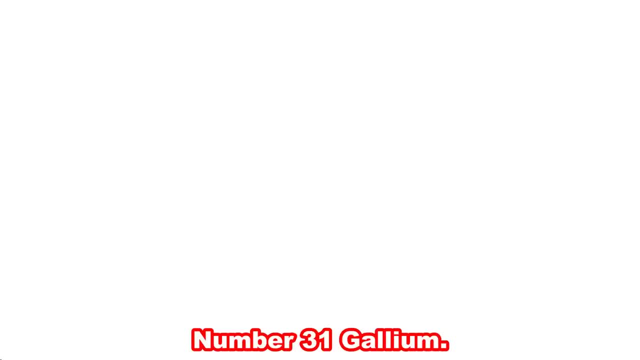 protons, 35 neutrons and 30 electrons. the price of zinc is about 2 dollars and 50 cents per kilogram as of 2019. number 31: gallium. gallium is a soft, silvery blue post transition metal. gallium is used for electronic circuits. 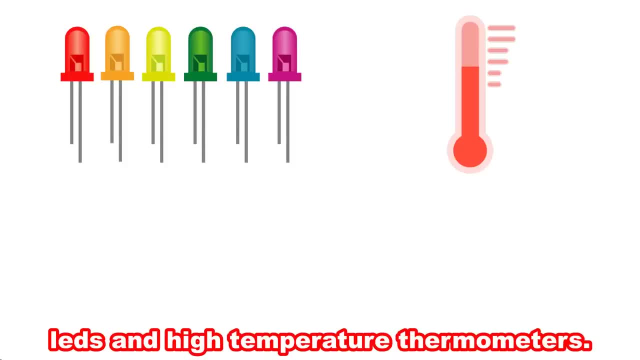 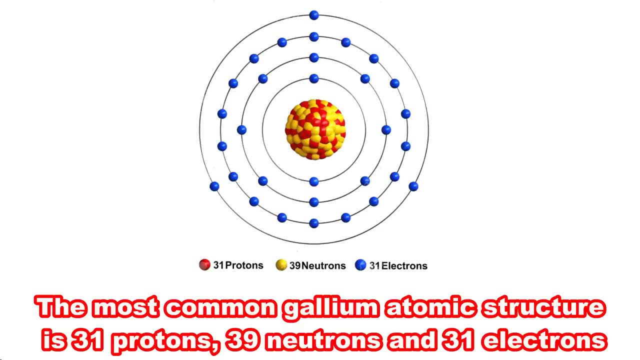 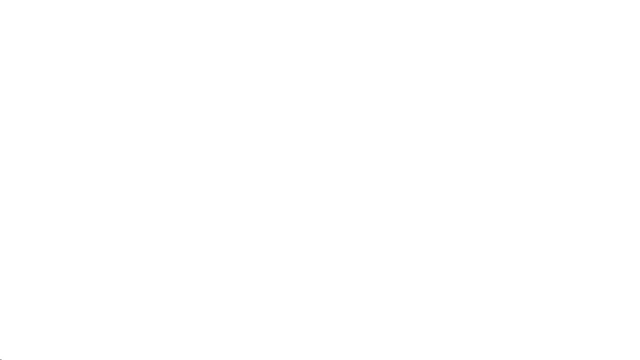 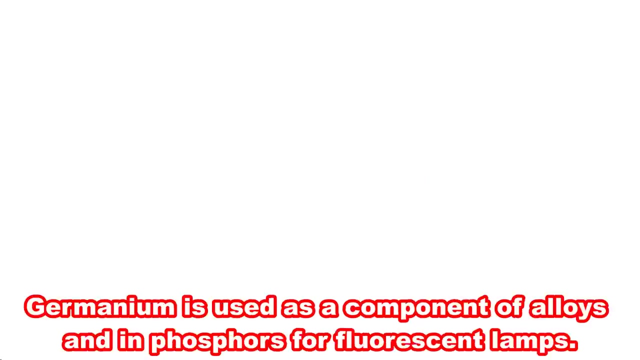 semiconductors, LEDs and high temperature thermometers. the most common gallium atomic structure is 31 protons, 39 neutrons and 31 neutrons electrons. the price of gallium is about 150 dollars per kilogram as of 2019. number 32: germanium. germanium is a shiny, brittle, grayish, white metalloid. germanium. 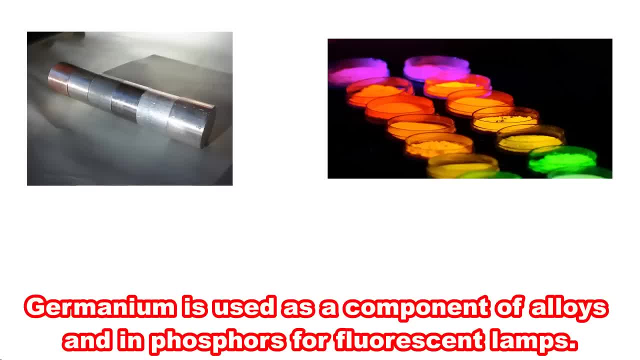 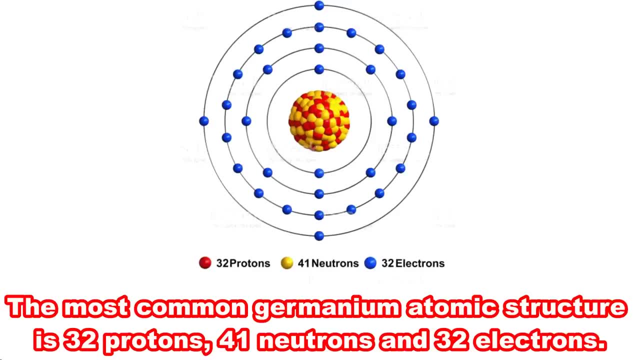 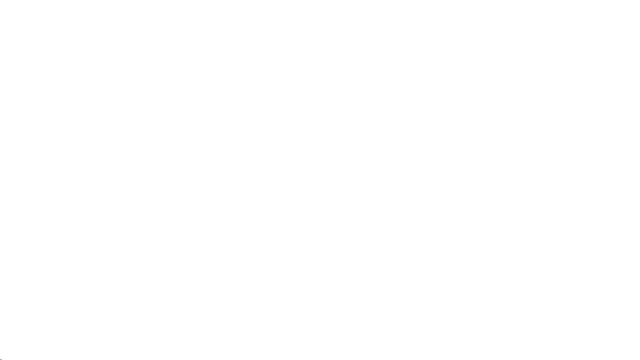 is used as a component of alloys and in phosphors for fluorescent lamps. the most common germanium atomic structure is 32 protons, 41 neutrons and 32 electrons. the price of germanium is about 1,000 dollars per kilogram as of 2020 number. 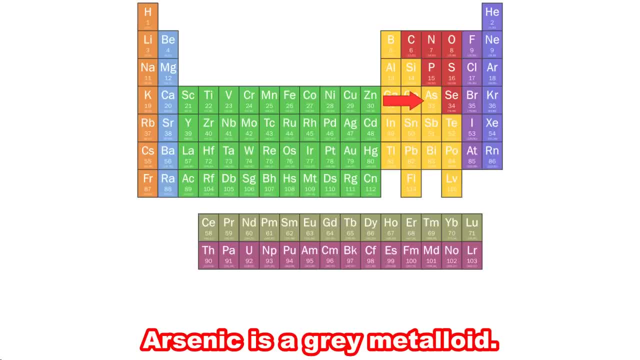 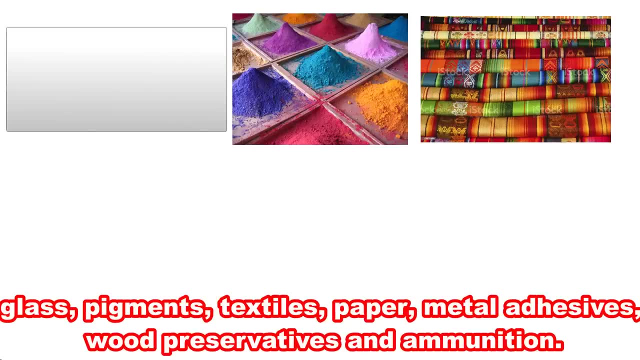 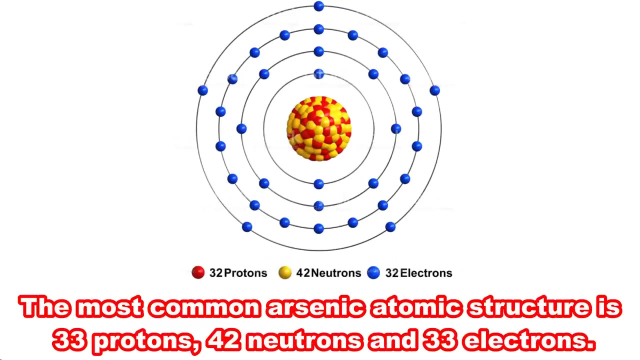 33 arsenic. arsenic is a gray metalloid. arsenic is used for alloying agent as well as in the processing of glass, pigments, textiles, paper, metal adhesives, wood preservatives and ammunition. the most common atomic structure is 33 protons, 42 neutrons and 33 electrons. the price of arsenic is about. 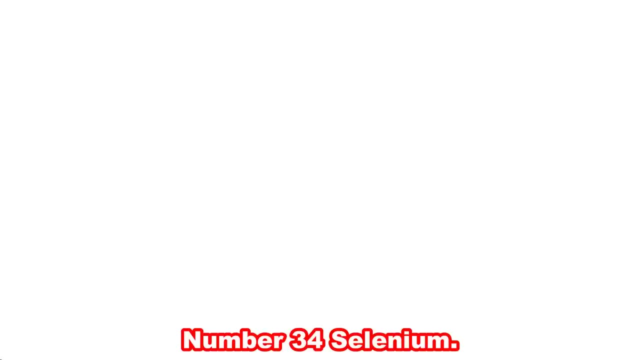 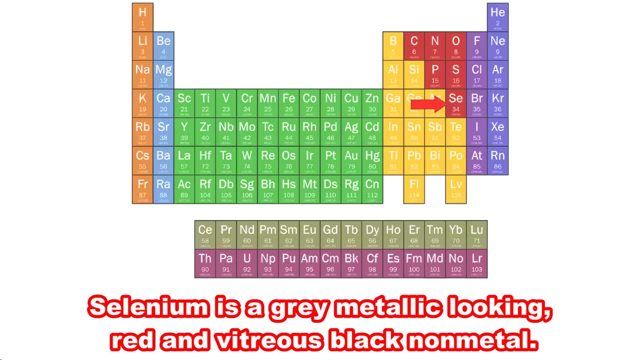 120 dollars per kilogram as of 2020. number 33: arsenic. arsenic is a gray per kilogram as of 2020. number 34: selenium. selenium is a gray, metallic looking red and vitreous black. nonmetal selenium is used to make pigments for. 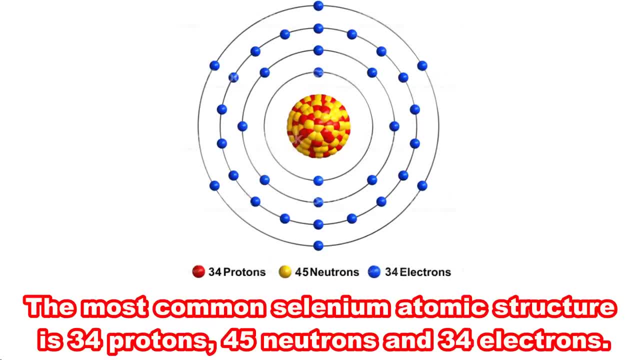 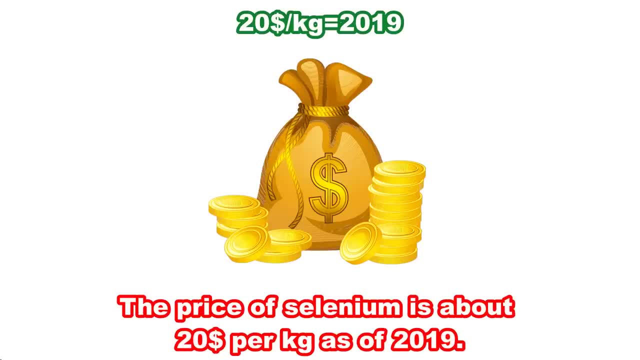 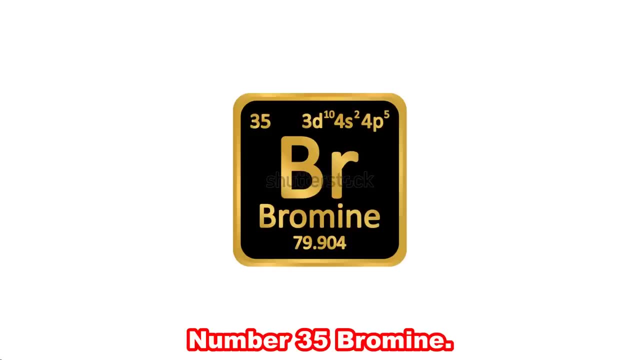 ceramics, paint and plastics. the most common selenium atomic structure is 34 protons, 45 neutrons and 34 electrons. the price of selenium is about $20 as of 2019. number 35, bromine: bromine is a light reddish brown. halogen bromine is: 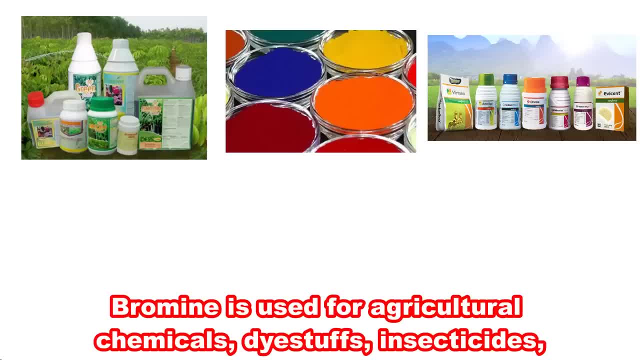 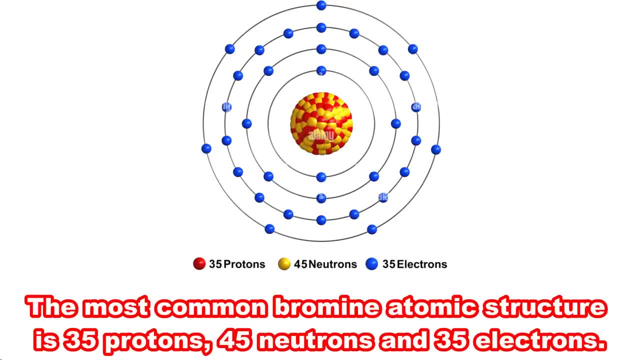 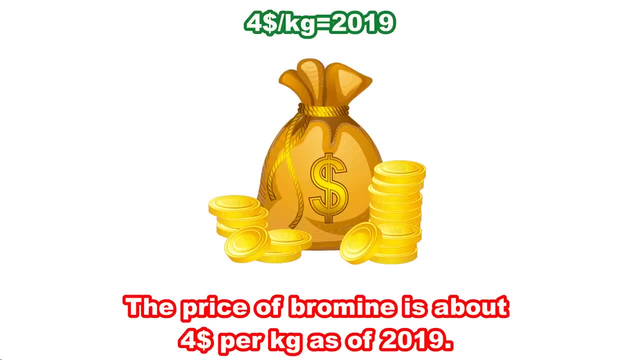 used for agricultural chemicals, dye stuffs, insecticides, pharmaceuticals and chemical intermediates. the most common bromine atomic structure is 35 protons, 45 neutrons and 35 electrons. the price of bromine is about $4 per kilogram as of 2019. 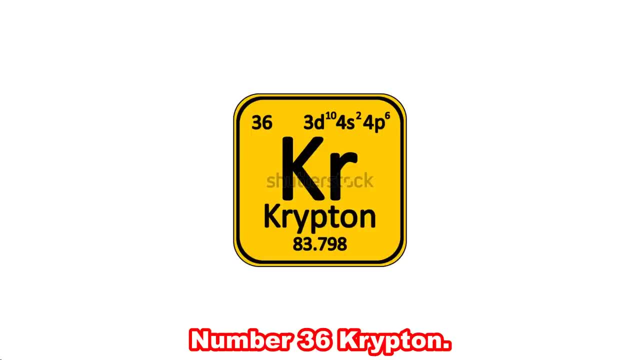 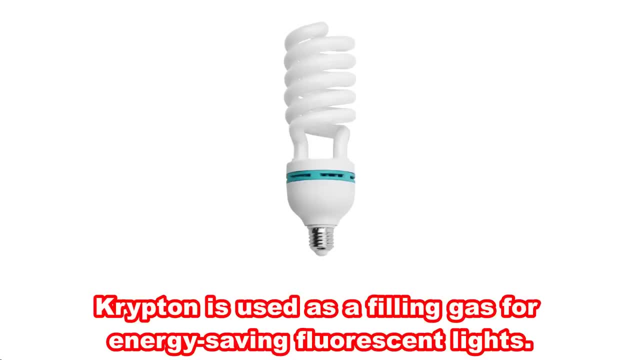 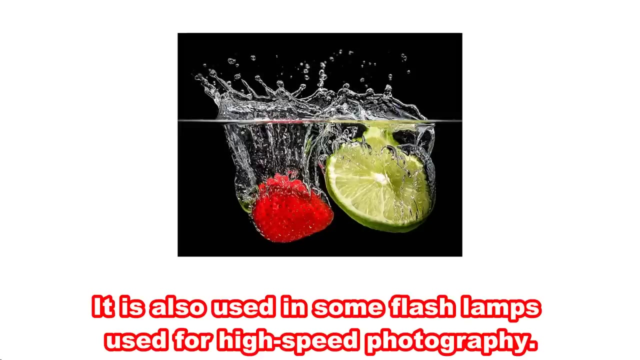 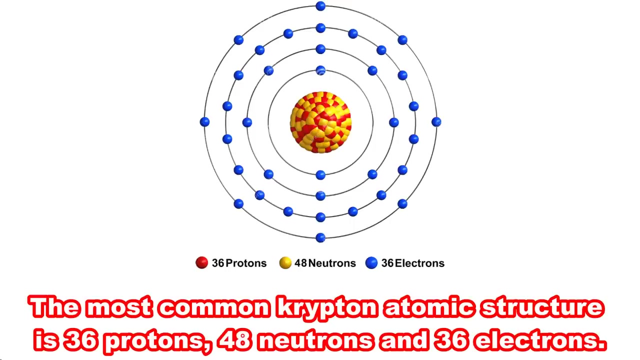 you No 36, krypton. krypton is a colorless, odorless, tasteless, noble gas. krypton is used as a filling gas for energy-saving fluorescent lights. it is also used in some flash lamps used for high-speed photography. the most common krypton atomic structure is 36 protons, 48 neutrons and 36 electrons. the price of 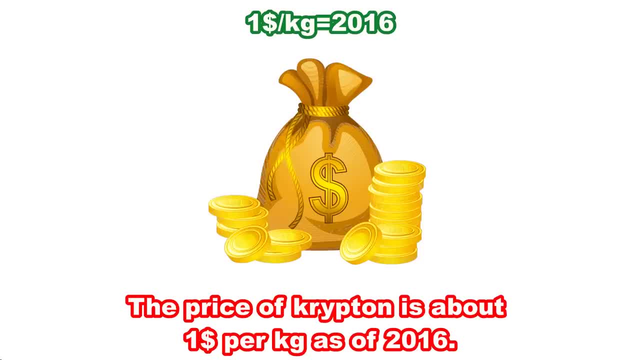 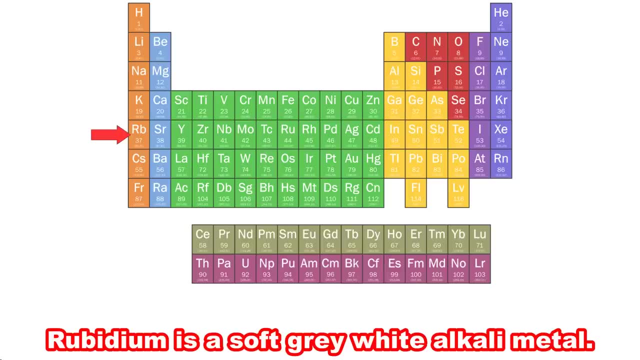 krypton is about $1 per kilogram as of 2016. number 37: rubidium. rubidium is a soft gray- white alkali metal. rubidium is used in a component of photocells to remove traces of oxygen from vacuum tubes and. 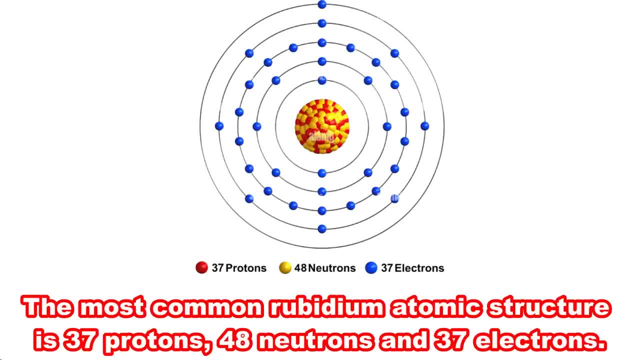 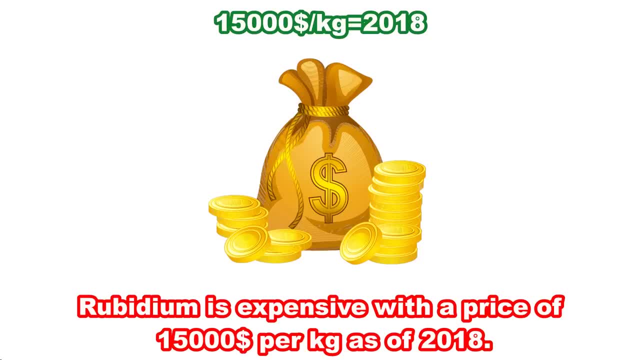 to make special types of glass. the most common rubidium atomic structure is 37 protons, 48 neutrons and 37 electrons. rubidium is expensive, with the price of $15,000 per kilogram as of 2018. number 37 rubidium is a soft, gray, white alkali metal. rubidium is used in a component of photocells, to remove traces of oxygen from vacuum tubes and to make special types of glass. the most common rubidium atomic structure is 37 protons, 48 neutrons and 37 electrons. rubidium is expensive, with the price of $15,000 per kilogram as of 2018. 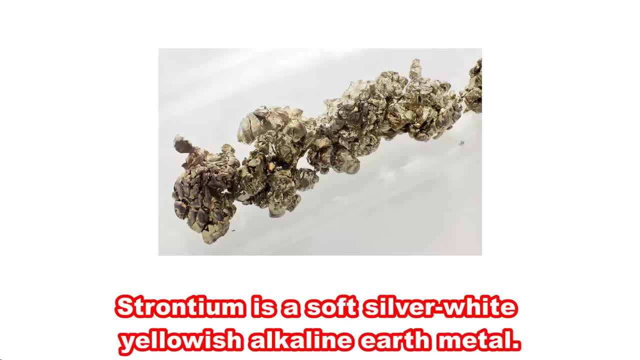 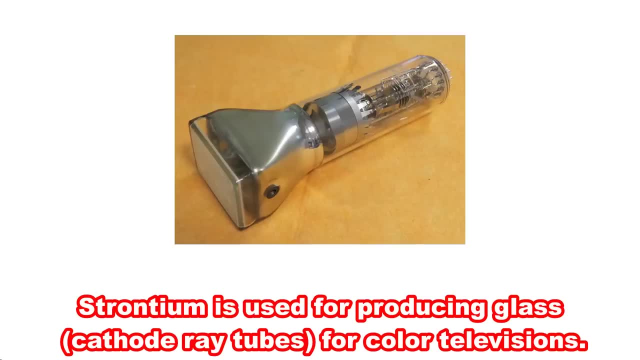 number 38, strontium. strontium is a soft, silver, white, yellow, ish alkaline earth types of glass and photos millionaire metal. strontium is used for producing glass for color televisions. strontium has also been used in the world's most accurate atomic clock. 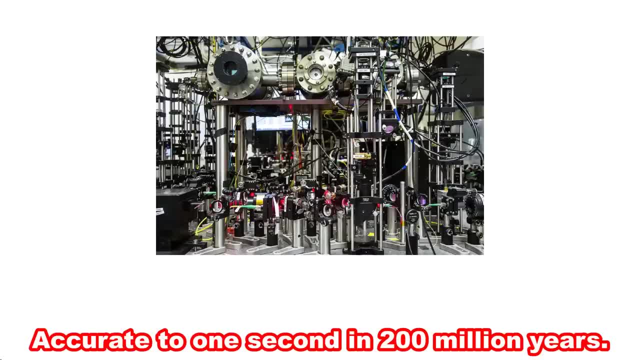 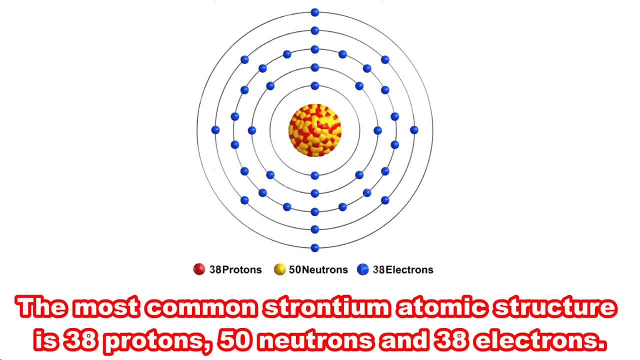 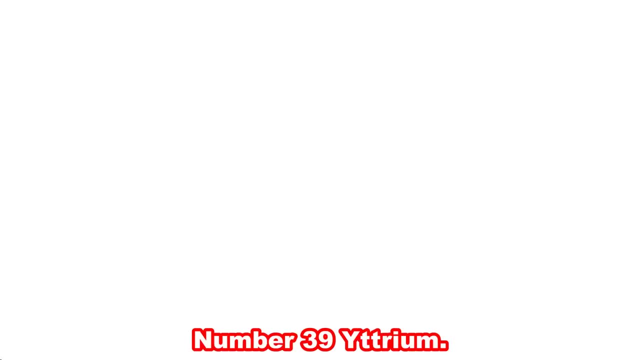 accurate to 1 second in 200 million years. the most common strontium atomic structure is 38 protons, 15 neutrons and 38 electrons. the price of strontium is of 2019. number 39 atrium atrium is a silvery, white transition metal. it is a. 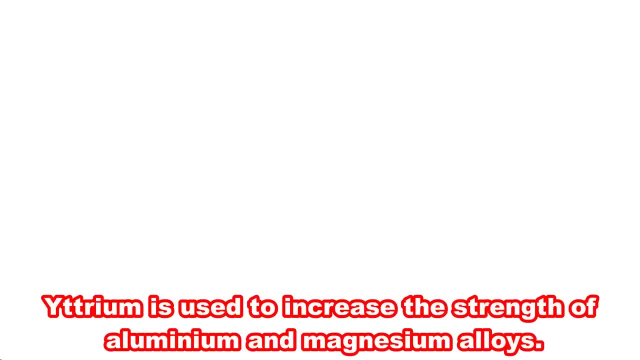 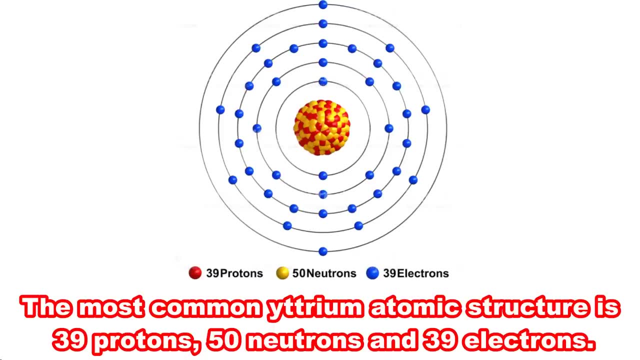 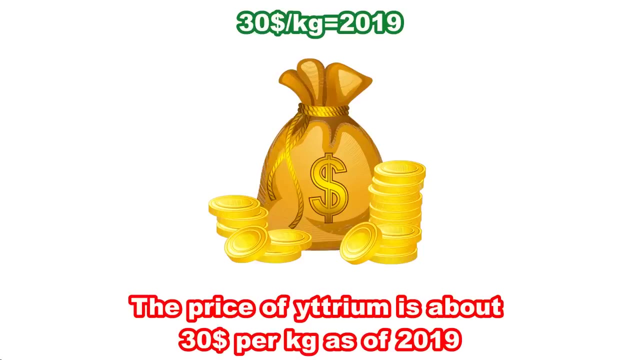 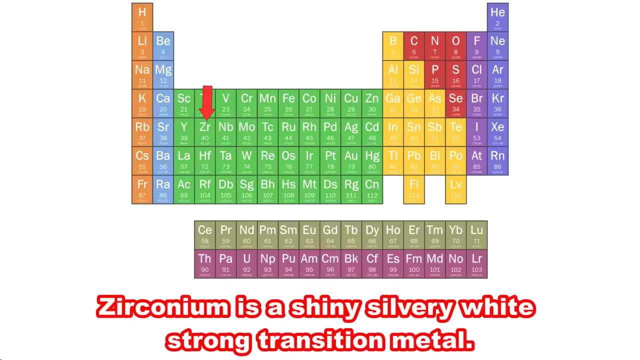 rare earth element. atrium is used to increase the strength of aluminium and magnesium alloys. the most common atrium atomic structure is 39 protons, 50 neutrons and 39 electrons. the price of atrium is about $30 per kilogram as of 2019. number 40: zirconium. zirconium is a shiny, silvery, white, strong transition. 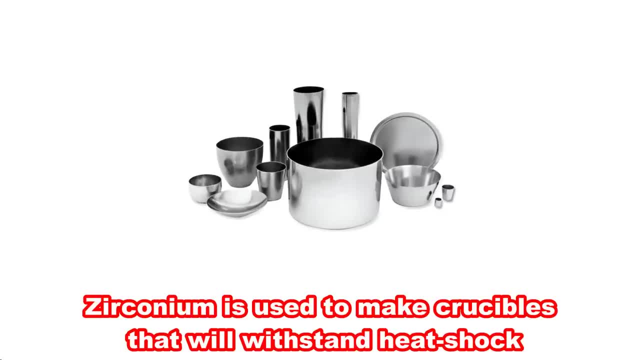 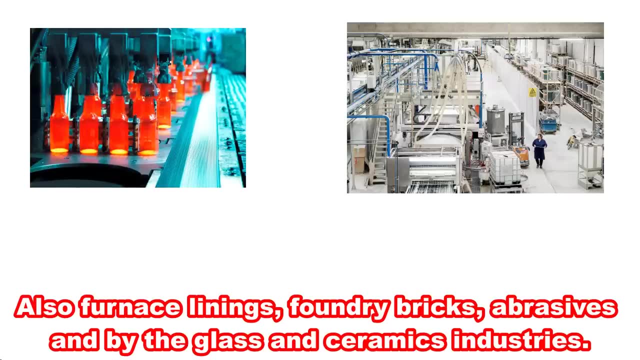 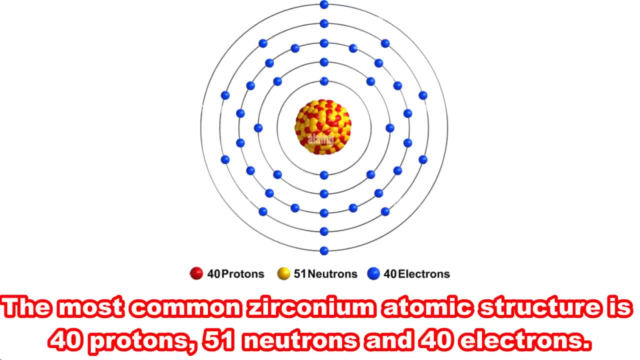 metal. zirconium is used to make crucibles that will withstand heat shock, also furnace linings, foundry bricks, abrasives, and by the glass and ceramics industries. the most common zirconium atomic structure is 40 protons, 51 neutrons and 40 electrons. the price of zirconium is about. 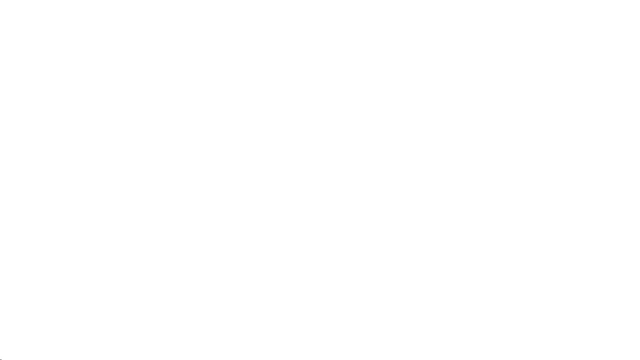 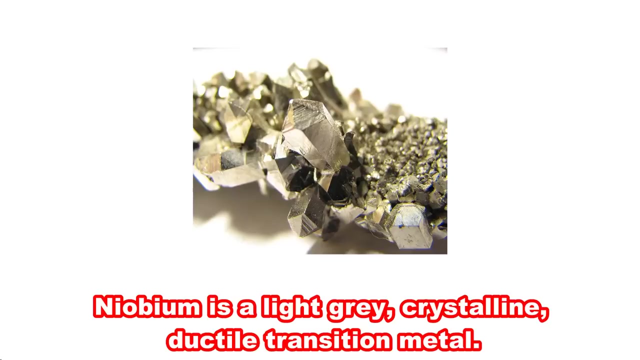 $美元. atrium atomic structure is 50 prorne's, 51 neutrons and 40 electrons. the price of zirconium is about $ dollars. actually most important atrium atrium reflecting a high standard, it was $36 per kilogram as of 2020. number 41: niobium. niobium is a light gray crystalline ductile. 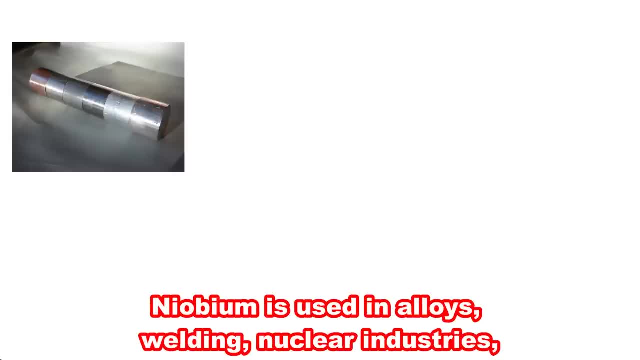 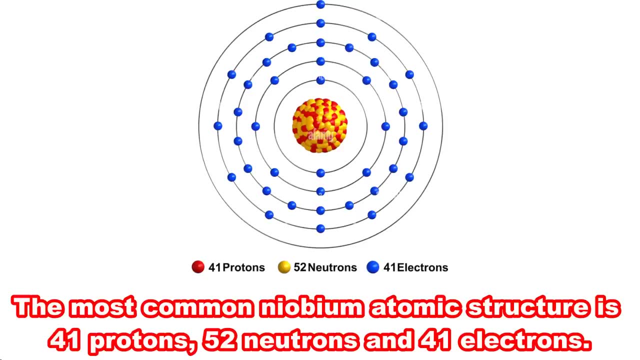 transition metal. niobium is used in alloys, welding, nuclear industries, electronics, optics, numismatics and jewelry. the most common niobium atomic structure is 41 protons, 52 neutrons and 41 electrons. the price of niobium is about seventy dollars per kilogram as of 2020. 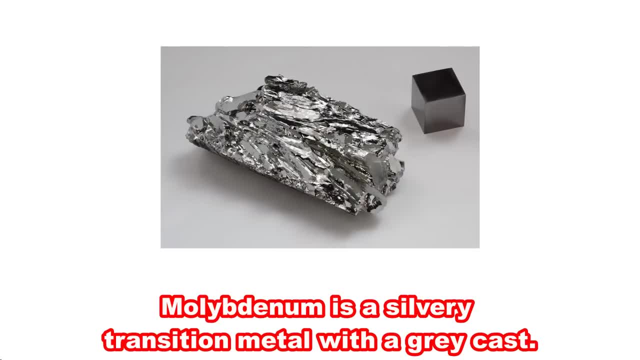 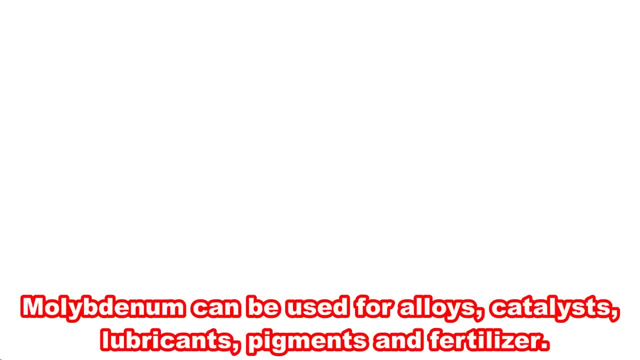 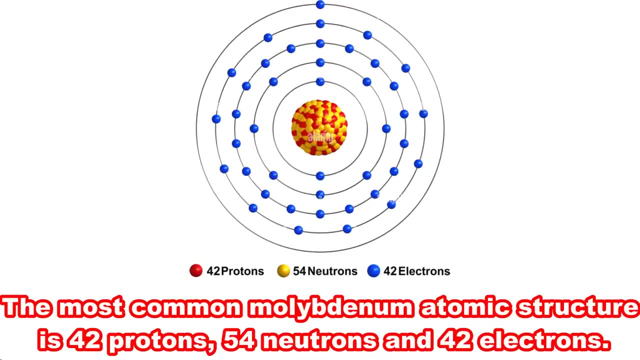 number 42, molybdenum. molybdenum is a silvery transition metal with a gray cast. it has a high melting point. molybdenum can be used for alloys, catalysts, lubricants, pigments and fertilizer. the most common molybdenum atomic structure is 42 protons, 54 neutrons and 42 electrons. 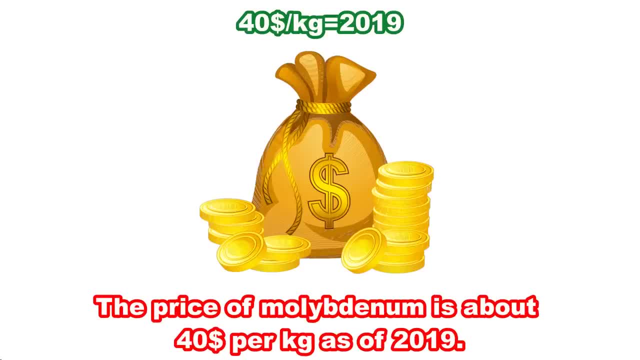 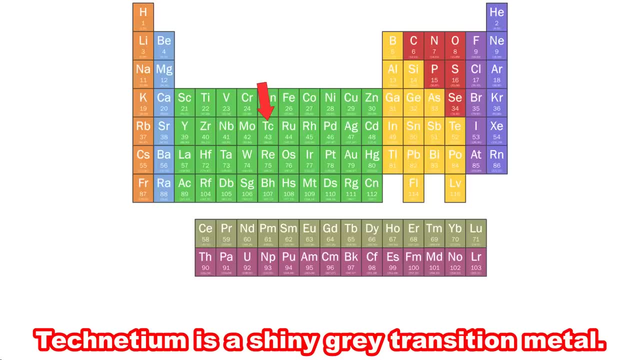 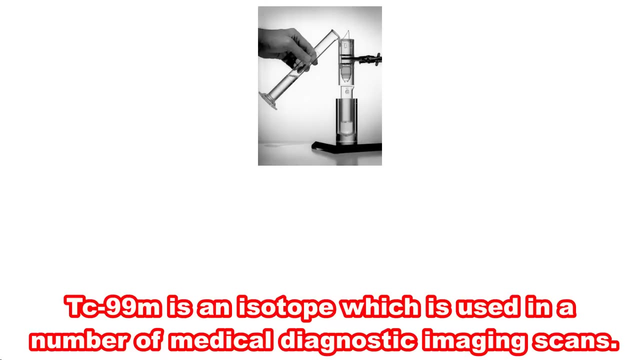 the price of molybdenum is about forty dollars per kilogram as of 2019. number 43: technetium. technetium is a shiny, gray transition metal. it is also a man-made element. all technetium isotopes are radioactive. tc99m is an isotope which is used in a number of medical 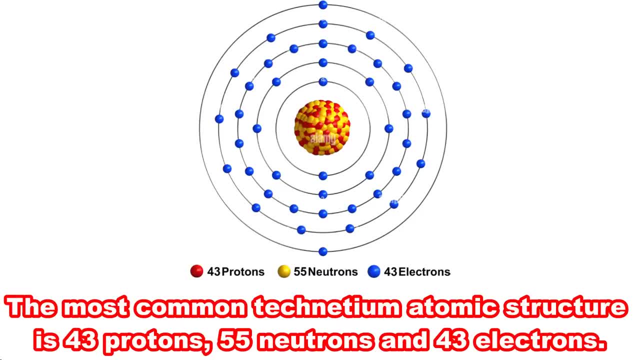 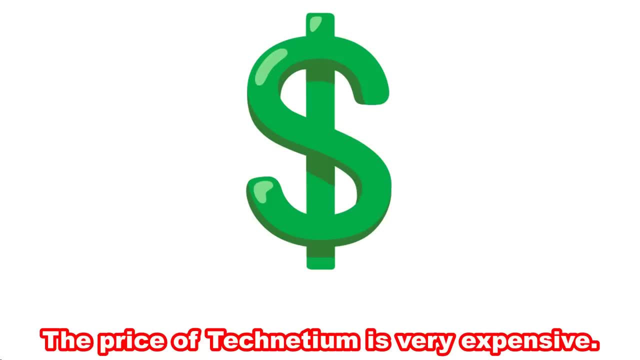 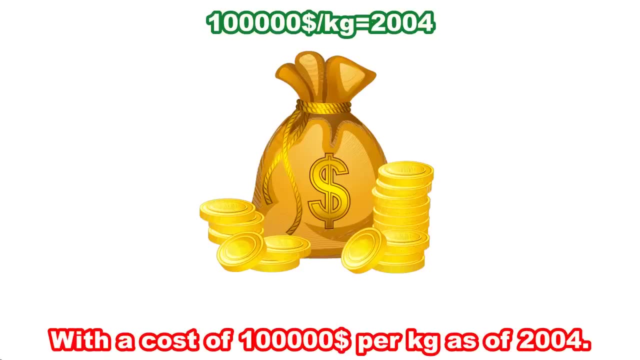 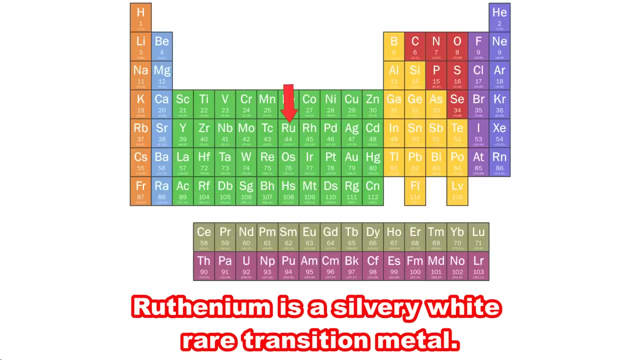 diagnostic imaging scans. the most common technetium atomic structure is 43 protons, 55 neutrons and 43 electrons. the price of technetium is very expensive, with a cost of 100 000 per kilogram as of 2004.. number 44: ruthenium. ruthenium is a silvery, white, rare transition metal. ruthenium is used to 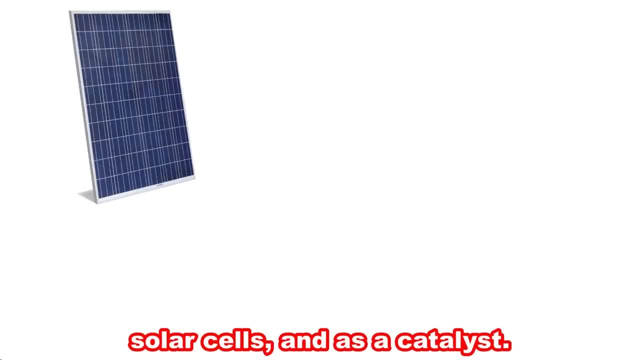 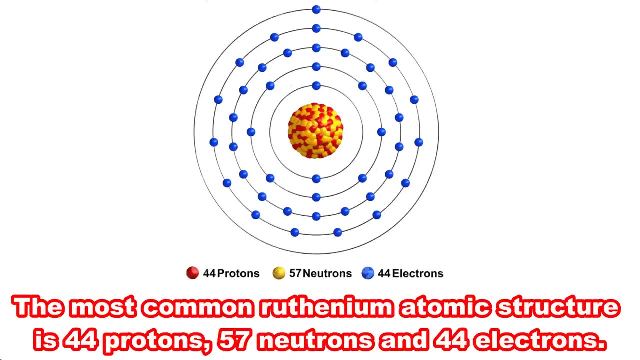 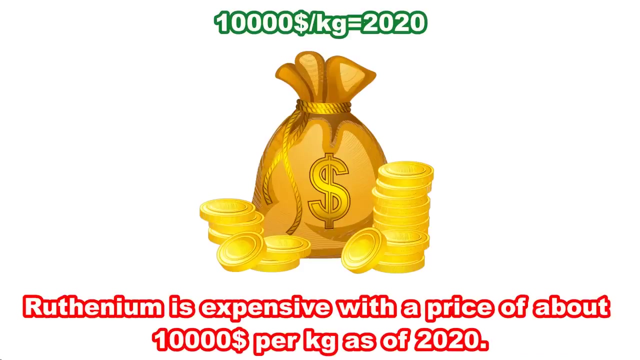 make jewelry, electrical contacts, solar cells and as a catalyst. the most common ruthenium atomic structure is 44 protons, 57 neutrons. the most common ruthenium atomic structure is 44 protons and 44 electrons. ruthenium is expensive, with a price of about 10 000 per kilogram as of 2020. 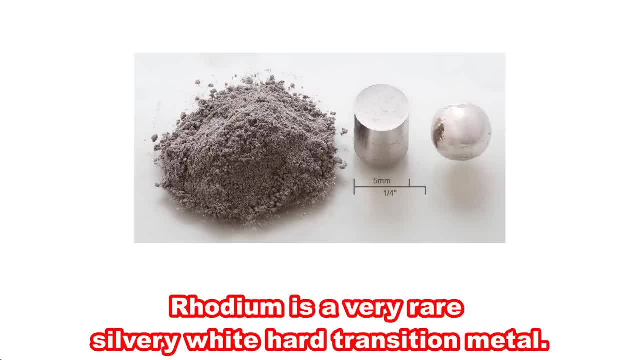 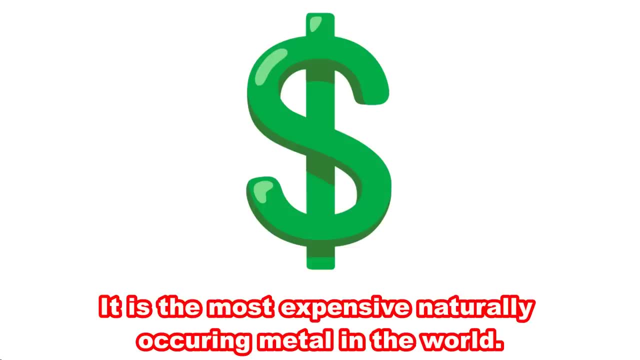 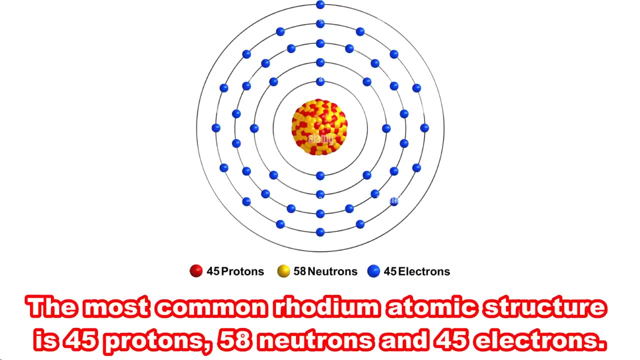 number 45, rhodium. rhodium is a very rare silvery- white hard transition metal. it is the most expensive naturally occurring metal in the world. the major use of rhodium is in catalytic converters for cars, but also jewelry. the most common rhodium atomic structure is 45 protons. 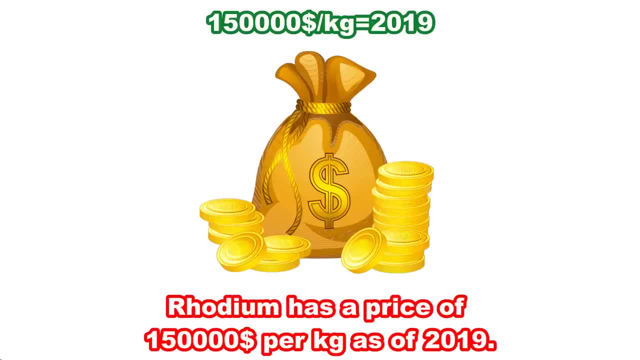 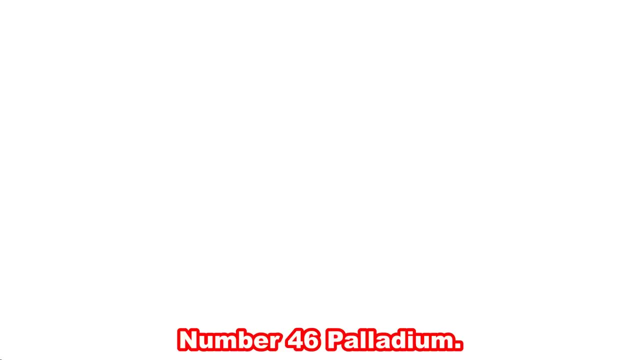 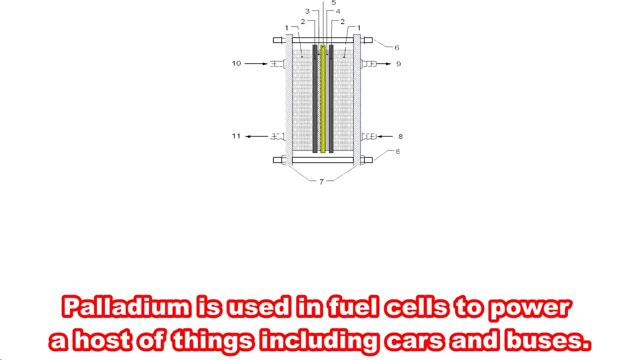 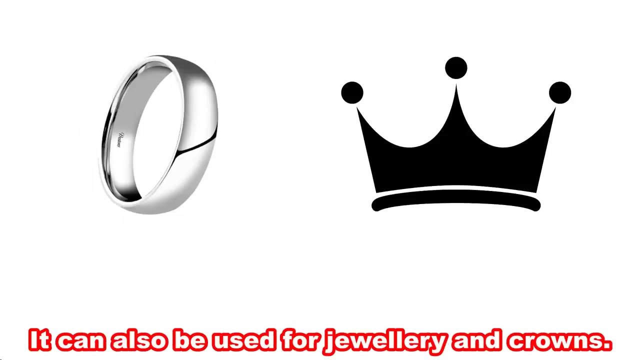 rhodium has a price of 150 000 per kilogram as of 2019.. number 46: palladium. palladium is a rare, shiny, silvery white transition metal. palladium is used in fuel cells to power a host of things, including cars and buses. it can also be used for jewelry and crowns. the most common palladium atomic structure: 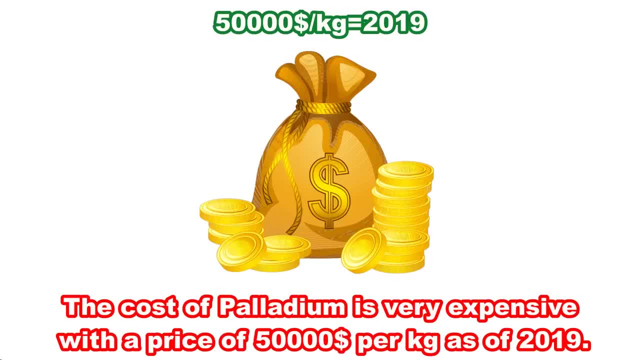 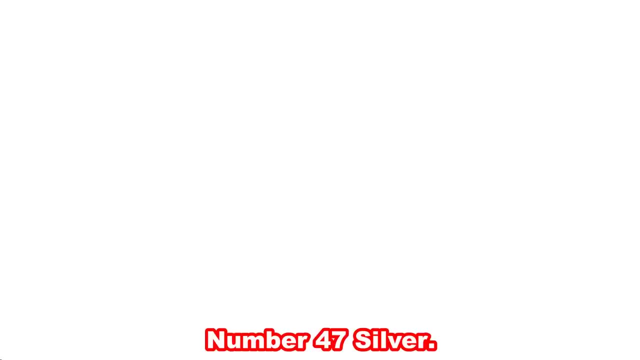 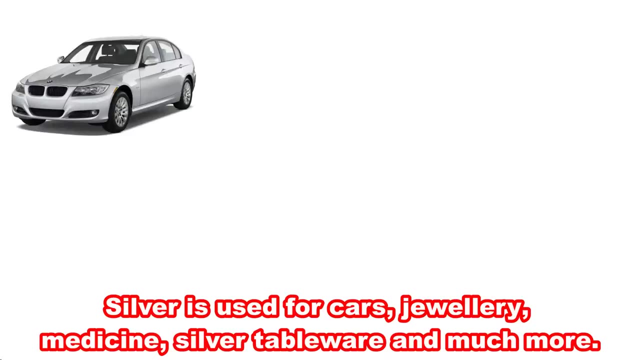 60 neutrons and 46 electrons. the cost of palladium is very expensive, with a price of 50 000 per kilogram as of 2019.. number 47: silver. silver is a soft, white, shiny transition metal. silver is used for cars, jewelry, medicine, silver tableware and much more. the most. 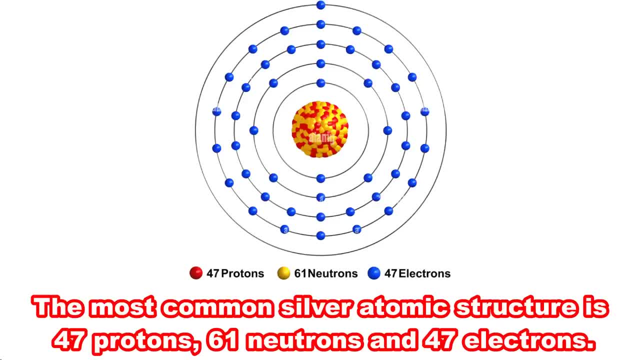 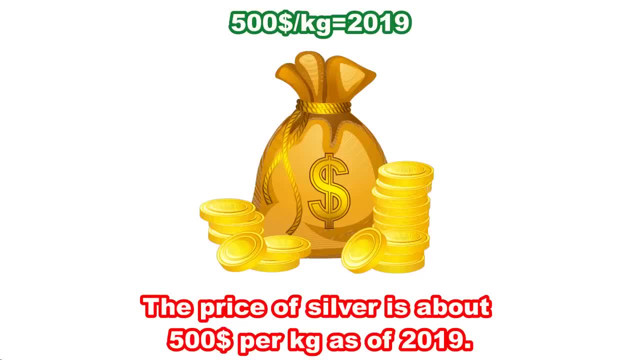 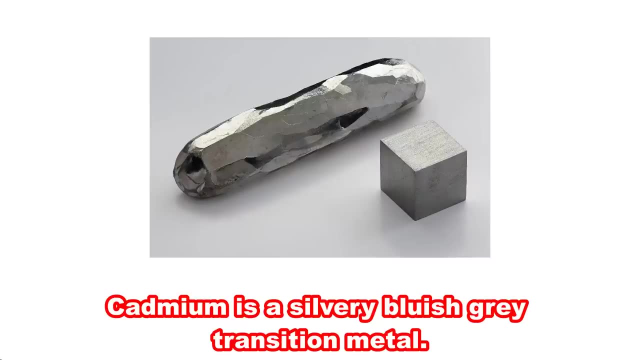 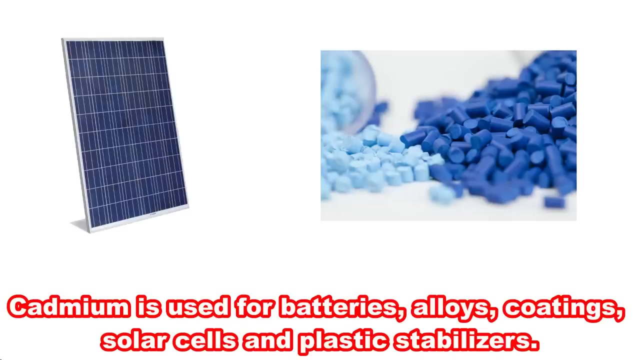 common silver atomic structure is 47 protons, 61 neutrons and 47 electrons. price of silver is about 500 per kilogram as of 2019.. number 48: cadmium. cadmium is a silvery, bluish, gray transition metal. cadmium is used for batteries, alloys, coatings, solar cells and plastic. 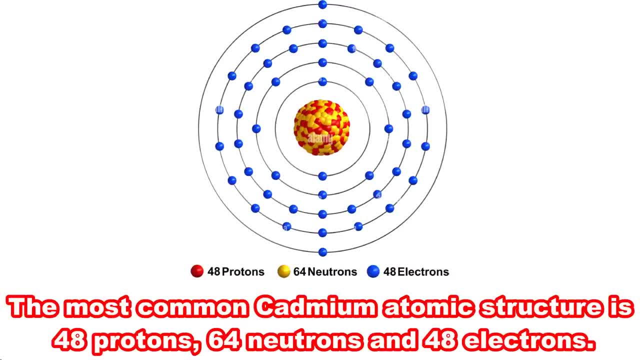 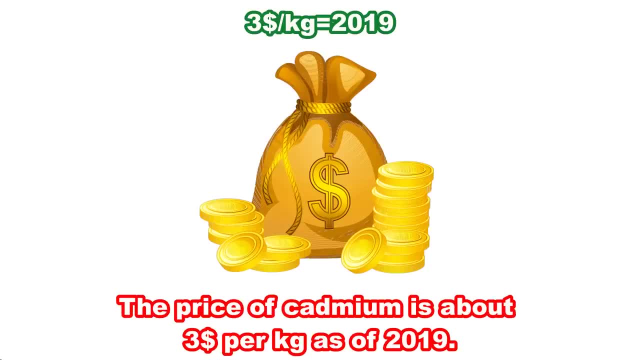 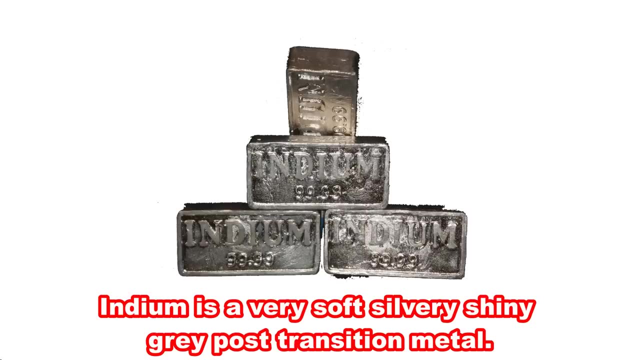 stabilizers. the most common cadmium atomic structure is 48 protons, 64 neutrons and 48 electrons. the price of cadmium is about three dollars per kilogram as of 2019.. number 49: indium. indium is a very soft, silvery, shiny, gray post transition metal. most indium is 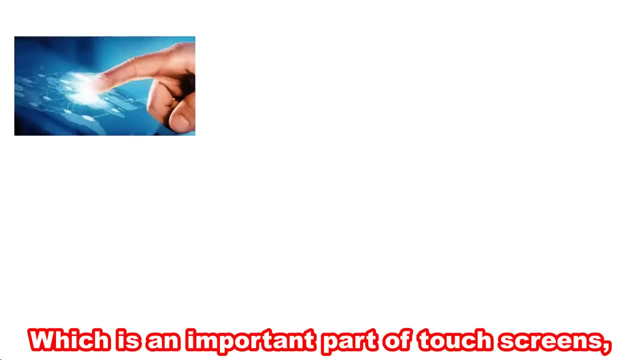 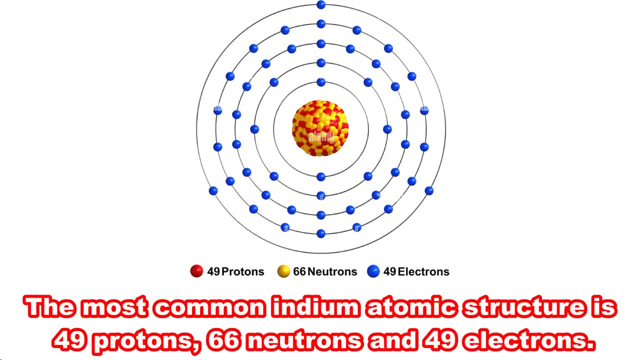 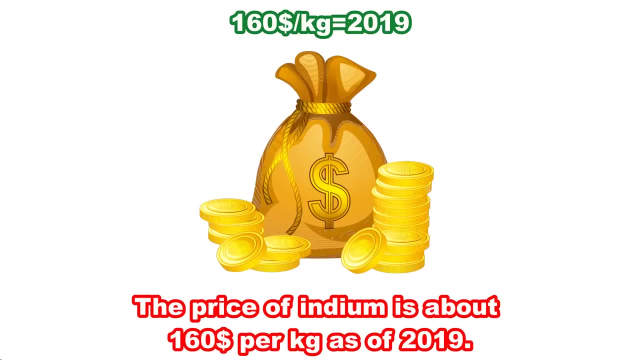 used to make indium tin oxide, which is an important part of touch screens, flat screen tvs and solar panels. the most common indium atomic structure is 49 protons, 66 neutrons and 49 electrons. the price of indium is about 160 dollars per kilogram as 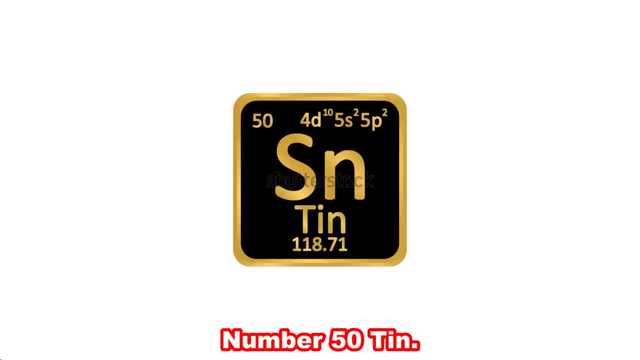 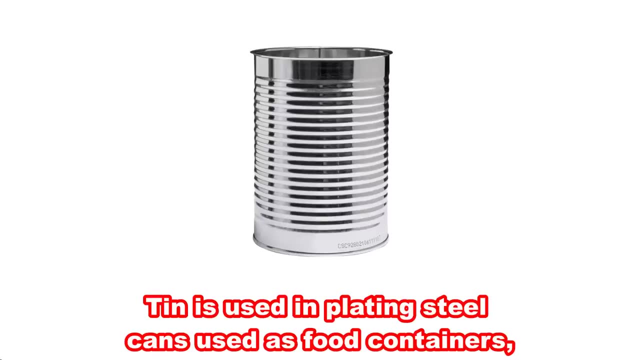 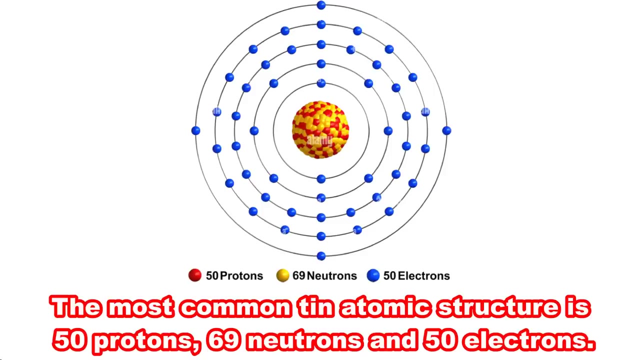 of 2019.. number 50: tin. tin is a very soft silvery white post transition metal. tin is used in plating steel cans, used as food containers, in metals used for bearings and in soldiers. the most common tin atomic structure is 50 protons, 69 neutrons and 50 electrons. 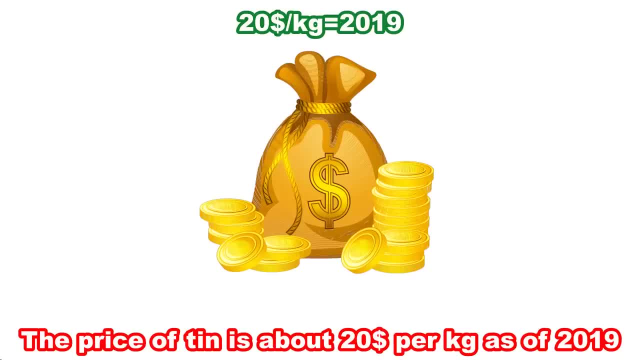 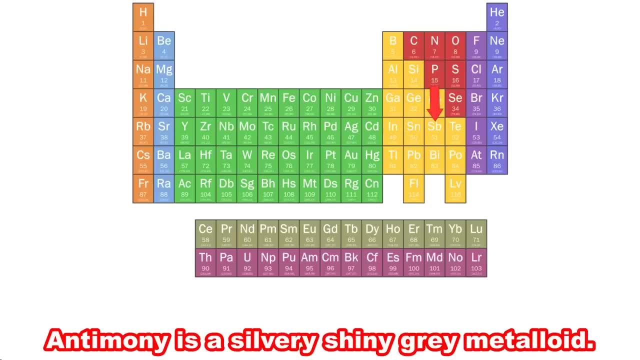 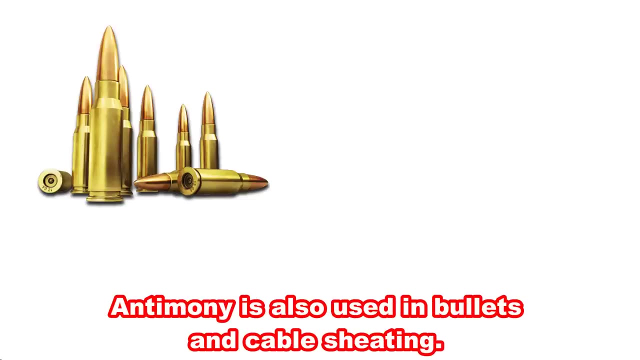 the price of tin is about 20 dollars per kilogram as of 2019.. number 51: antimony. antimony is a silvery, shiny gray metalloid. antimony can be used to increase the hardness of alloys. antimony is also used in bullets and cable sheeting. the most common antimony atomic structure: 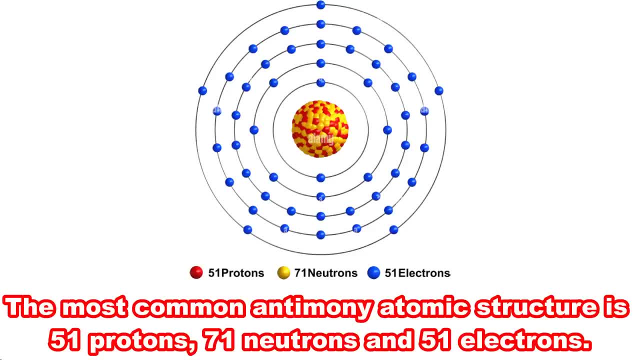 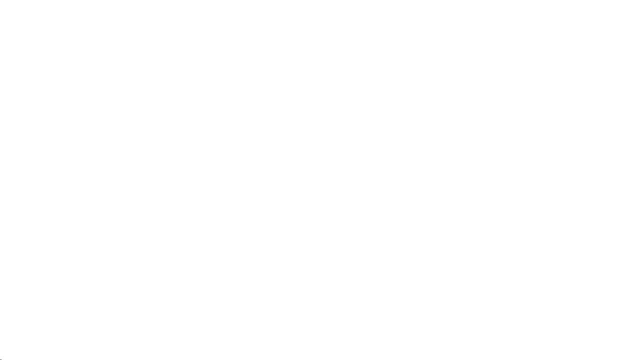 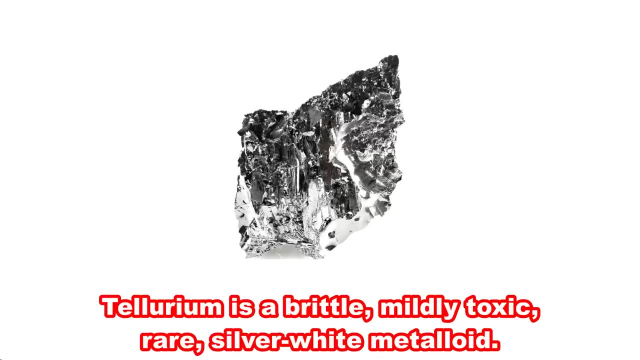 is 51 protons, 71 neutrons and 51 electrons. the price of antimony is about six dollars per kilogram as of 2019.. number 52 tellurium tellurium is a brittle, mildly toxic. rare silver white metalloid tellurium can be used to vulcanize. 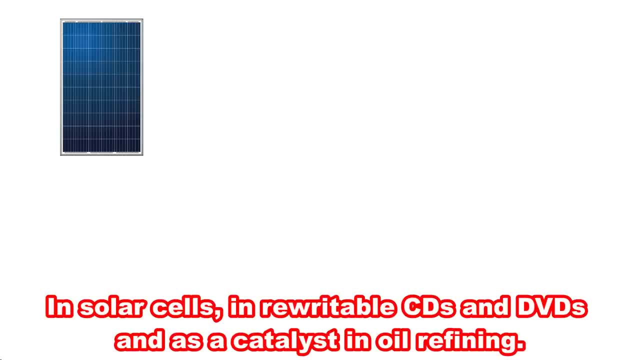 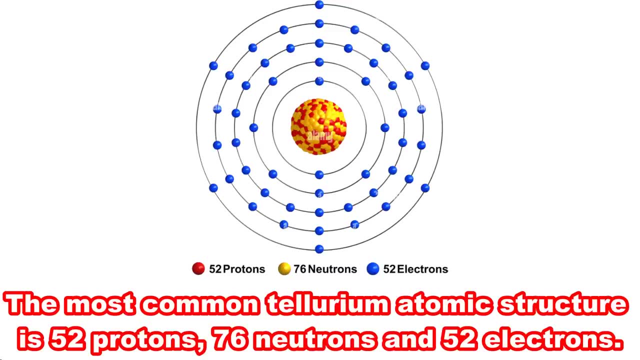 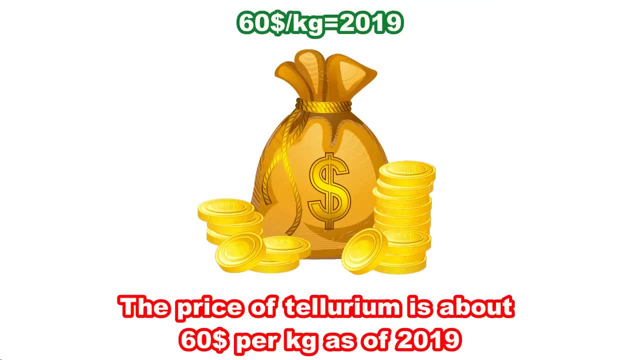 rubber to tint glass and ceramics, in solar cells, in rewritable cds and dvds and as a catalyst in oil refining. the most common tellurium atomic structure is 52 protons, 76 neutrons and 52 electrons. the price of tellurium is about sixty dollars per kilogram as of 2019.. 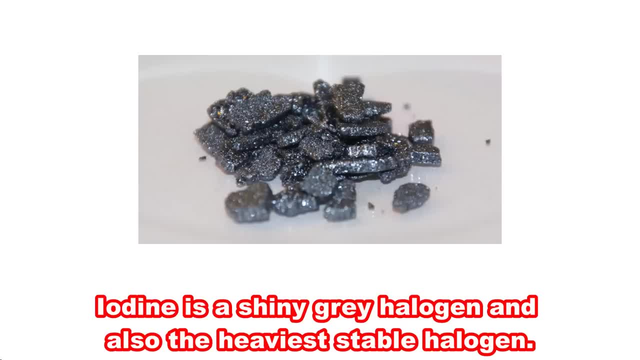 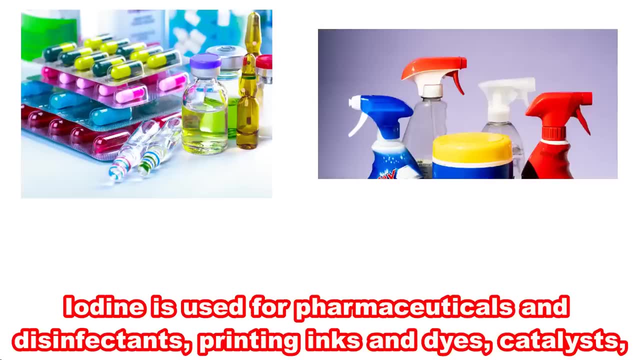 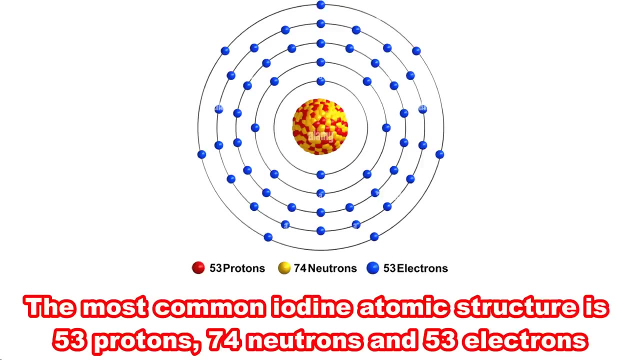 number 53, iodine. iodine is a shiny gray halogen and also the heaviest stable halogen. iodine is used for pharmaceuticals and disinfectants, printing inks and dyes, catalysts, animal feed supplements and photographic chemicals. the most common iodine atomic structure: 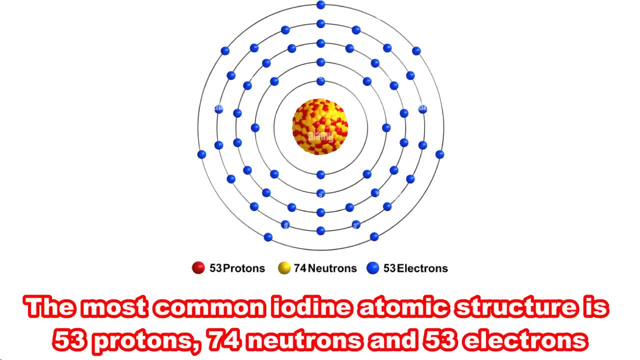 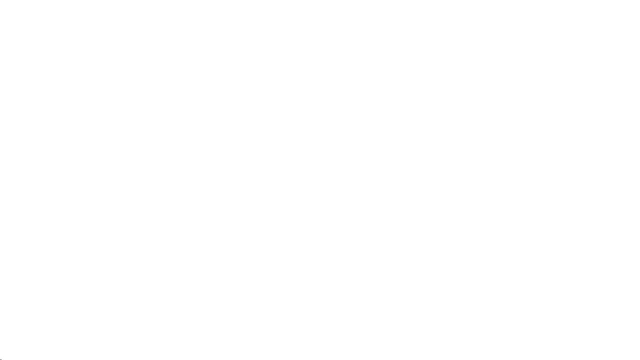 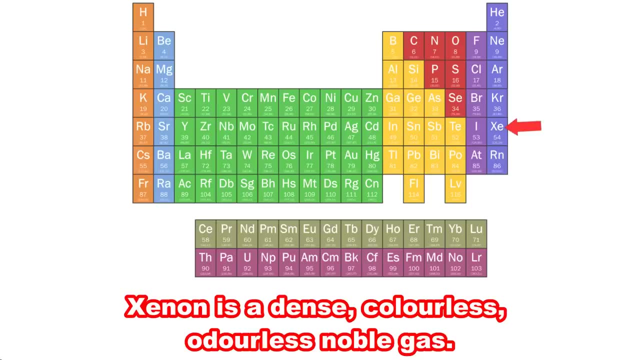 is 53 protons, 74 neutrons and 53 electrons. the price of iodine is about 35 dollars per kilogram as of 2019.. number 54: xenon. xenon is a dense, colorless, odorless noble gas. xenon isn't used. 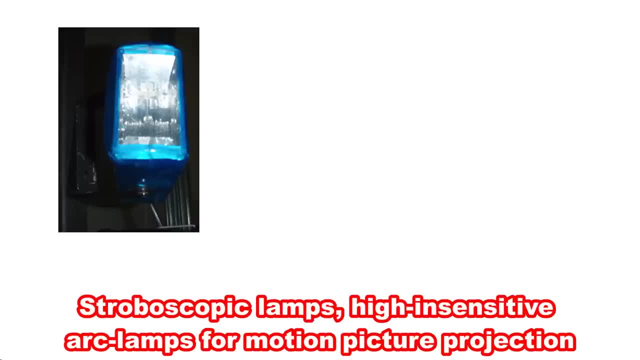 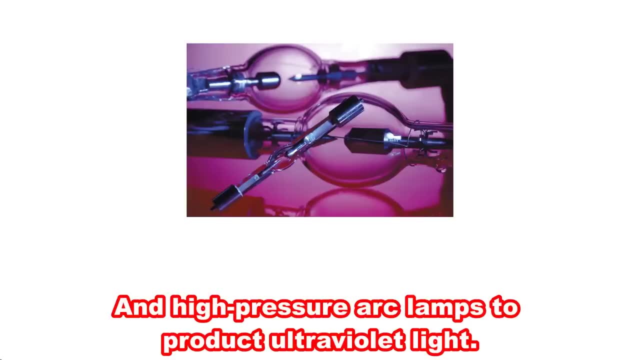 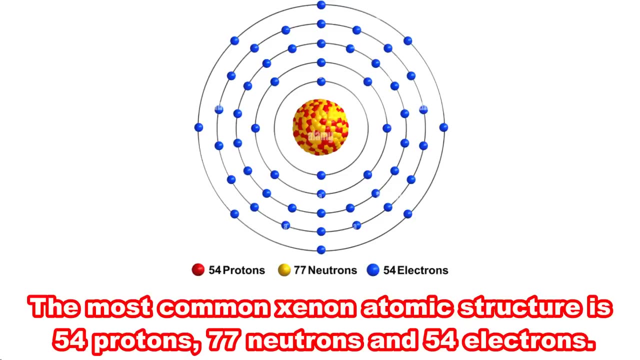 for so much, but it is used in photographic flash lamps, stroboscopic lamps, high insensitive arc lamps for motion picture projection and high pressure arc lamps to product ultraviolet light. the most common xenon atomic structure is 54 protons, 77 neutrons and 54 electrons. 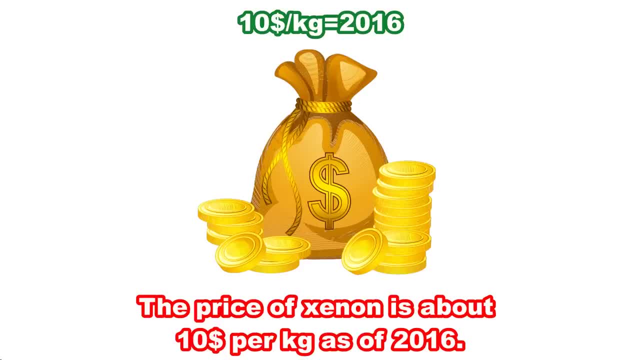 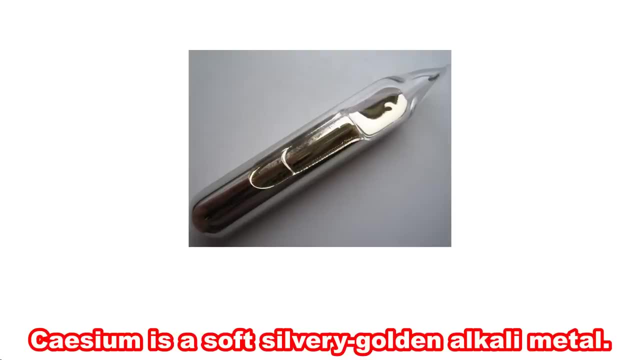 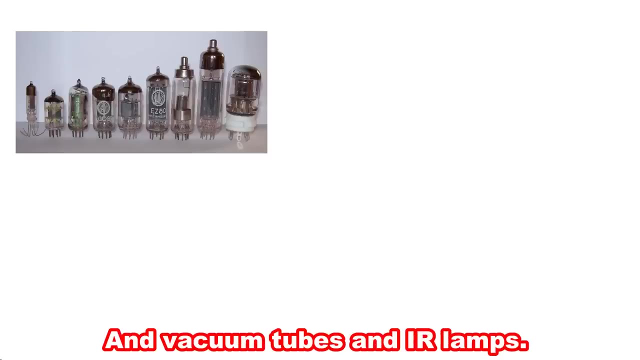 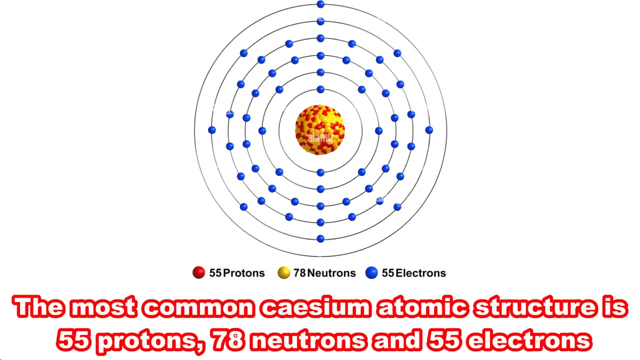 the price of xenon is about 10 per kilogram as of 2016.. number 55: cesium. cesium is a soft, silvery, golden alkali metal. cesium is used as a drilling fuel, a catalyst, photoelectric cells and vacuum tubes and ir lamps. the most common cesium atomic structure is 55 protons, 78 neutrons and 55. 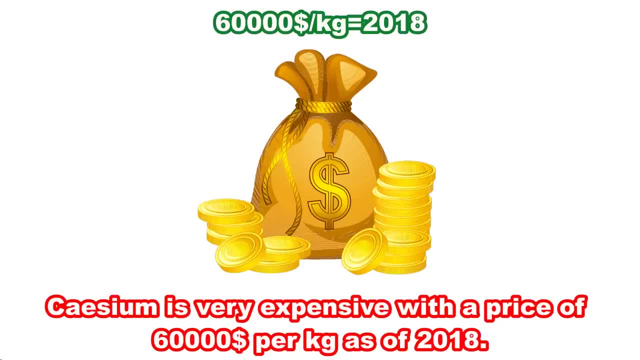 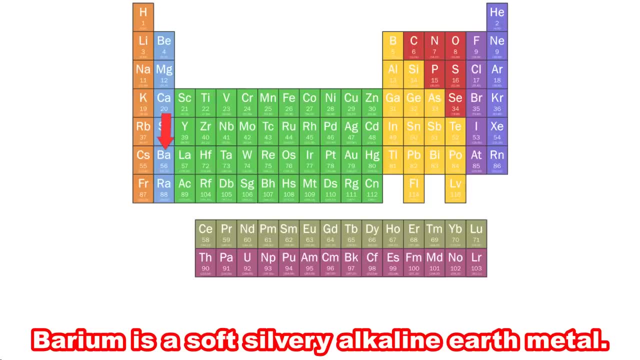 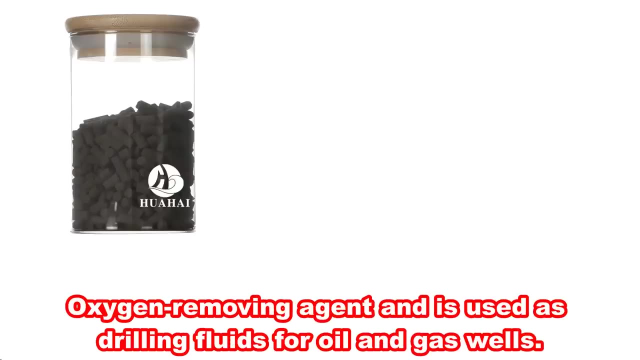 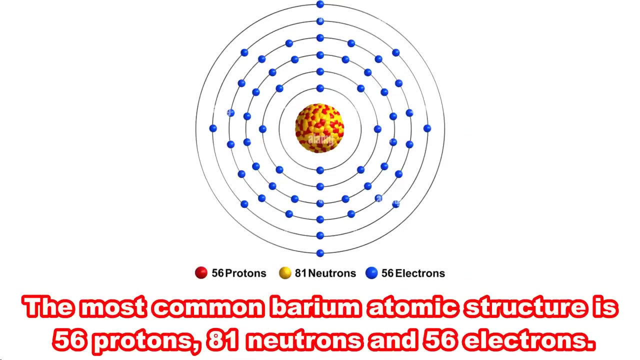 electrons. so people think it is an atomic structure but it is not. it is a neutron. the most common xenon atomic structure is 56 protons, 81 neutrons and 56 electrons. baryam is a soft, silvery, alkaline earth metal. baryam is used for spark plug electrodes and in vacuum tubes as a drying oxygen removing agent and is used as drilling fluids for oil and gas wells. the most common barium atomic structure is 56 protons, 81 neutrons and 56 electrons. baryam is the most common atomic structure. baryam atomic is a gainer of oxygen and is used as a drying agent in the Jasmine. 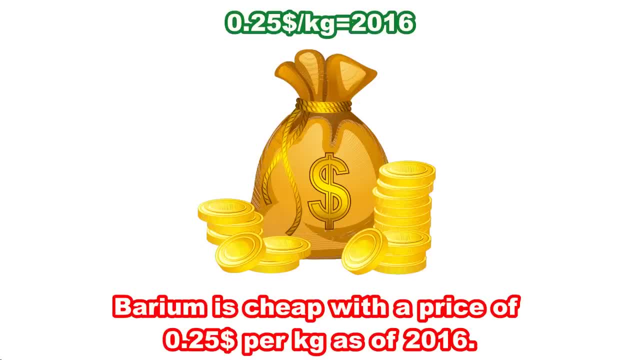 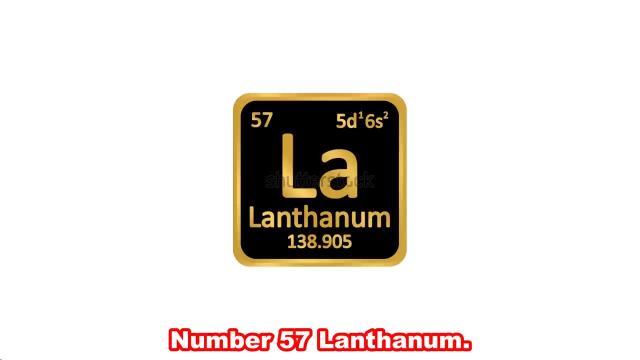 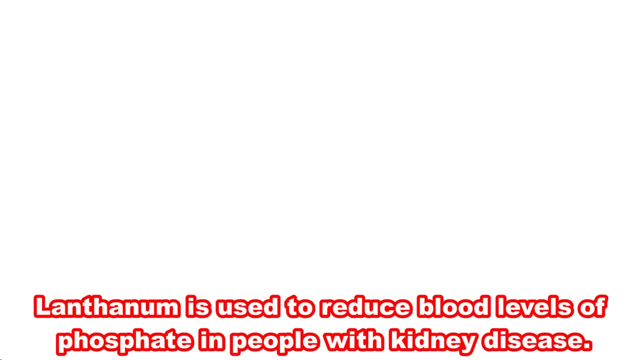 cheap, with a price of 25 cents per kilogram as of 2016. now on to all the lanthanides: number 57: lanthanum. lanthanum is a soft ductile. silvery white lanthanide. lanthanum is used to reduce blood levels of phosphate in people with 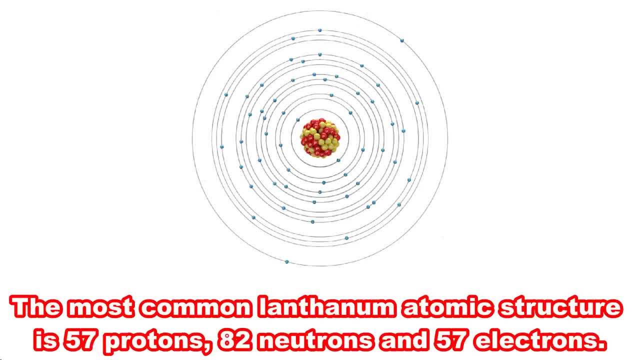 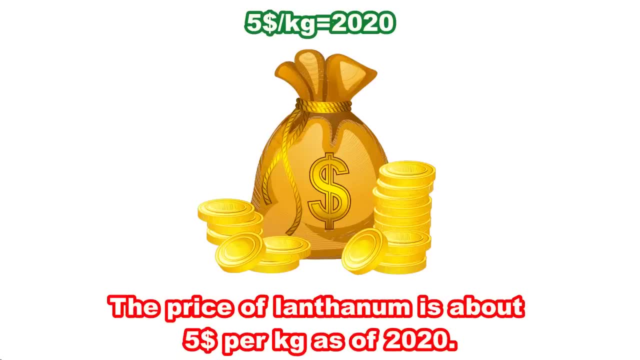 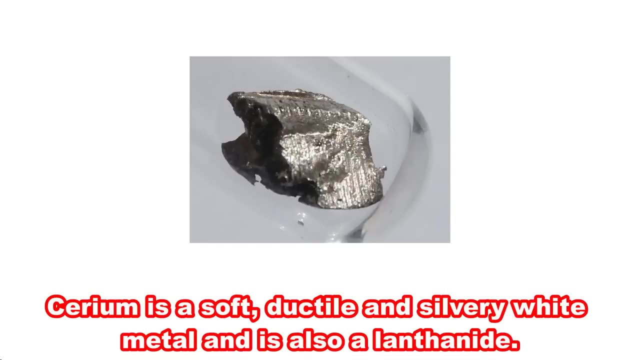 kidney disease. the most common lanthanum atomic structure is 57 protons, 82 neutrons and 57 electrons. the price of lanthanum is about five dollars per kilogram as of 2020. number 58, cerium. cerium is a soft, ductile and silvery 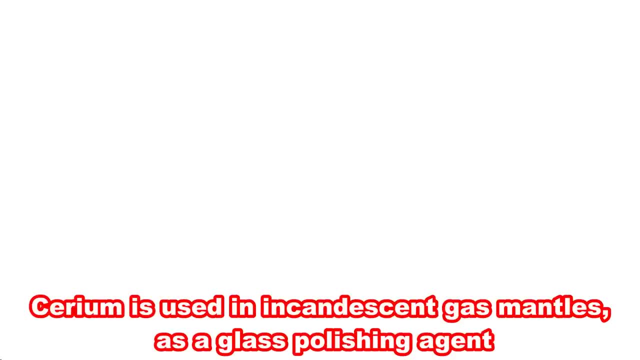 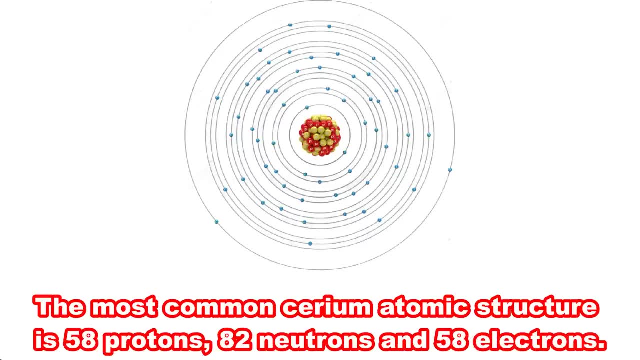 white metal and is also a lanthanide. cerium is used in incandescent gas mantles, as a glass polishing agent and as a catalyst in self-cleaning ovens. the most common cerium atomic structure is 58 protons, 82 neutrons and 58. 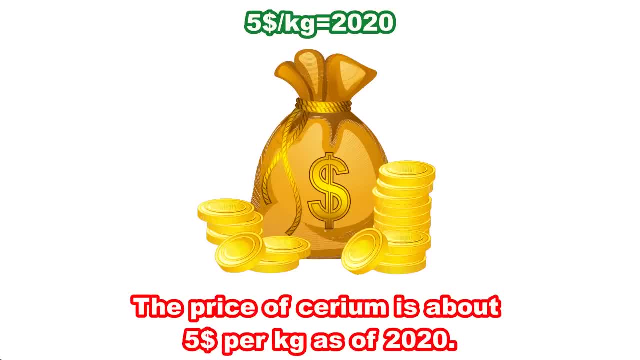 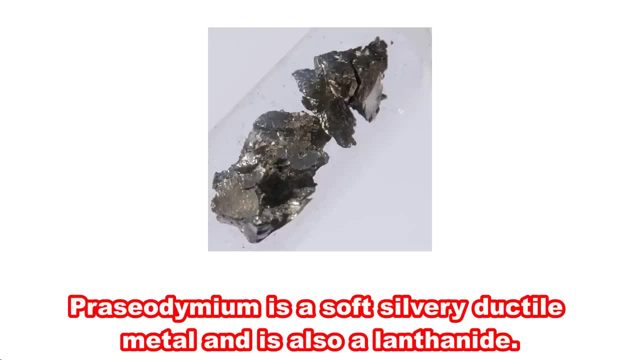 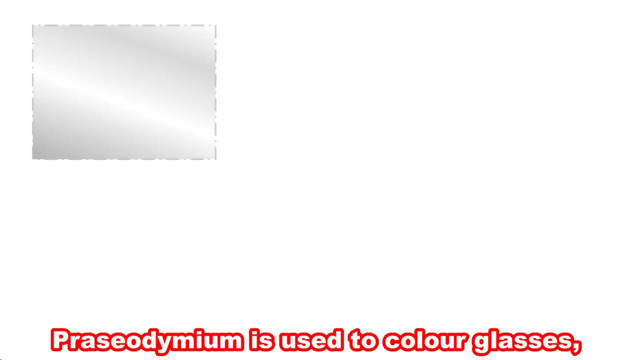 electrons. the price of cerium is about five dollars per kilogram as of 2020. number 59: preysiodymium. preysiodymium is a soft, silvery, ductile metal and is also lanthanide. preysiodymium is used to color glasses, enamel glazes, an intense 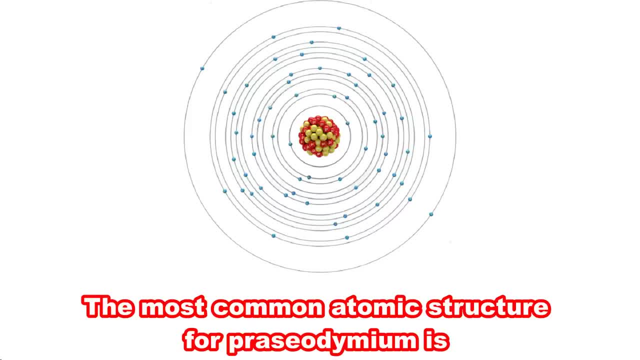 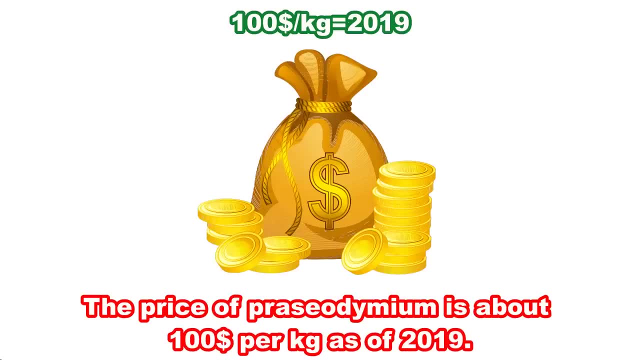 and unusually clean yellow. the most common atomic structure for preysiodymium is 59 protons, 82 Neutrons and 59 electrons. the price of cerium and lanthanide. Eagles camouflaged of ciserulic iron and don'ttinidine black. 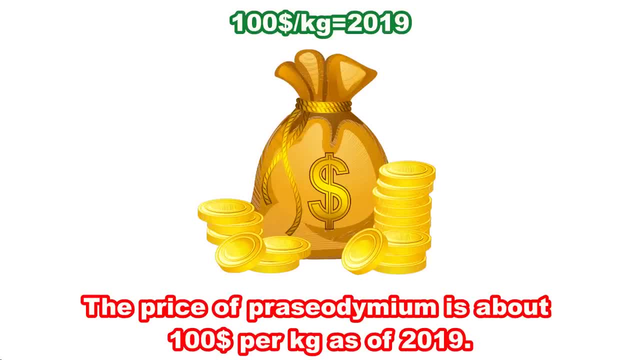 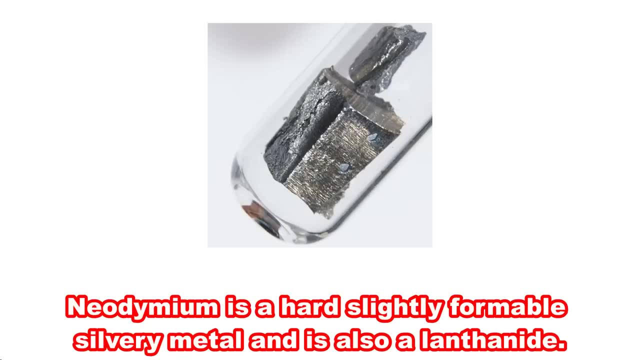 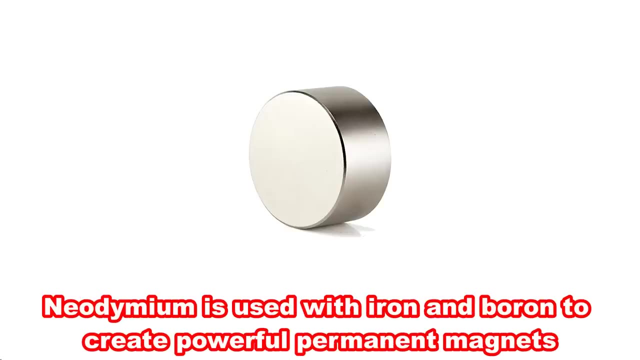 of praseodymium is about $100 per kilogram as of 2019.. Number 60. Neodymium. Neodymium is a hard, slightly formable silvery metal and is also a lanthanide. Neodymium is used with iron and boron to create powerful permanent magnets, which is used in 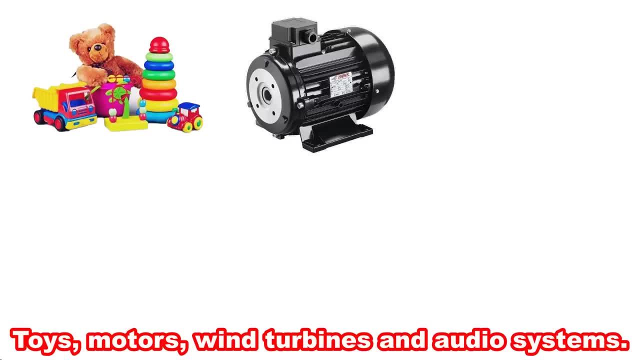 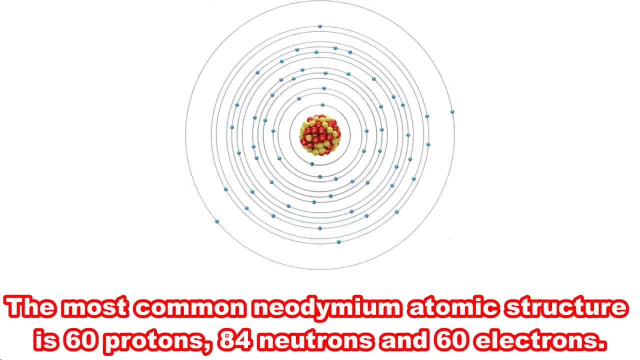 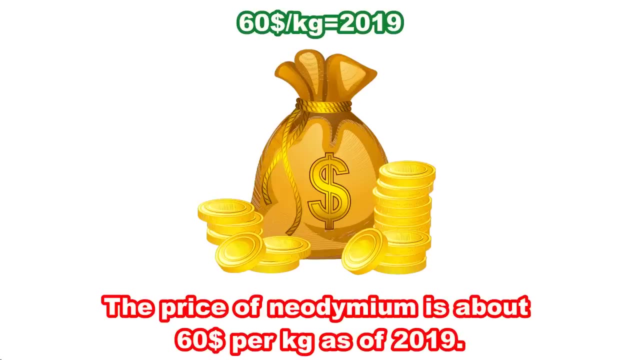 computers, cell phones, medical equipment, toys, motors, wind turbines and audio systems. The most common neodymium atomic structure is 60 protons, 84 neutrons and 60 electrons. The price of neodymium is about $60 per kilogram as of 2019.. 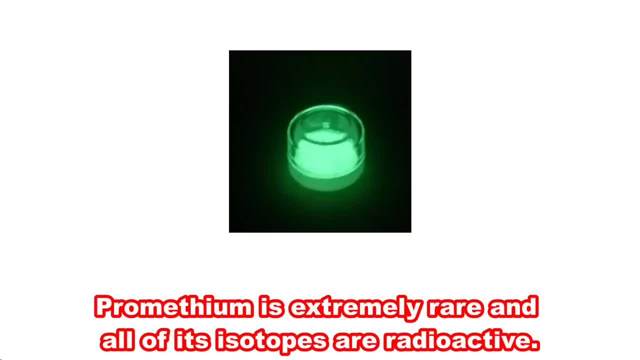 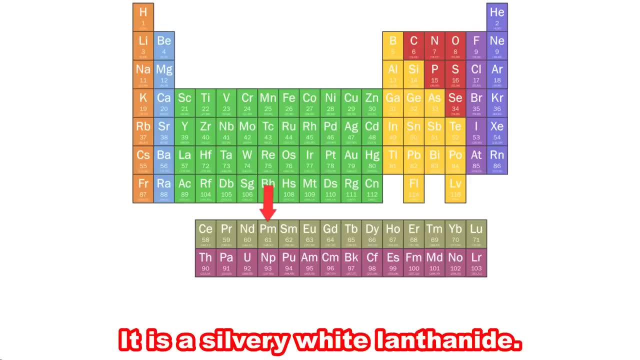 Number 61. Prometheum. Prometheum is extremely rare and all of its isotopes are radioactive. It is a silvery white lanthanide. Almost every prometheum we have is used in research. The most common prometheum atomic structure is neodymium. 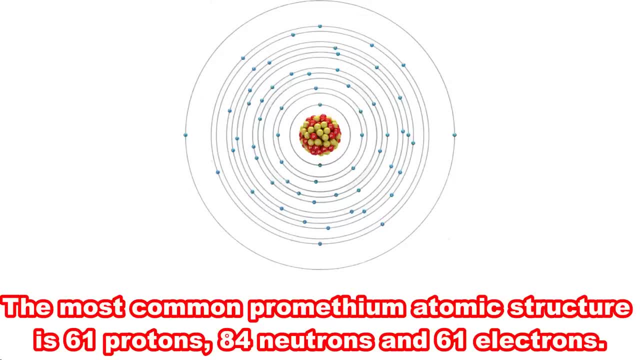 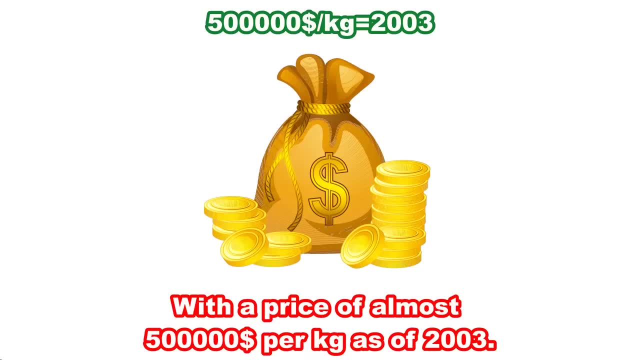 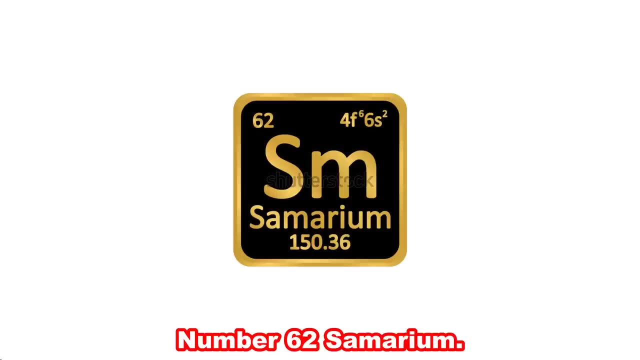 Number 60. is 61 protons, 84 neutrons and 61 electrons. the price of promethean 147 is extremely expensive, with a price of almost half a million dollars per kilogram as of 2003. number 62: samarium. samarium is a pretty hard silvery metal. 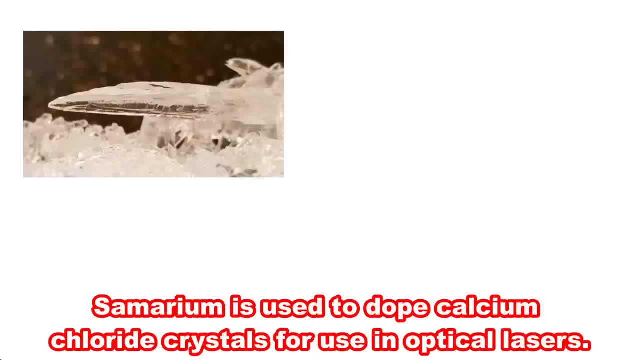 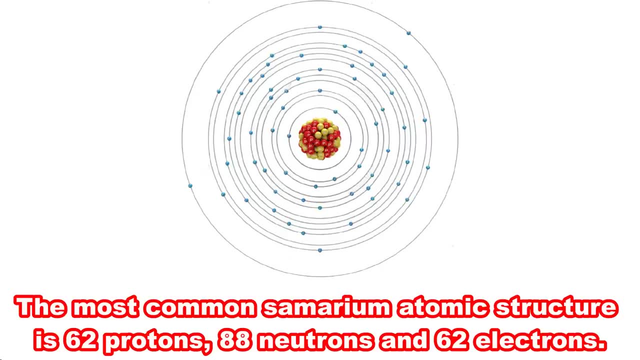 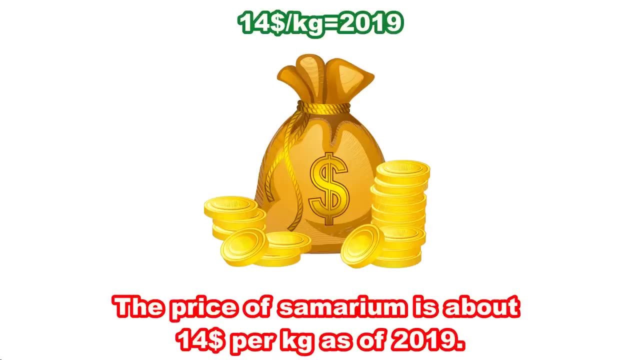 and also a lanthanide. samarium is used to dope calcium chloride crystals for use in optical lasers. the most common samarium atomic structure is 62 protons, 88 neutrons and 62 electrons. the price of samarium is about $14 per kilogram. 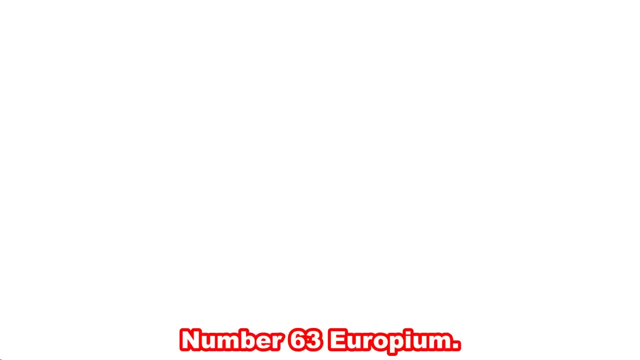 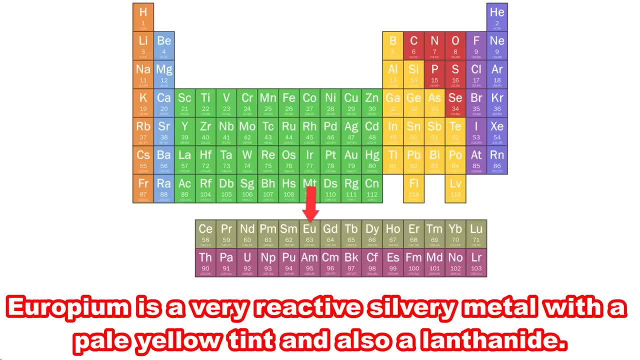 as of 2019. number 63: europium. europium is a very reactive silvery metal with a pale yellow tint and also a lanthanide. europium is very good at absorbing neutrons, making it valuable in control rods for nuclear power plants and nuclear power plants. and nuclear power plants are. 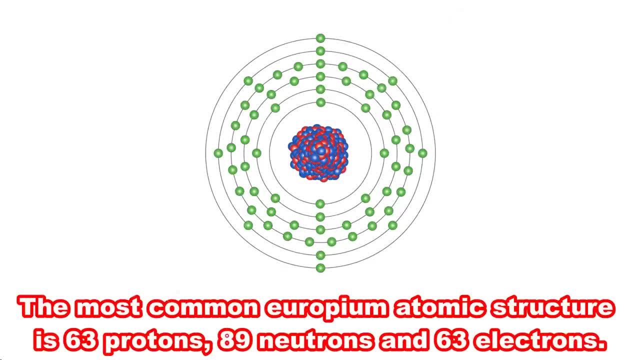 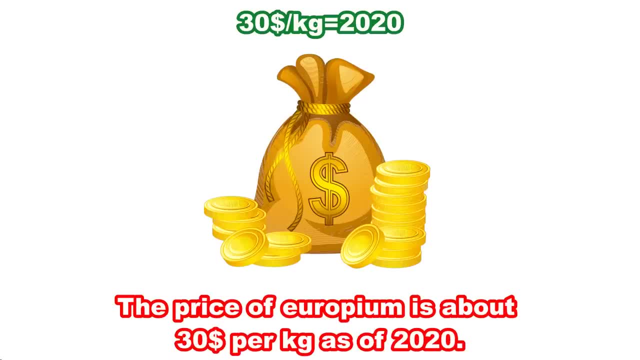 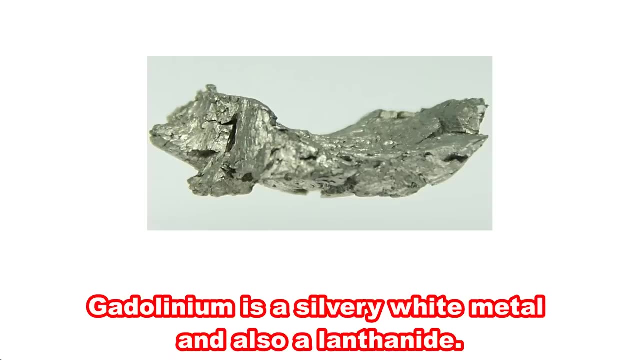 nuclear reactors. the most common europium atomic structure is 63 protons, 89 neutrons and 63 electrons. the price of europium is about $30 per kilogram as of 2020. number 64: gadolinium. gadolinium is a silvery white metal and also a. 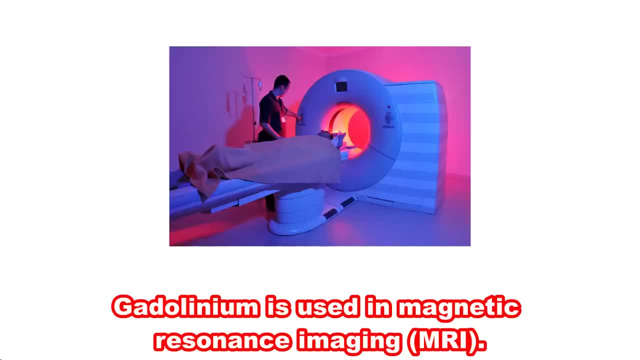 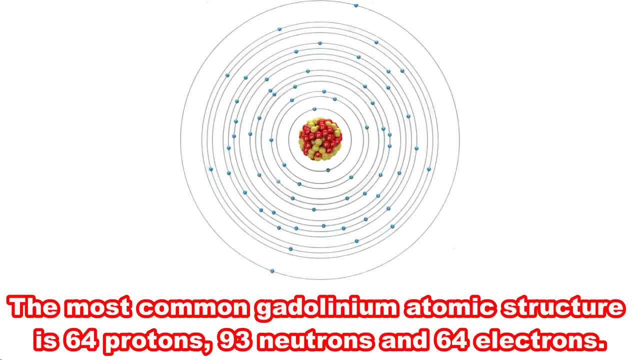 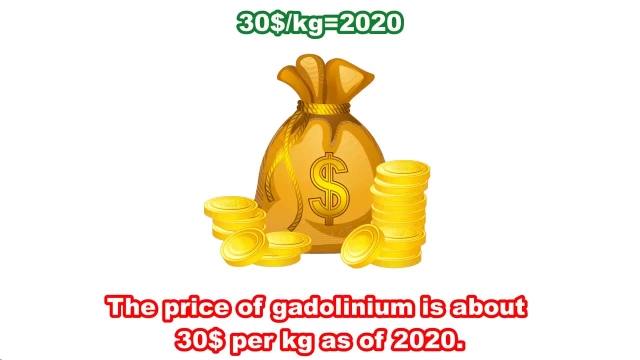 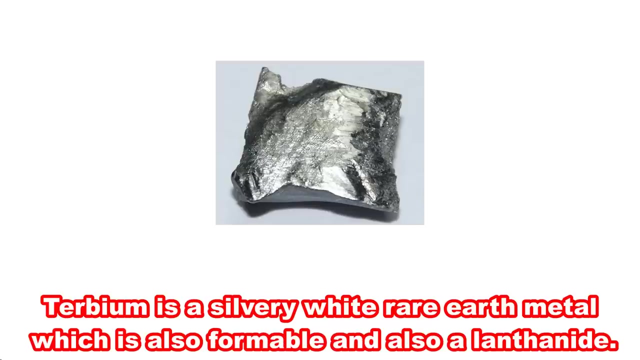 lanthanide. gadolinium is used in magnetic resonance imaging, particularly in diagnosing cancerous tumors. the most common gadolinium atomic structure is 64 protons, 93 neutrons and 64 electrons. the price of gadolinium is about $30 per kilogram of of 2020 number 65 terbium. terbium is a silvery white. 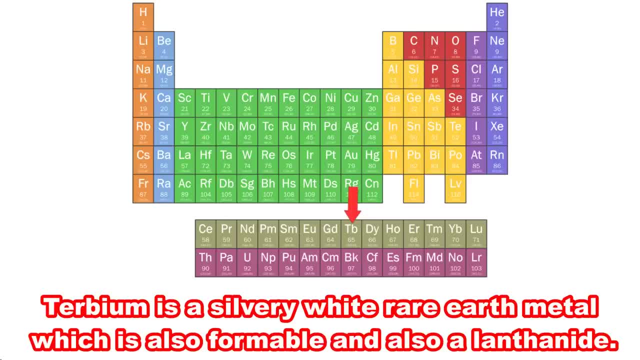 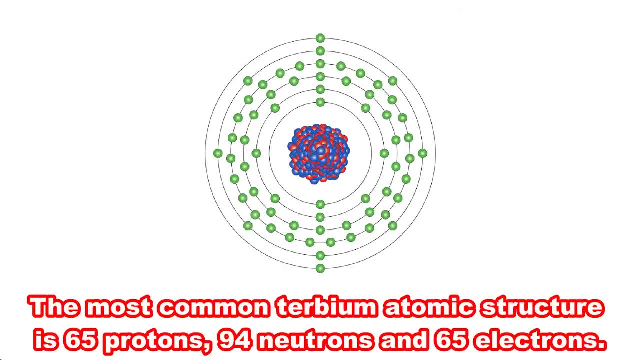 rare-earth metal which is also formable, and also a lanthanide terbium is used to dope calcium fluoride, calcium tungstate and strontium. mu libertate of the structure is 65 protons級 Turbium. atomic structure is 65 protons, 94 neutrons and 65 electrons. 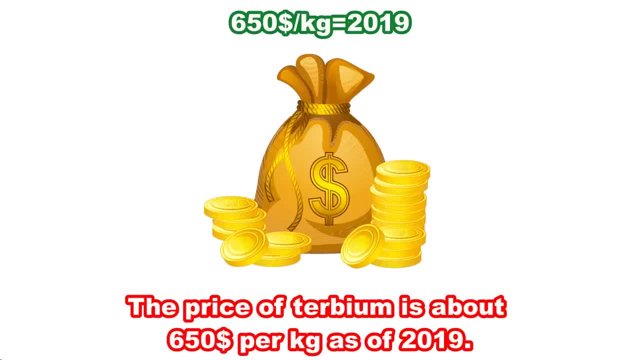 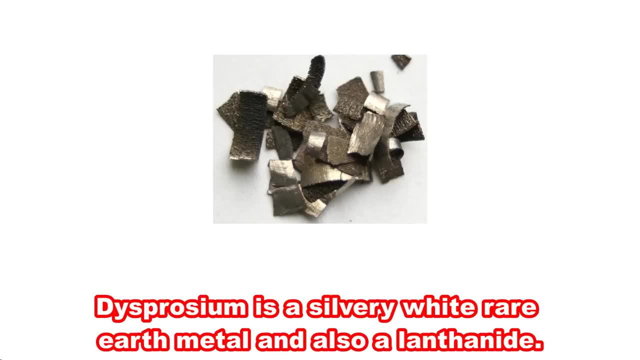 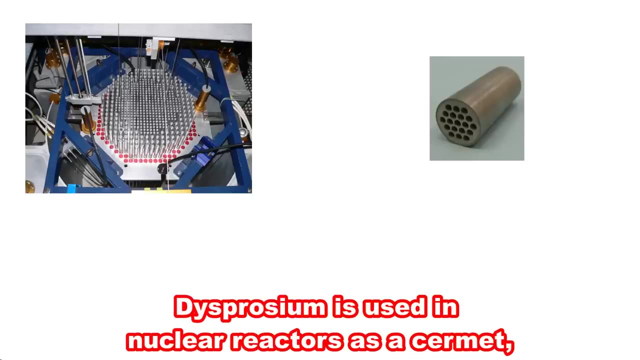 The price of Turbium is about $ 650 per kg as of 2019.. Number 66.. Dysprosium. Dysprosium is a silvery, white rare earth metal and also a lanthanide. Dysprosium is used in nuclear reactors as a Cermet, a composite material made of ceramic. 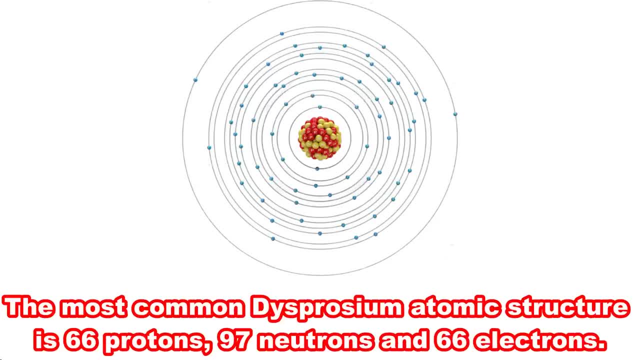 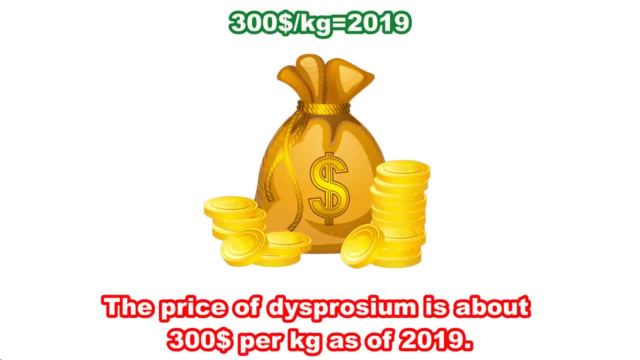 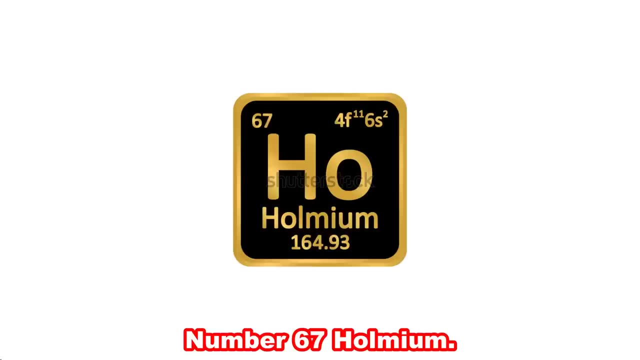 and sintered metal. The most common Dysprosium atomic structure is 66 protons, 97 neutrons and 66 electrons. The price of Dysprosium is about $ 300 per kg as of 2019.. Number 67.. 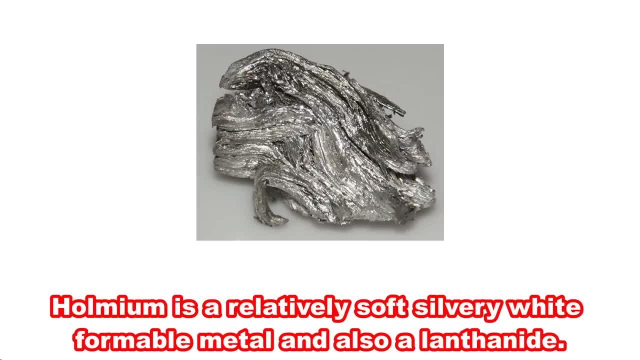 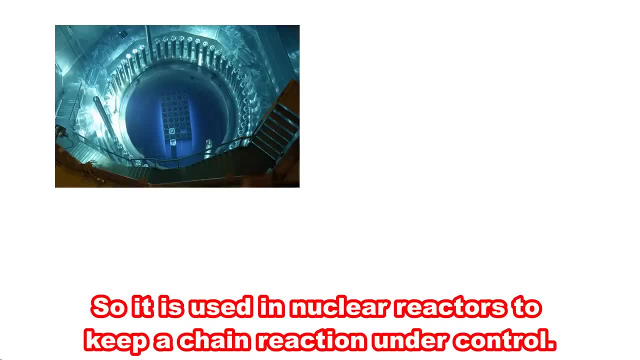 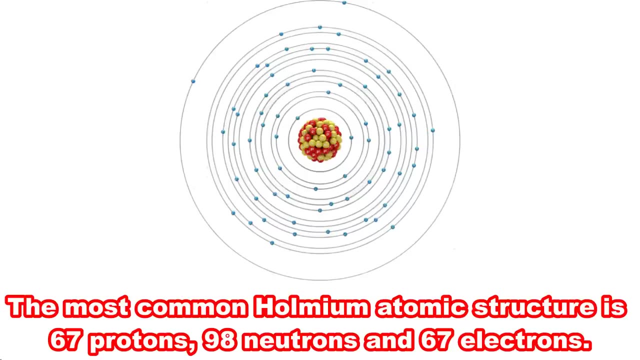 Holmium. Holmium is a relatively soft, silvery, white, formable metal and also a lanthanide. Holmium can absorb neutrons, so it is used in nuclear reactors to keep a chain reaction under control. The most common Holmium atomic structure is 67 protons, 98 neutrons and 67 electrons. 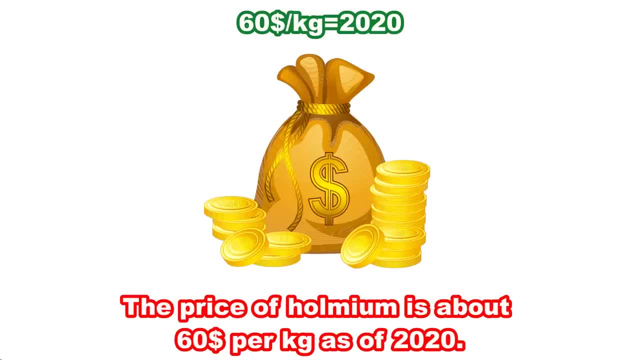 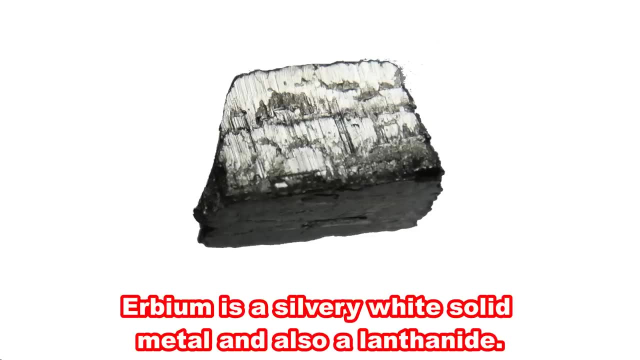 The price of Holmium is about $ 60 per kg as of 2020.. Number 68. Erbium. Erbium is a silvery, white solid metal and also a lanthanide. Erbium is used to color the lenses of glasses. 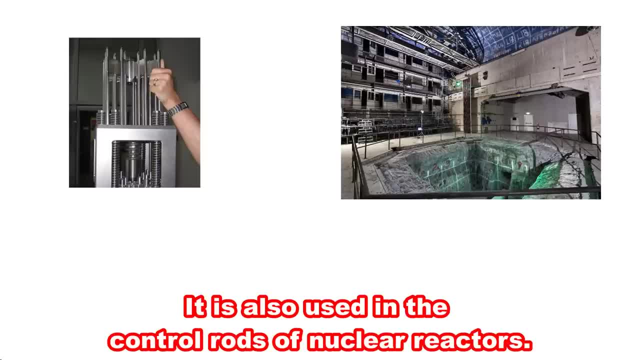 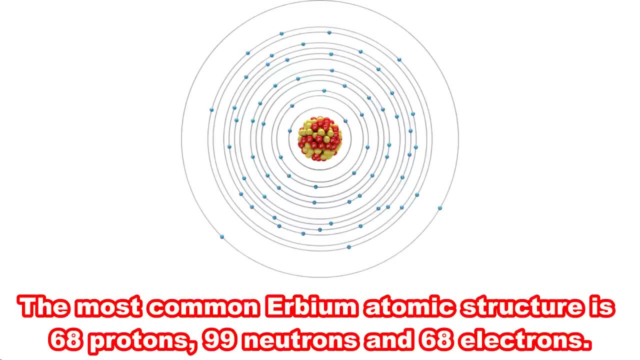 It is also used in the control rods of nuclear reactors. The most common Erbium atomic structure is Dysprosium. Holmium atomic structure is 68 protons, 99 neutrons and 68 electrons. The price of Erbium is about $ 26 per kg as of 2020.. 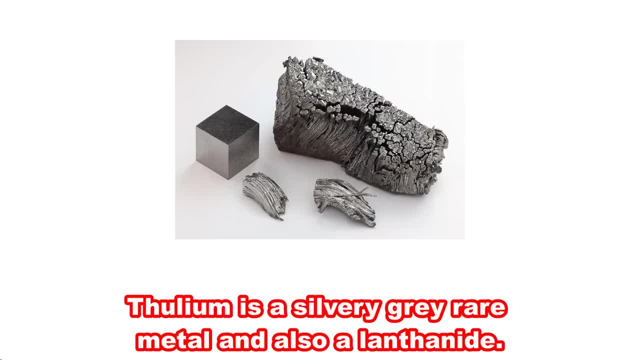 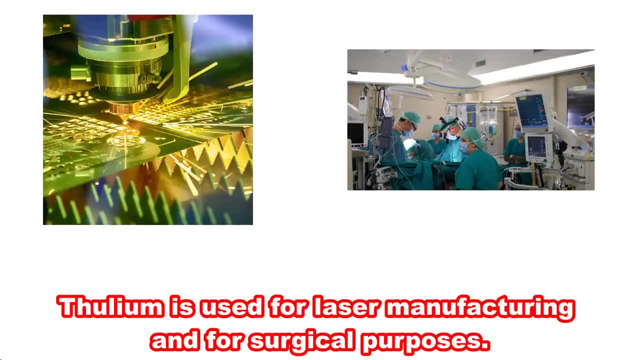 Number 69. Thulium. Thulium is a silvery gray rare metal and also a lanthanide. Thulium is used for laser manufacturing and for surgical purposes. The most common Thulium atomic structure is 69 protons, 100 neutrons and 66 electrons. 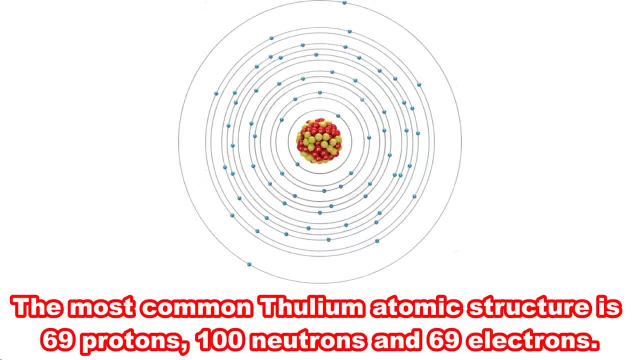 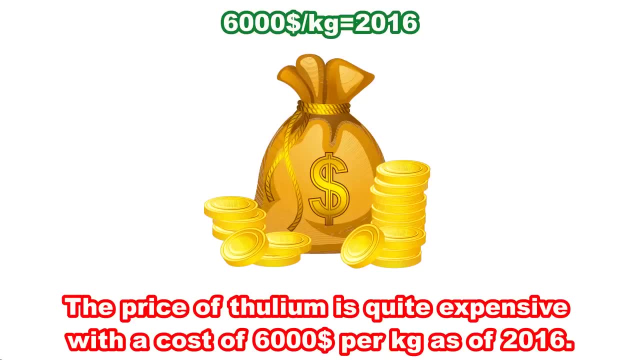 The most common Erbium atomic structure is Dysprosium. Holmium is a relatively soft, silvery, white, formable metal and also a lanthanide. The price of Thulium is quite expensive, with a cost of $ 6,000 per kg as of 2016.. 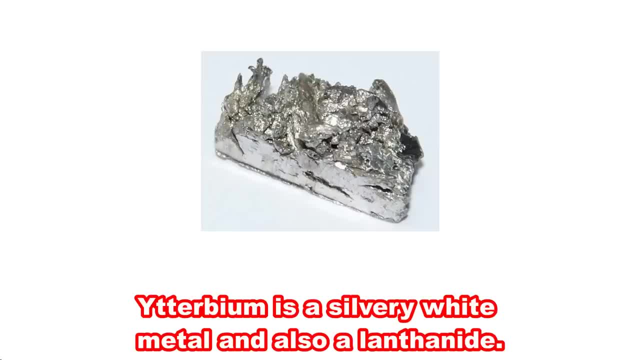 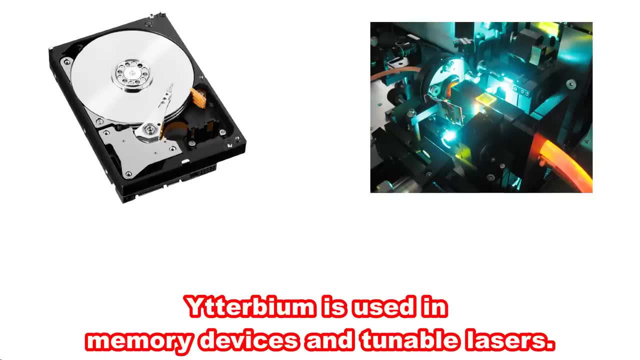 Number 70. Ytterbium. Ytterbium is a silvery white metal and also a lanthanide. Ytterbium is used in memory devices and tunable lasers. It can also be used as an industrial catalyst. 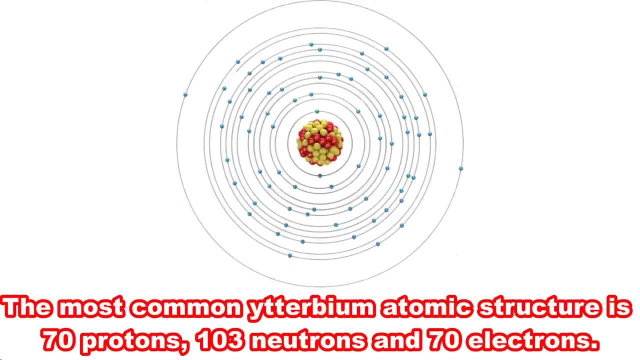 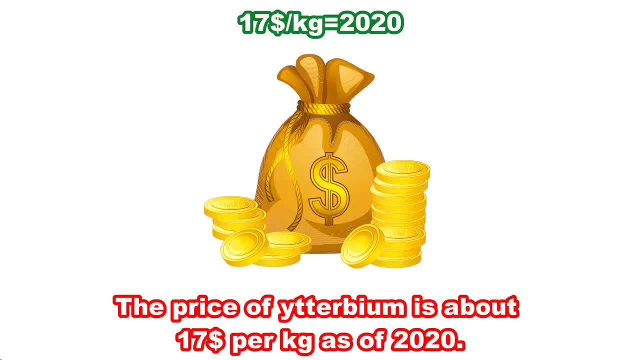 The most common Ytterbium atomic structure is 70 protons, 103 neutrons and 60 electrons. The price of Ytterbium is about $ 17 per kg as of 2020.. Number 71. Lutetium. 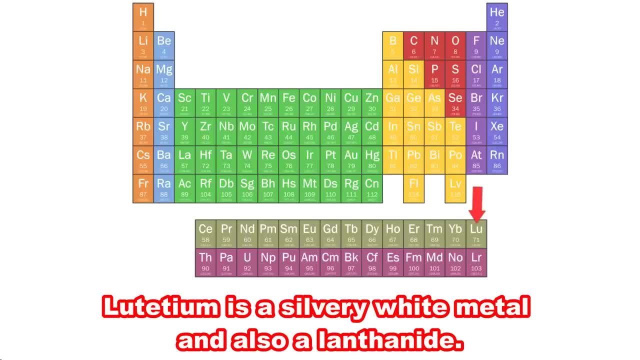 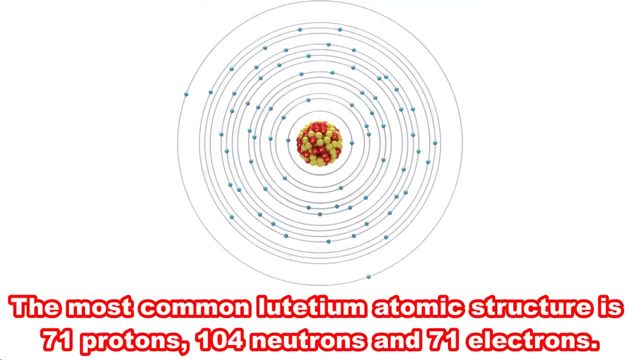 Lutetium is a silvery white metal and also a lanthanide. Lutetium is mostly used in research, but also in scintillators and X-ray Phosphors. The most common Lutetium atomic structure is 71 protons, 104 neutrons and 71 electrons. 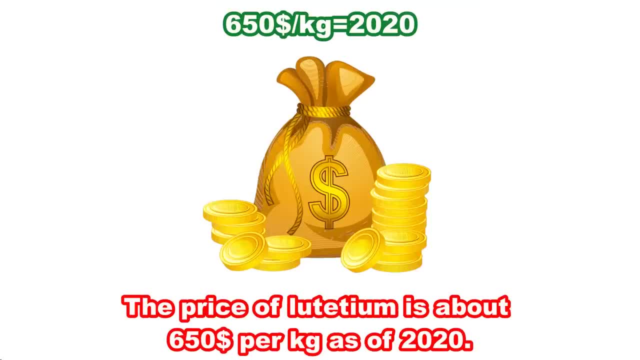 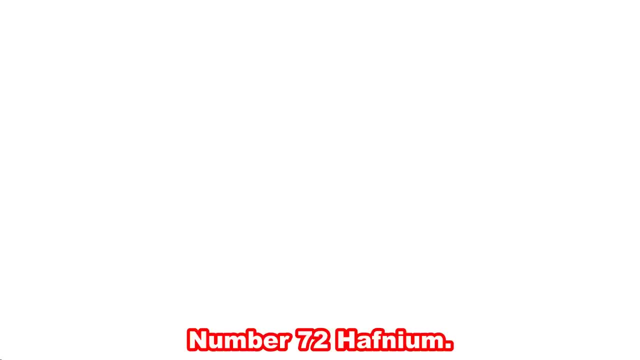 The price of Lutetium is about $ 10 per kg as of 2020.. Number 71. Lutetium. Lutetium is about $650 per kilogram as of 2020.. Number 72. Hafnium. 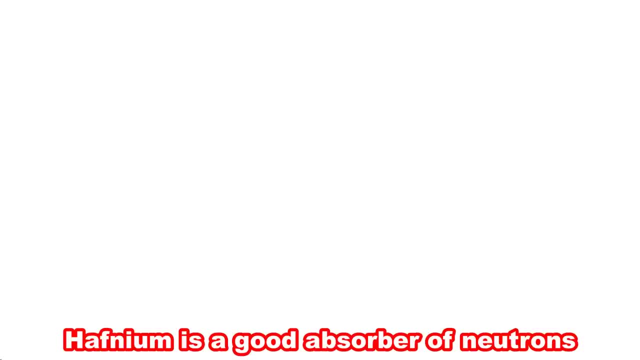 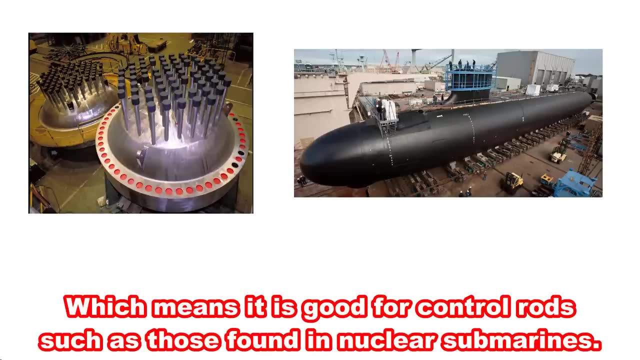 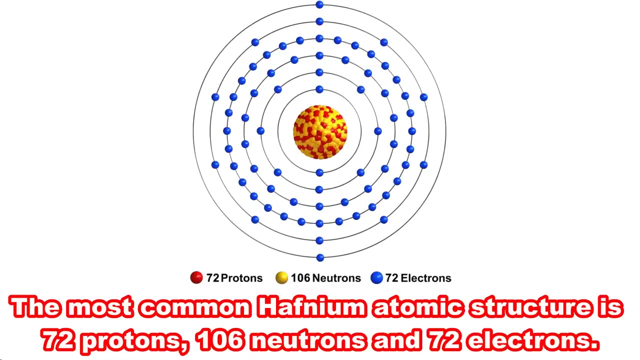 Hafnium is a shiny, silvery, gray transition metal. Hafnium is a good absorber of neutrons, which means it is good for control rods such as those found in nuclear submarines. The most common Hafnium atomic structure is 72 protons, 106 neutrons and 72 electrons. 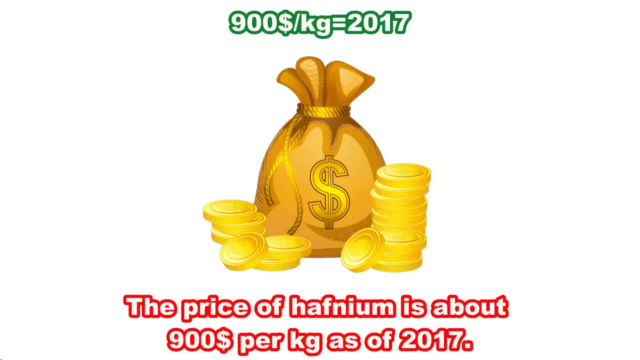 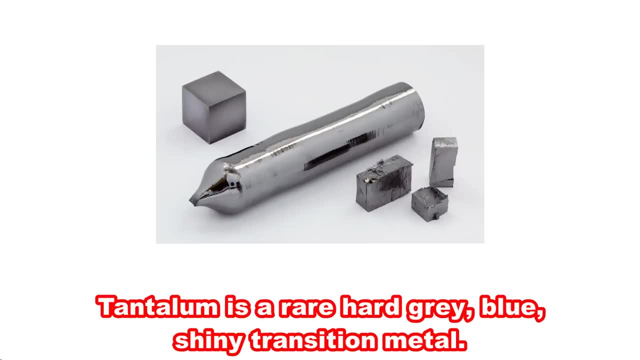 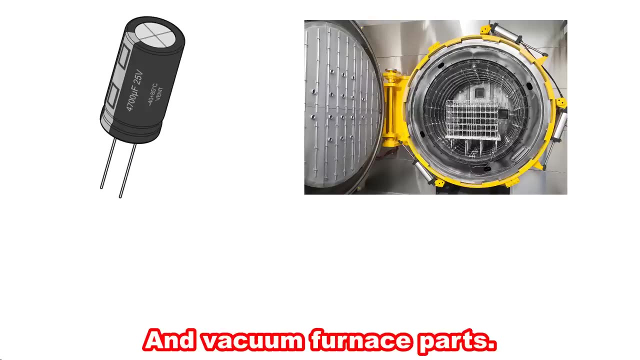 The price of Hafnium is about $900 per kilogram as of 2017.. Number 73. Tantalum. Tantalum is a rare hard gray, blue, shiny transition metal. More than half of Tantalum's use is for electrolytic capacitors and vacuum furnace parts. 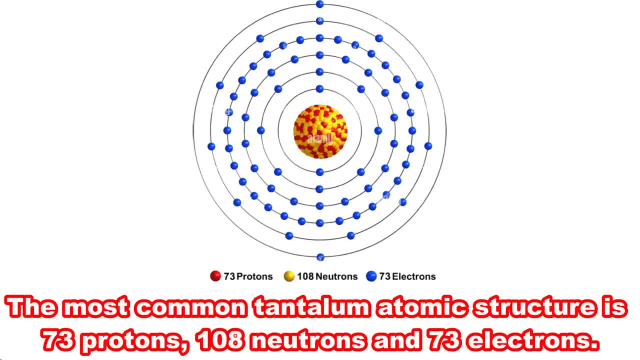 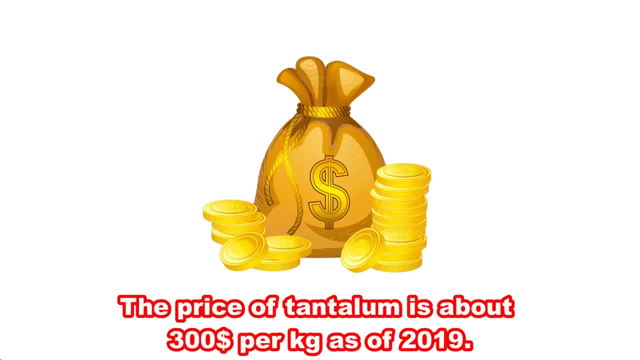 The most common Tantalum atomic structure is 73 protons, 108 neutrons and 73 electrons. The price of Tantalum is about $300 per kilogram. The most common Tantalum atomic structure is about $100 per kilogram as of 2019.. 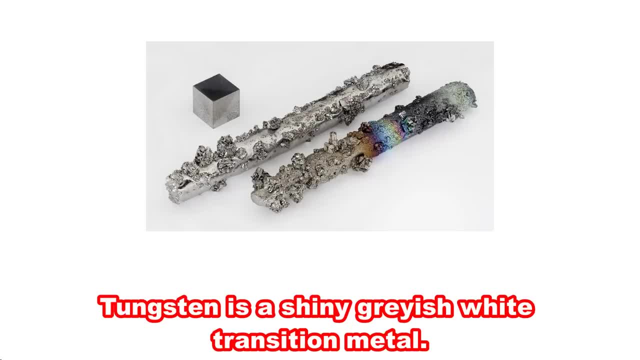 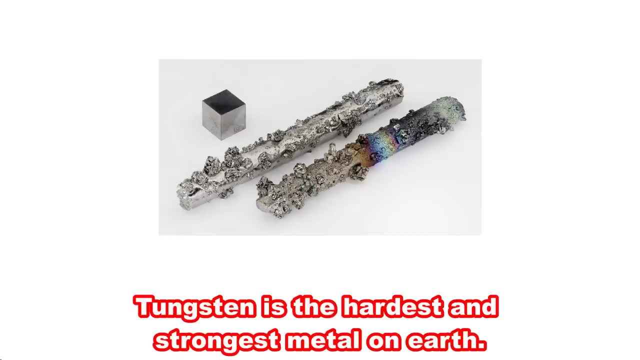 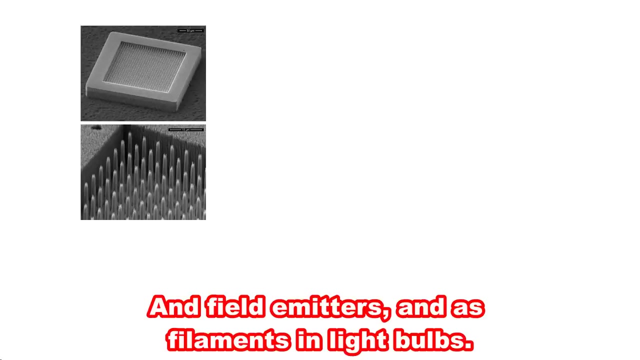 Number 74.. Tungsten. Tungsten is a shiny, grayish, white transition metal. It has the highest melting and boiling point of all elements. Tungsten is the hardest and strongest metal on earth. Tungsten is used for electrodes, heating elements and field emitters and as filaments in light. 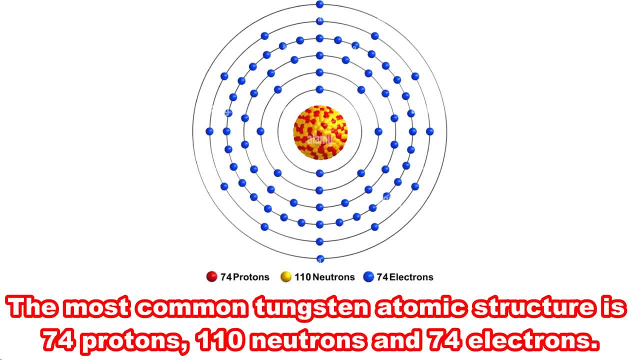 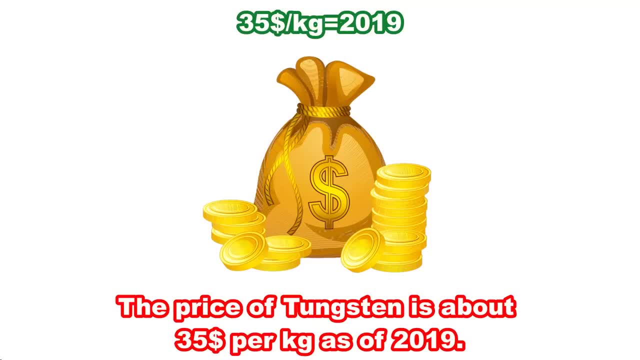 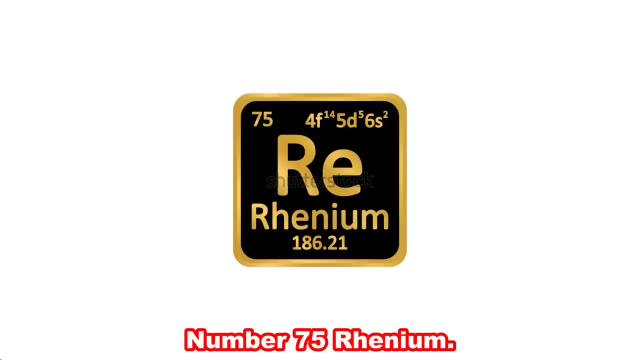 bulbs. The most common Tungsten atomic structure is 74 protons, 110 neutrons and 70 electrons. The price of Tungsten is about $35 per kilogram as of 2019.. Number 75. Rhenium. 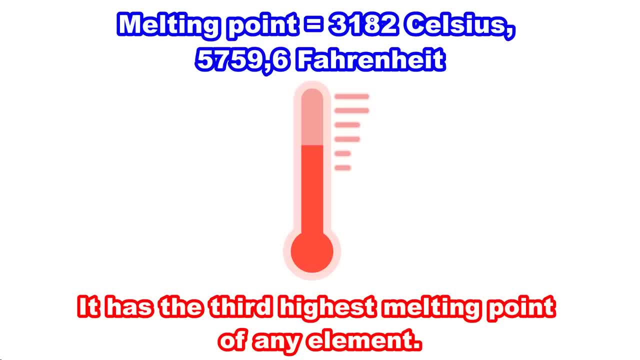 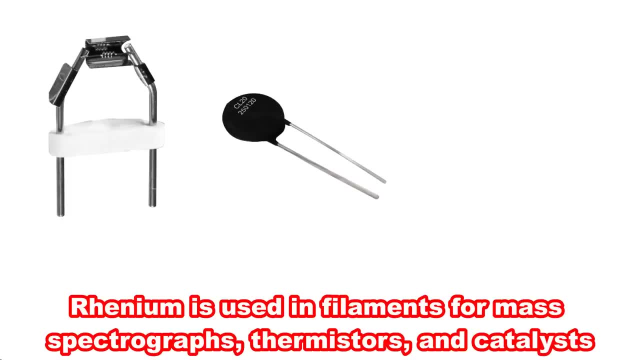 Rhenium is a silvery gray heavy transition metal. It has the third highest melting point of any element. Rhenium is used in filaments for mass spectrographs, thermistors and catalysts and as an additive to tungsten and molybdenum-based alloys. 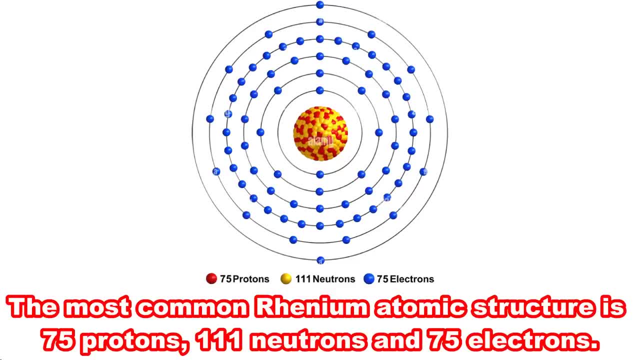 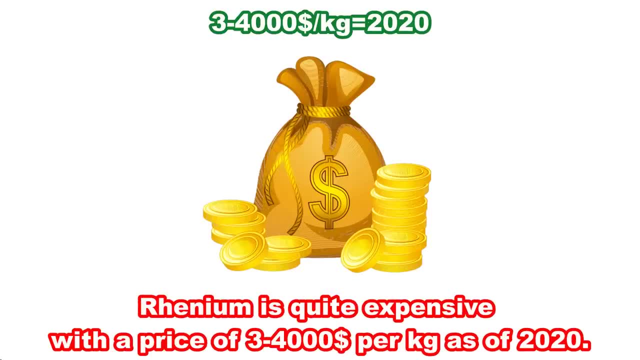 The most common Rhenium atomic structure is 75 protons, 108 neutrons and 74 electrons. Rhenium is quite expensive, with a price of $3,000 to $4,000 per kilogram as of 2020.. 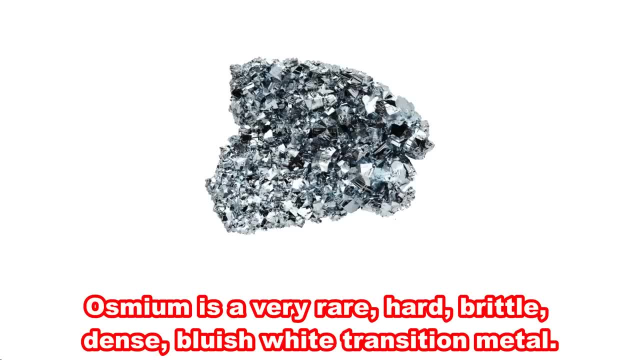 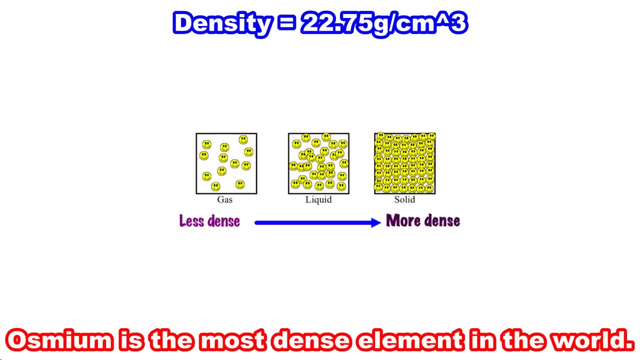 Number 76.. Osmium. Osmium is a very rare, hard brittle, dense, bluish, white transition metal. Osmium is the most dense element in the world. It is used to produce very hard alloys for fountain pens. 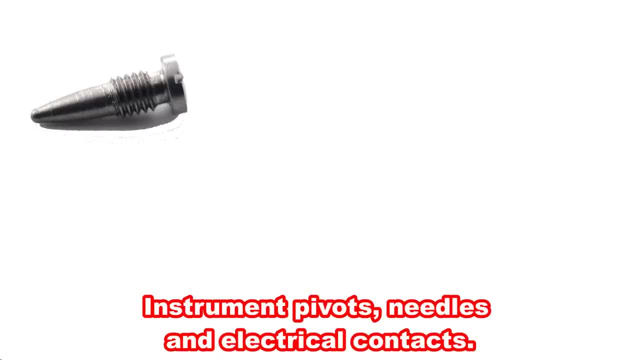 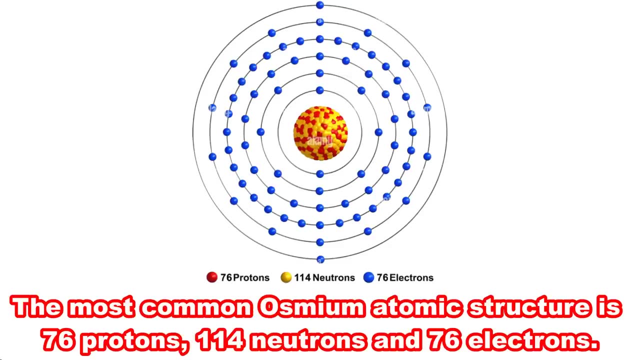 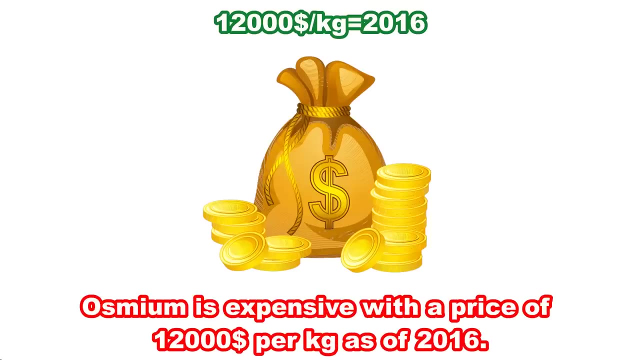 It has the highest melting point on earth. It is used for fountain pen, tips, instrument pivots, needles and electrical contacts. The most common Osmium atomic structure is 76 protons, 114 neutrons and 76 electrons. Osmium is expensive, with a price of $12,000 per kilogram as of 2016.. 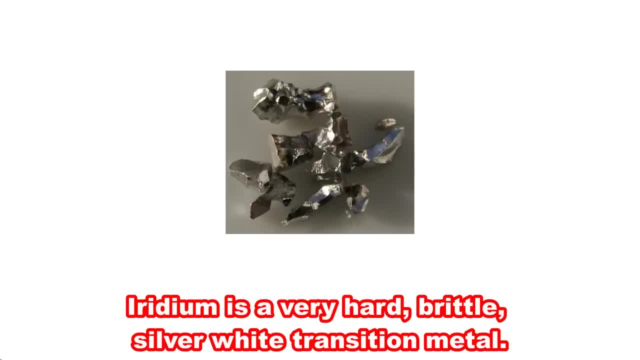 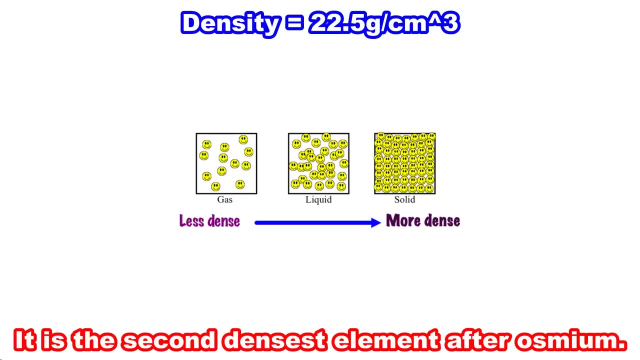 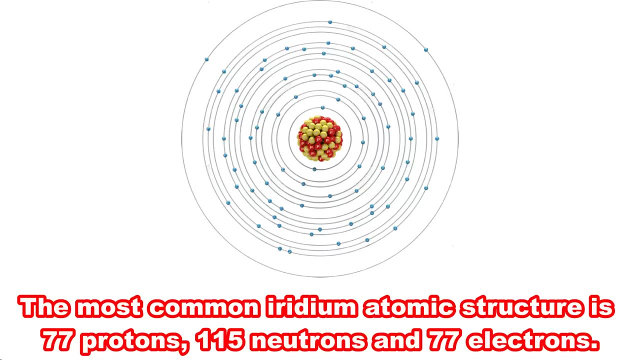 Number 77. Iridium. Iridium is a very hard, brittle silver white transition metal. It is the second densest element after Osmium. Iridium's primary use is a hardening agent for platinum. The most common Iridium atomic structure is 77 protons, 115 neutrons and 77 electrons. 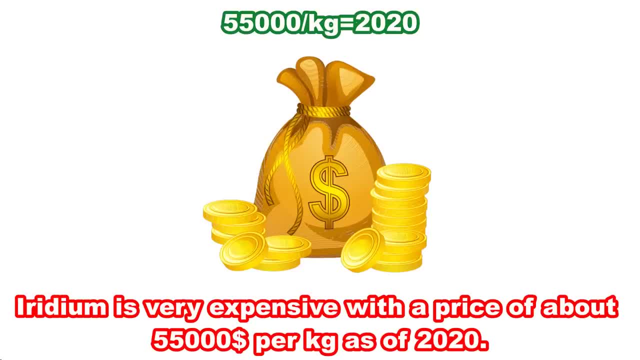 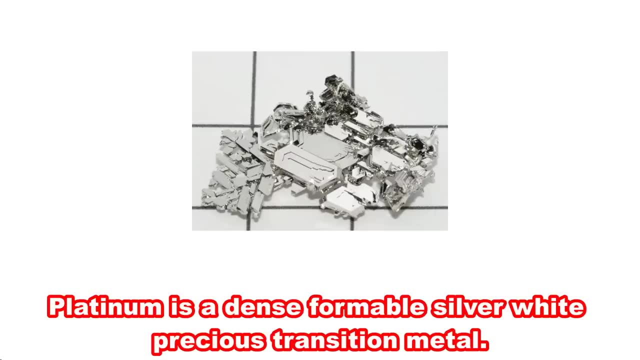 Iridium is very expensive, with a price of about $55,000 per kilogram as of 2020.. Number 78. Platinum. Platinum is a dense, formable silver- white precious transition metal. It is the second densest element after osmium. 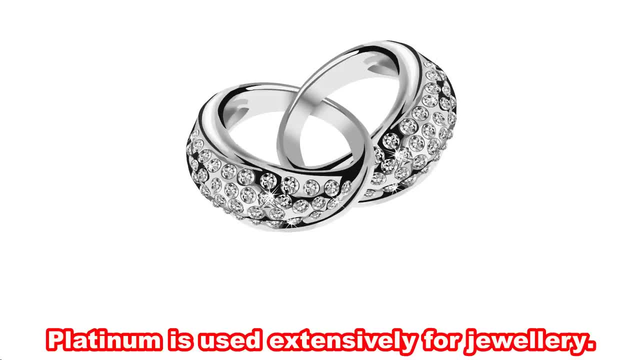 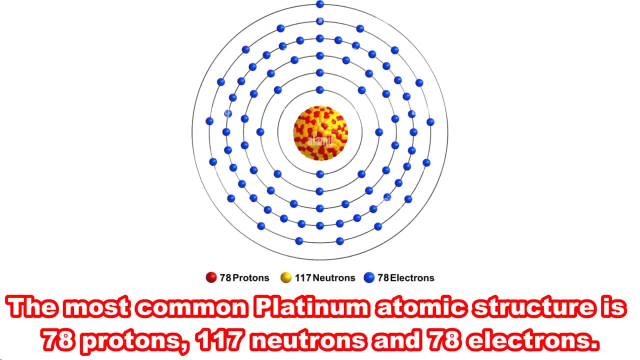 Iridium's primary use is a hardening agent. for platinum, It is the second densest element after osmium. Platinum is used extensively for jewelry. Its main use, however, is in catalytic converters for cars, trucks and buses. The most common platinum atomic structure is 78 protons, 117 neutrons and 78 electrons. 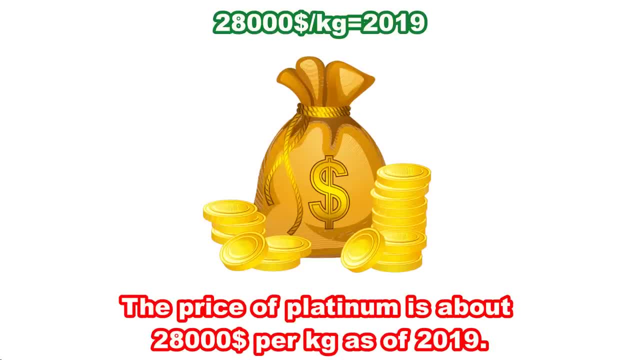 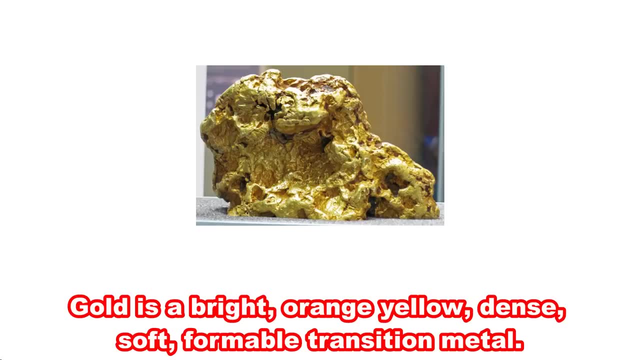 The price of platinum is about $28,000 per kilogram as of 2019.. Number 79. Gold Gold. Gold is a bright orange, yellow, dense, soft, silky, silver, white transition metal. It is the second densest element after osmium. 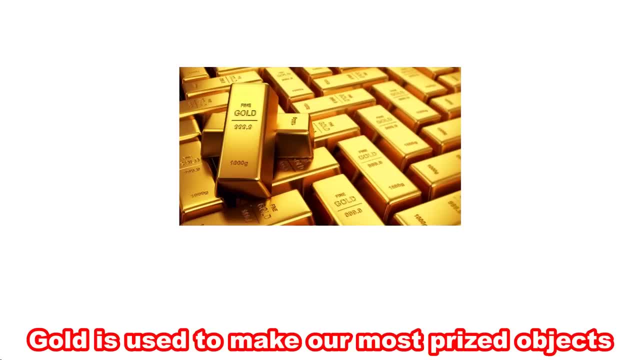 This is a common point on metal sources such as stocks, edessa, AOE, Chia-Iberiaавлив Gold, reef, Scarfiños. The Gold is used to make our most prized objects: wedding rings, Olympic medals, money, jewelry. 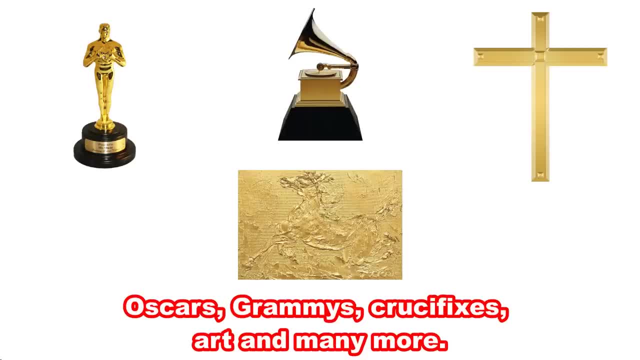 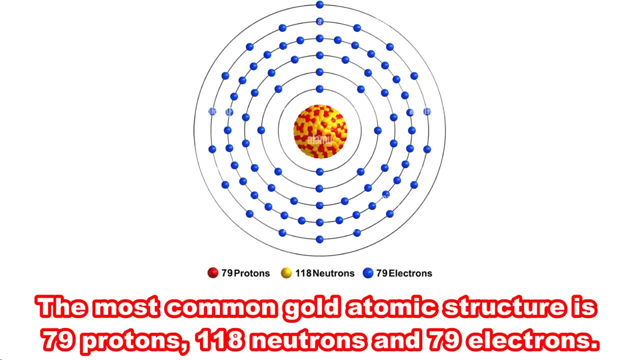 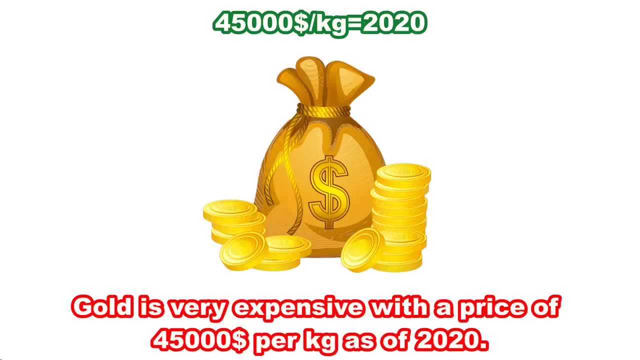 Oscars, Grammy's, crucifixes, art and many more. The most common gold atomic structure is 79 protons, 118 neutrons and 79 electrons. Gold is very expensive, with a price of about $45,000 per kilogram as of 2020.. 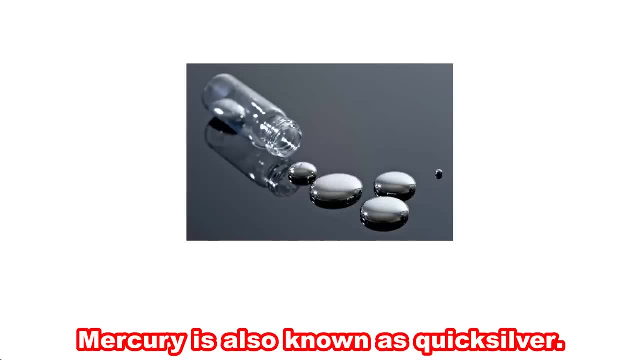 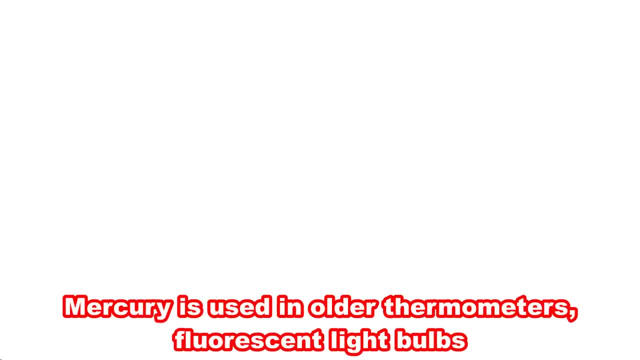 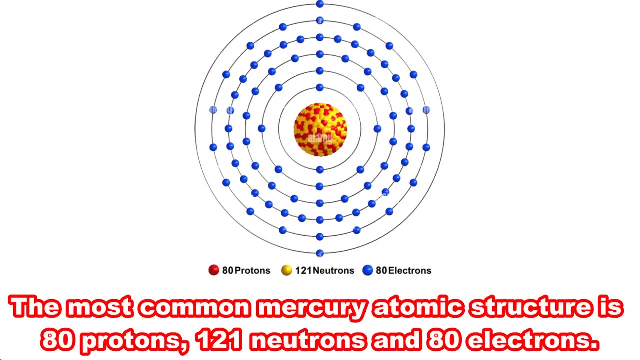 Number 80. Mercury. Mercury is also known as quicksilver. It is a shiny silver liquid and also a transition metal. Mercury is used in older thermometers, fluorescent light bulbs and some electrical switches. The most common mercury atomic structure is 80 protons, 121 neutrons and 80 electrons. 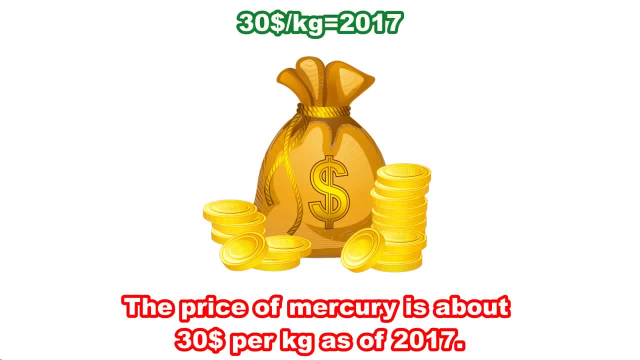 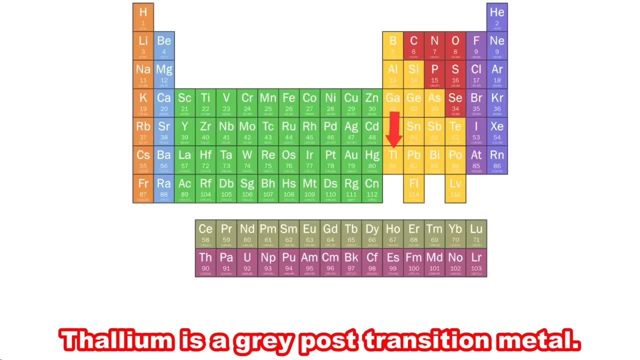 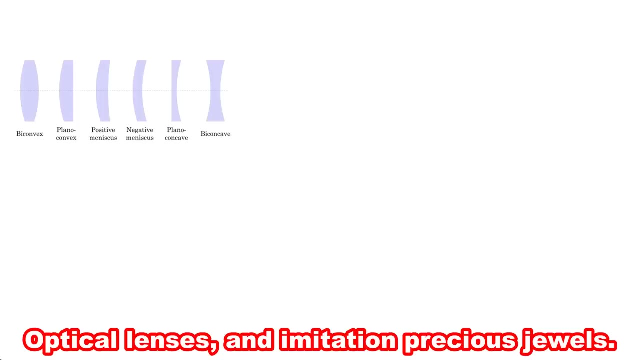 The price of mercury is about $30 per kilogram as of 2017.. Number 81. Thallium. Thallium is a great post transition metal. Thallium is used for manufacture of electronics, low temperature thermometers, optical lenses. 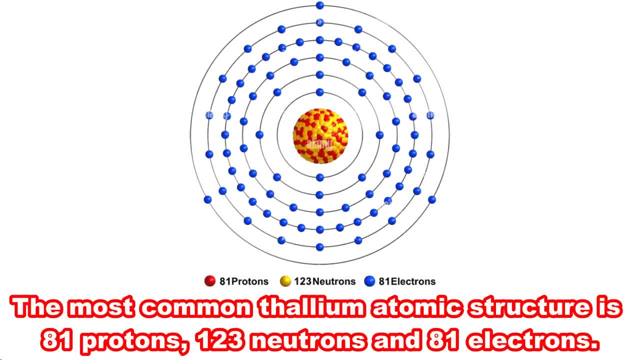 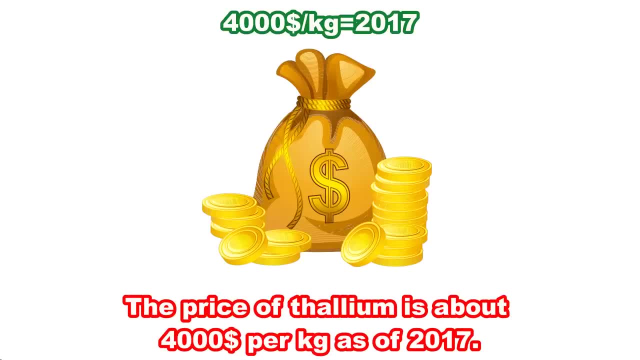 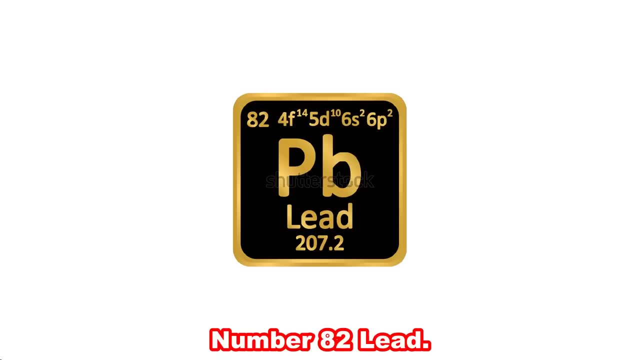 and imitation precious jewels. The most common thallium atomic structure is 81 protons, 123 neutrons and 81 electrons. The price of thallium is about $4000 per kilogram as of 2017.. Number 82.. 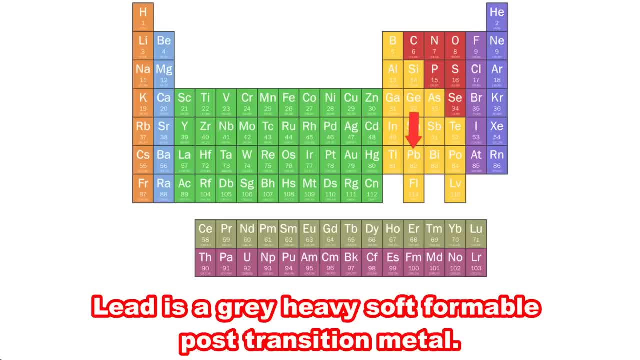 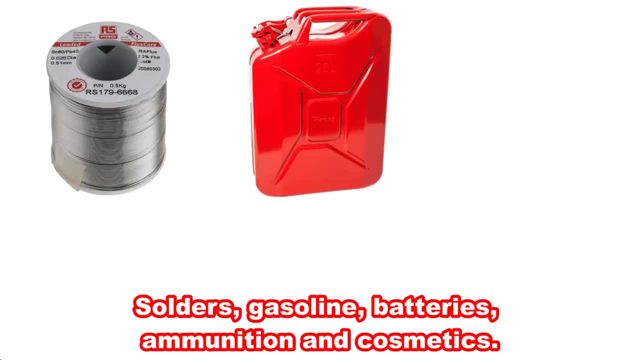 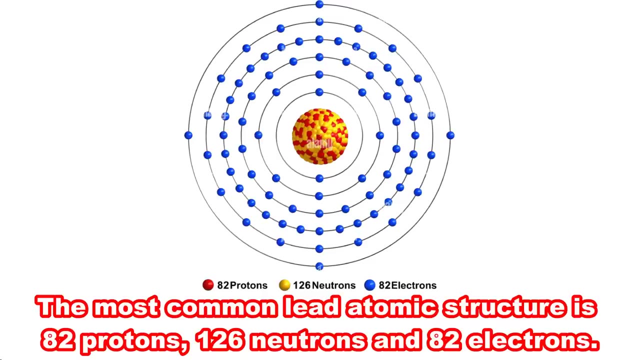 Lead. Lead is a gray, heavy, soft formable post transition metal. Lead is used for paint, ceramics, pipes and plumbing materials, solders, gasoline, batteries, ammunition and cosmetics. The most common lead atomic structure is 82 protons, 126 neutrons and 82 electrons. 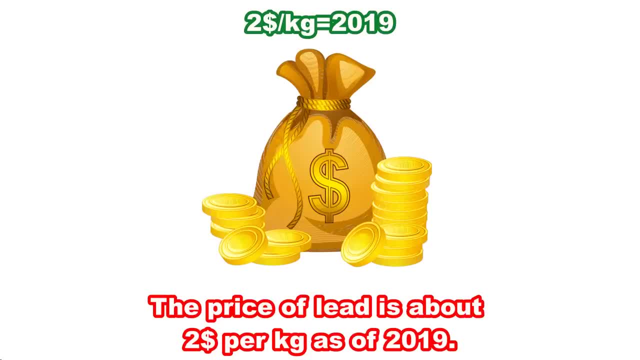 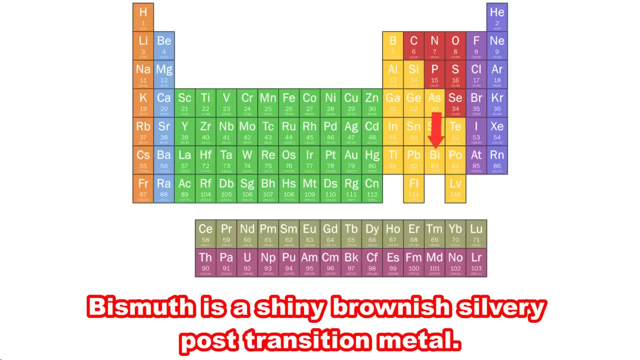 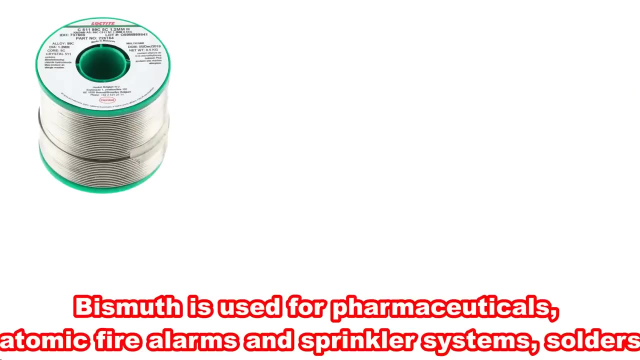 The price of lead is about $2 per kilogram as of 2019.. Number 83. Bismuth. Bismuth is a shiny brownish- silvery post transition metal. Bismuth is used for pharmaceuticals, atomic fire alarms and sprinkler systems solders. 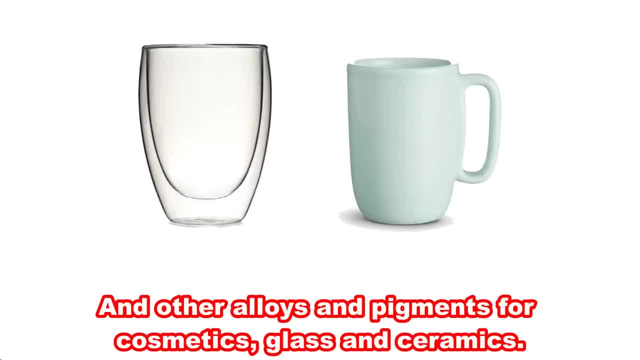 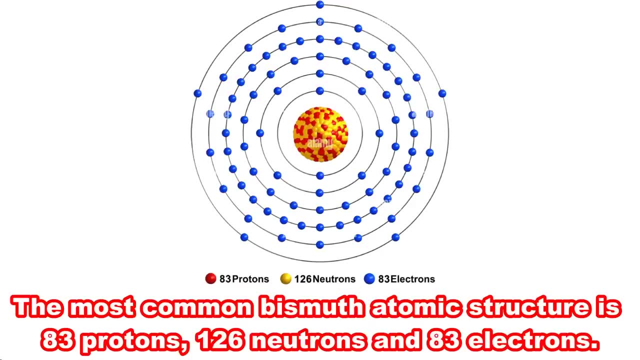 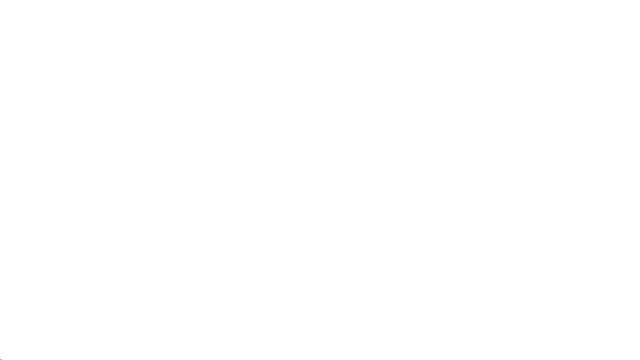 and other alloys and pigments for cosmetics, glass and ceramics. The most common bismuth atomic structure is 83 protons, 126 neutrons and 83 electrons. The price of bismuth is about $6 per kilogram as of 2019.. 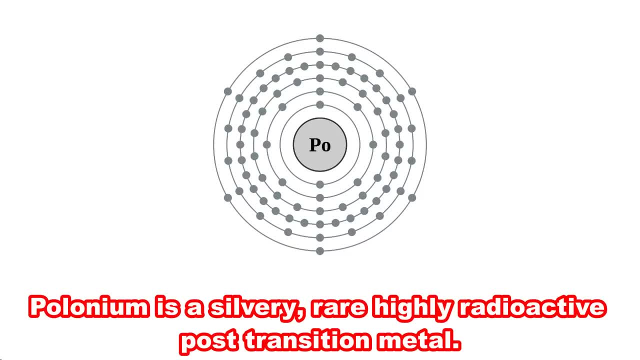 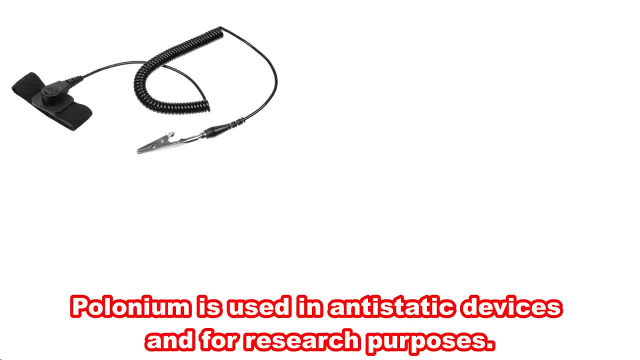 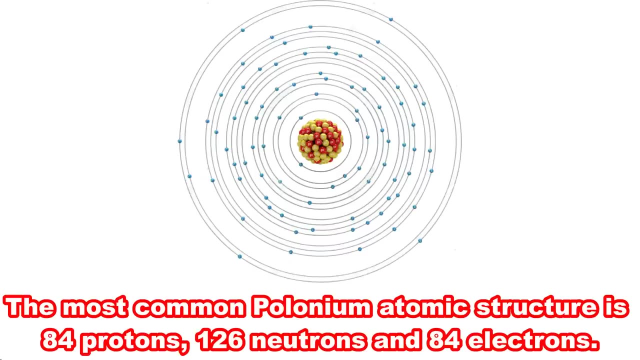 Number 84.. Polonium. Polonium is a silvery, rare, highly radioactive post transition metal. Polonium is used in anti-static devices and for research purposes. The most common polonium atomic structure is 84 protons, 126 neutrons and 84 electrons. 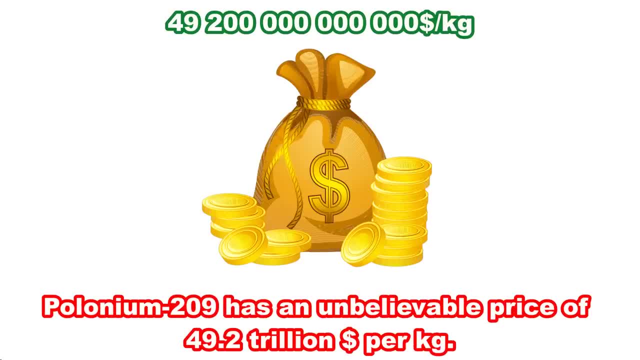 Polonium 209 has an unbelievable price of $49.2 trillion per kilogram, But the price of polonium 210 is about $10 per kilogram. The most common bismuth atomic structure is 84 protons, 126 neutrons and 84 electrons. 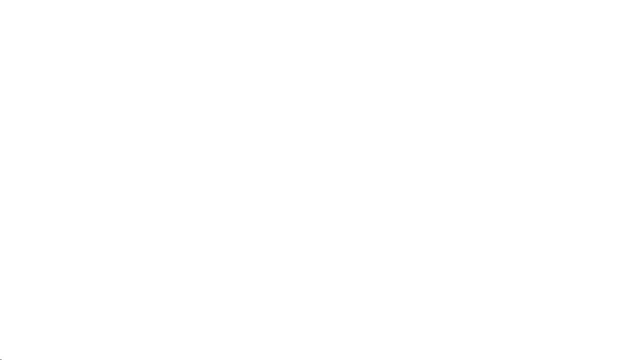 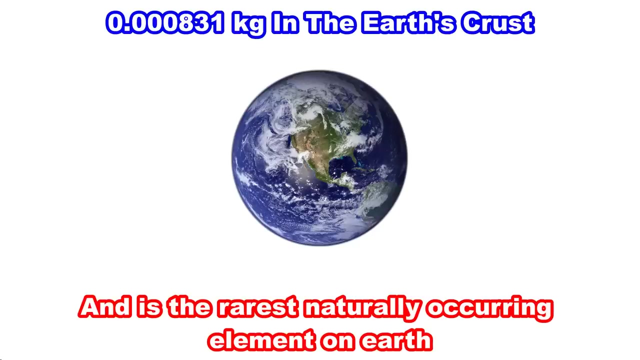 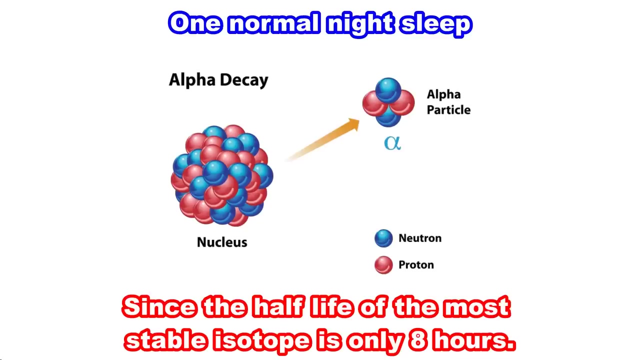 Polonium 210 is about $80,000 per kilogram. Number 85.. Astatine: Astatine is a halogen that has an unknown appearance and is the rarest naturally occurring element on earth. There are no other uses for astatine except research, since the half-life of the most stable. 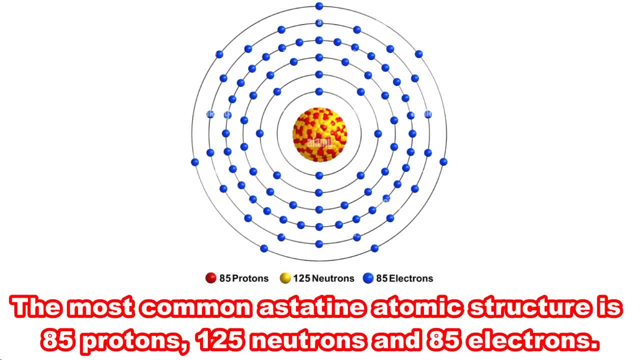 isotope is only 8 hours. The most common astatine atomic structure is 85 protons, 125 neutrons and 85 electrons. There is no other use for astatine except research, since the half-life of the most stable isotope. 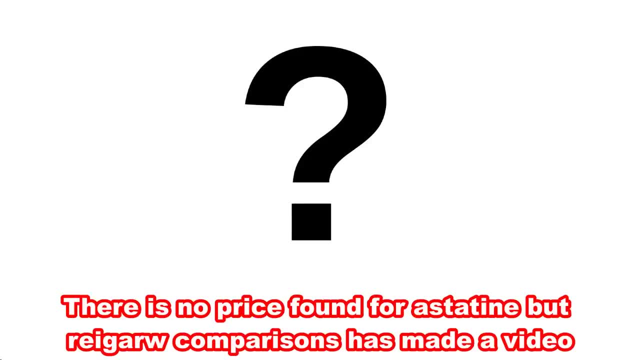 is only 8 hours. The most common astatine atomic structure is 85 protons, 125 neutrons and 85 electrons. There is no price found for astatine, but Rehgar Comparisons has made a video about the estimated. 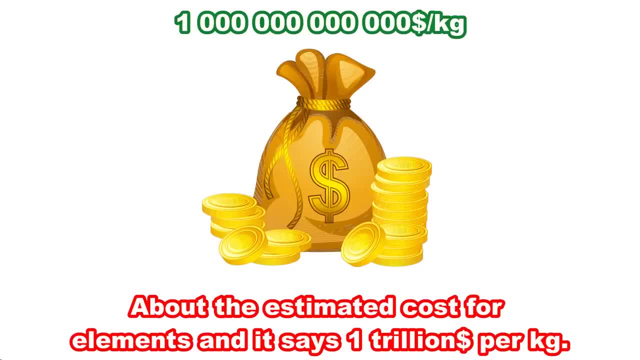 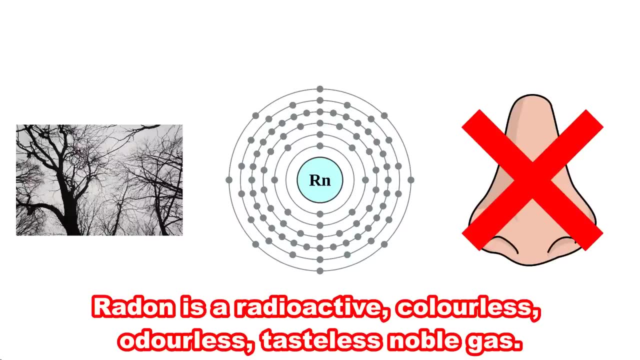 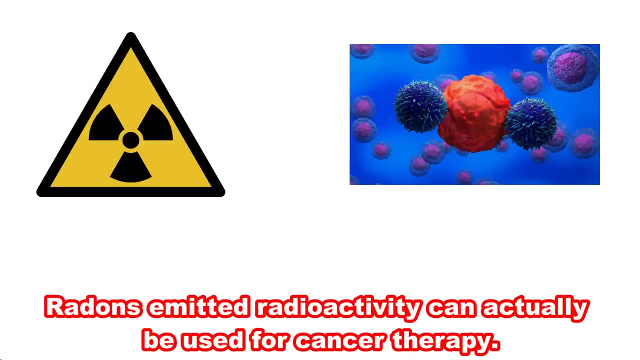 cost for elements and it says $1 trillion per kilogram. Number 86.. Radon. Radon is a radioactive, colorless, odorless, tasteless, noble gas. Radon's emitted radioactivity can actually be used for cancer therapy. 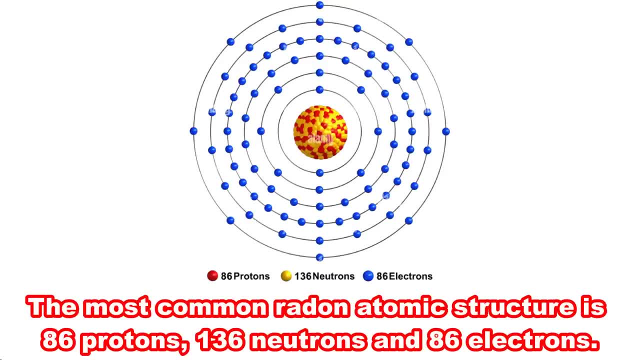 The most common radon atomic structure is 86 protons, 136 neutrons and 86 electrons. The most common radon atomic structure is 86 protons, 136 neutrons and 86 electrons. The most common radon atomic structure is 86 protons, 136 neutrons and 86 electrons. 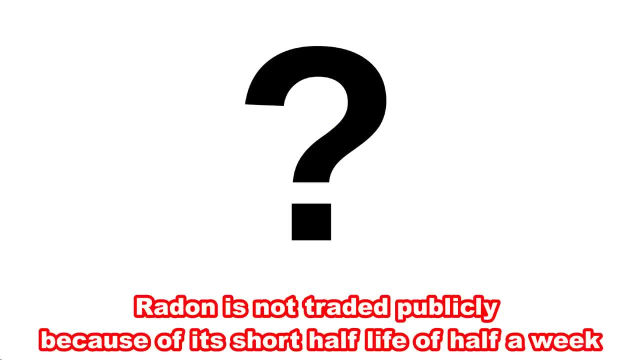 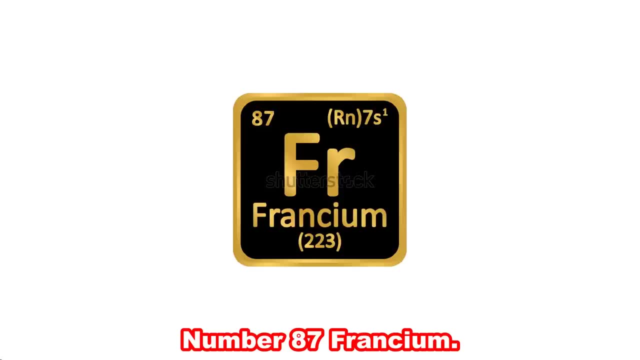 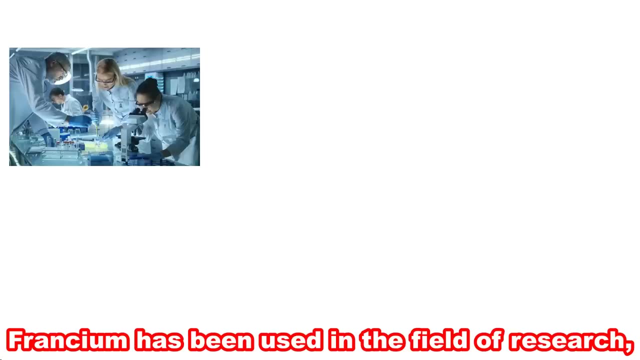 Radon is not traded publicly because of its short half-life of half a week, so I couldn't find a price for it. Number 87. Francium- Francium is a extremely radioactive alkali metal. Francium has been used in the field of research, chemistry and also in the atomic structure. 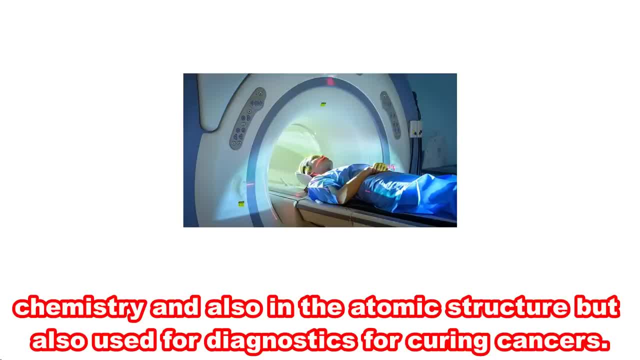 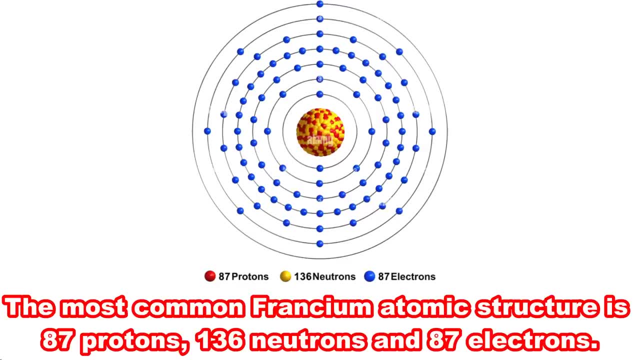 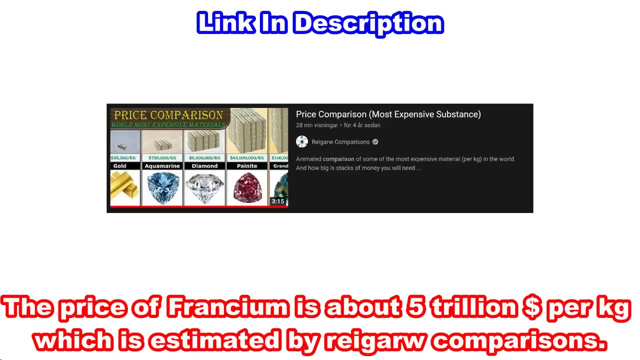 but also used for diagnostics for curing cancers. The most common francium atomic structure is 87 protons, 136 neutrons and 86 electrons- 136 neutrons and 87 electrons. The price of francium is about 5 trillion dollars per kilogram, which is estimated by 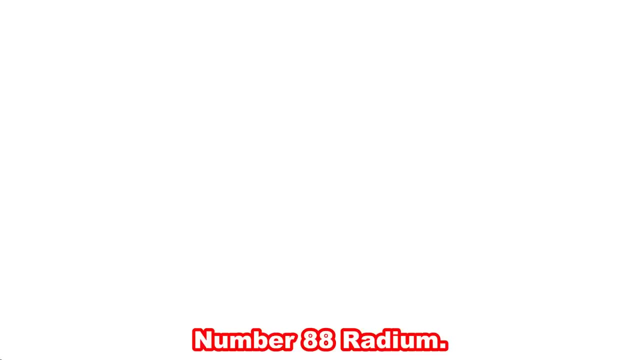 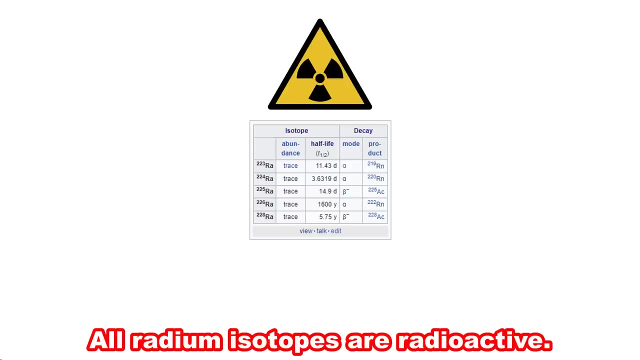 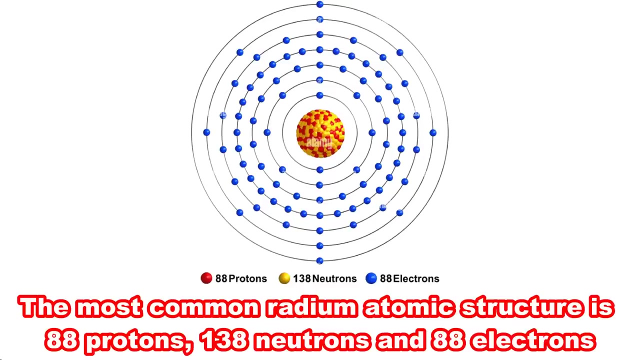 Rheogar comparisons, Number 88. Radium. Radium is a silvery, white, alkaline earth metal. All radium isotopes are radioactive. Radium is used in medicine to produce radon gas used for cancer treatment. The most common radium atomic structure is 88 protons, 138 neutrons and 88 electrons. 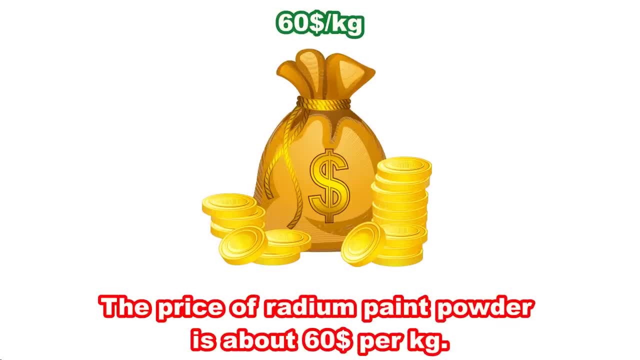 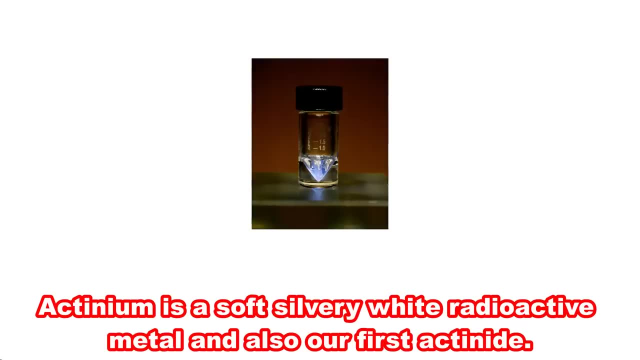 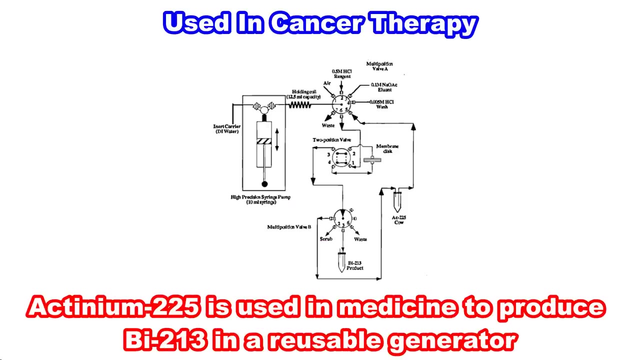 The price of radium paint powder is about 60 dollars per kilogram. Number 89. Actinium. Actinium is a soft, silvery, white radioactive metal and also our first actinide. Actinium 225 is used in medicine to produce by 213 in a reusable generator. 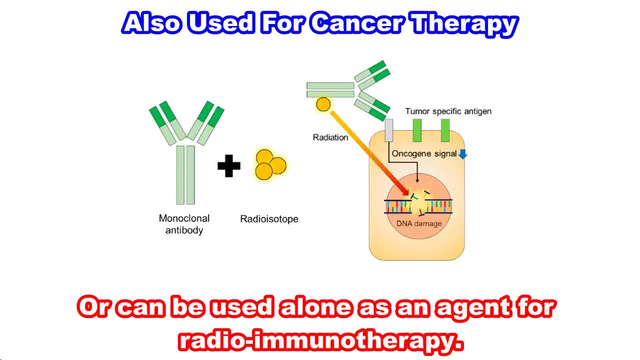 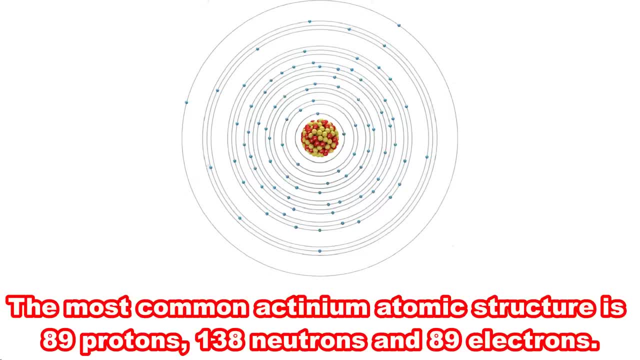 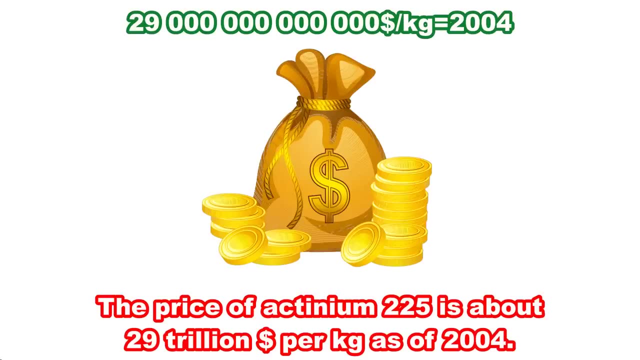 Or can be used alone as an agent for radio immunotherapy. The most common actinium atomic structure is 89 protons, 138 neutrons and 89 electrons. The price of actinium 225 is about 29 trillion dollars per kilogram as of 2004.. 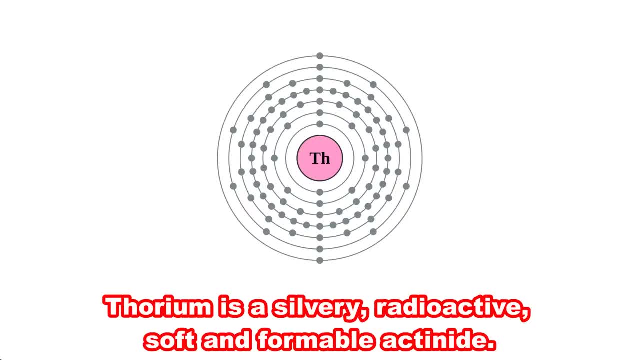 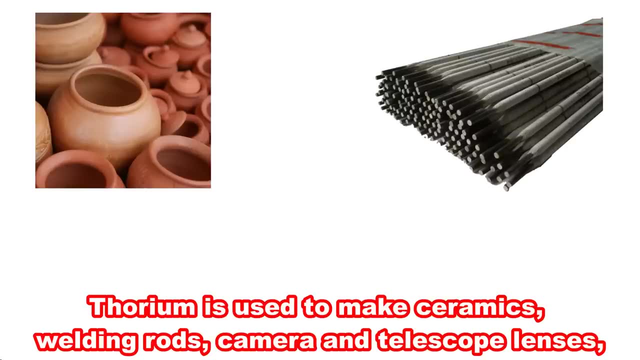 Number 90. Thorium. Thorium is a silvery, radioactive, soft and formable actinide. Thorium is used to make ceramics. Thorium is a silvery, radioactive, soft and formable actinide. Thorium is used to make ceramics, welding rods, camera and telescope lenses, fire brick. 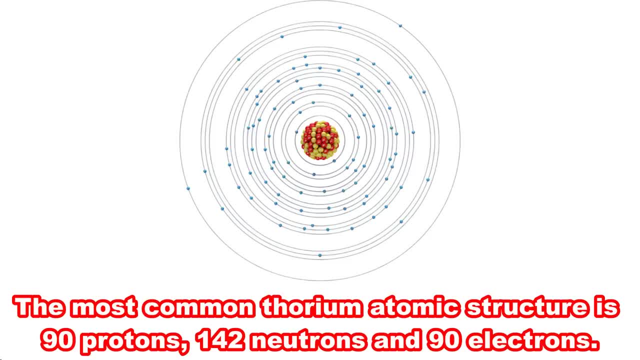 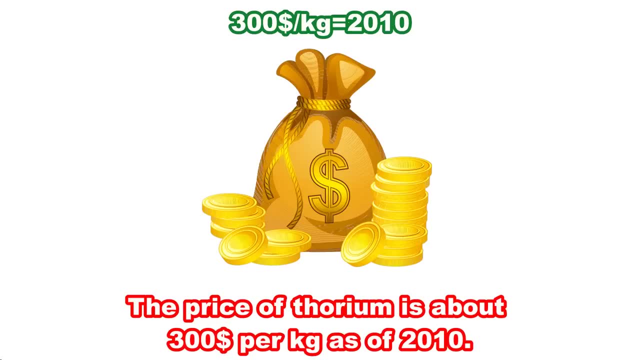 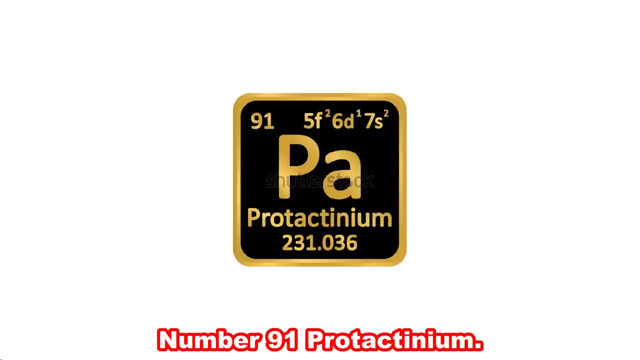 heat resistant paint and more. The most common thorium atomic structure is 90 protons, 142 neutrons and 90 electrons. The price of thorium is about 300 dollars per kilogram as of 2010.. Number 91.. 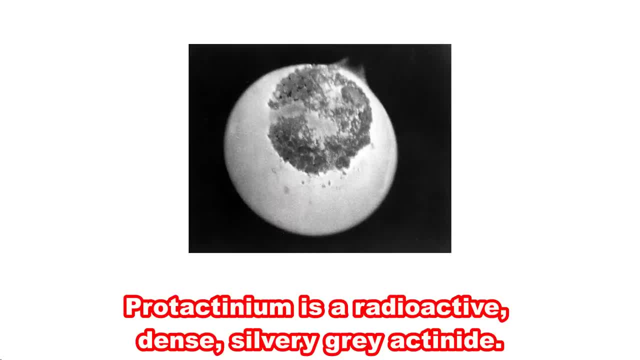 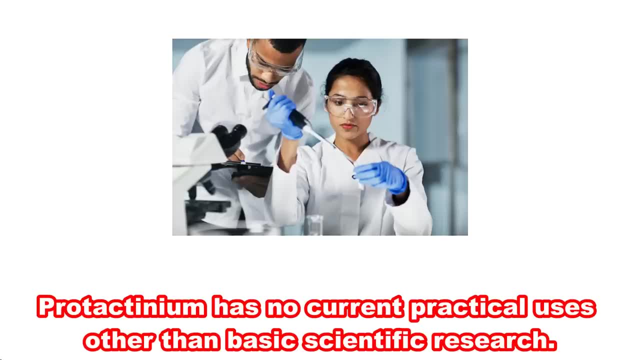 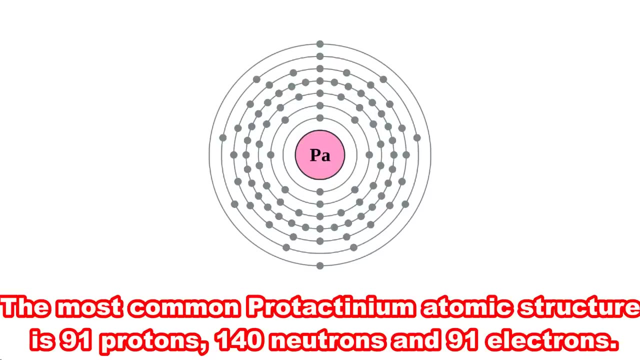 Protactinium. Protactinium is a radioactive dense silvery gray actinide. Protactinium has no current practical use. There are no current practical uses other than basic scientific research. The most common protactinium atomic structure is 91 protons, 140 neutrons and 91 electron. 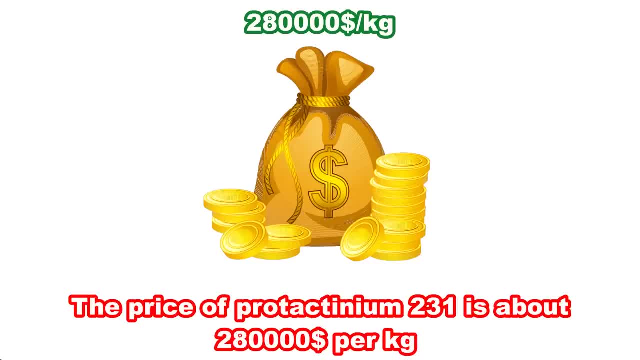 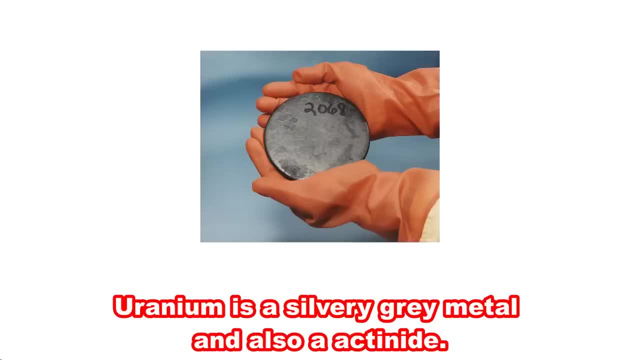 The price of protactinium 231 is about 280 thousand dollars per kilogram. Number 92. Uranium. Uranium is a silvery gray metal and also a actinide. Uranium is used to power commercial nuclear plants. Uranium is a silvery gray metal and also a actinide. 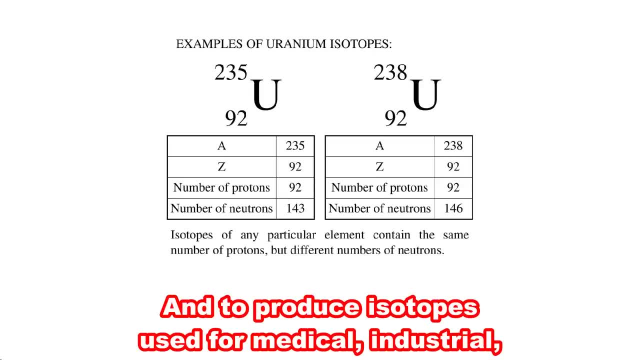 Uranium is used to power commercial nuclear plants. Uranium is used to make solar reactors that produce electricity and to produce isotopes used for medical, industrial and defense purposes around the world. Uranium is used to make solar reactors that produce electricity and to produce isotopes used for medical, industrial and defense purposes around the world. 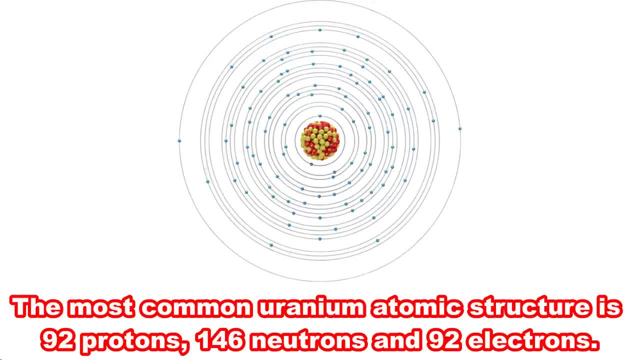 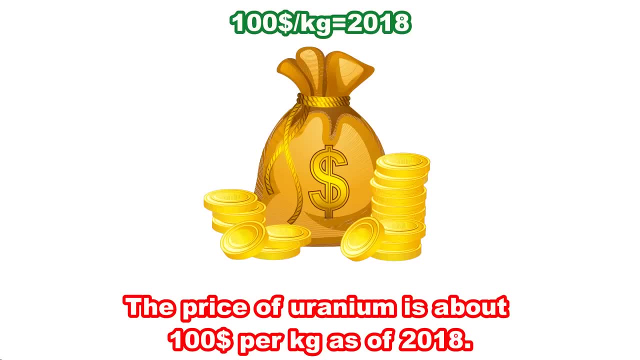 The most common uranium atomic structure is 92 protons, 146 neutrons and 92 electrons. The price of uranium is about 100 dollars per kilogram as of 2018.. The price of uranium is about 100 dollars per kilogram as of 2018.. 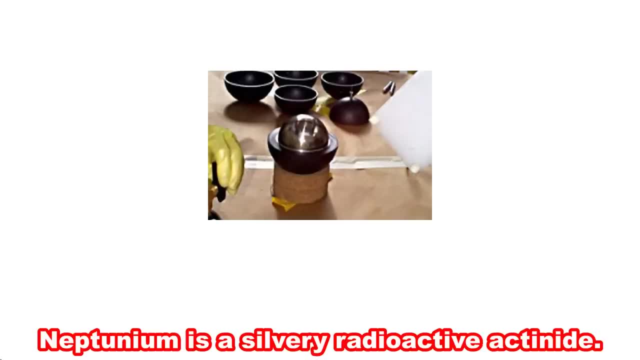 Number 93. Neptunium. Neptunium is a silvery radioactive actinide. Its minutes long. during the aku period means a sensor that starts when the sun is near side. Neptunium's current applications are limited. 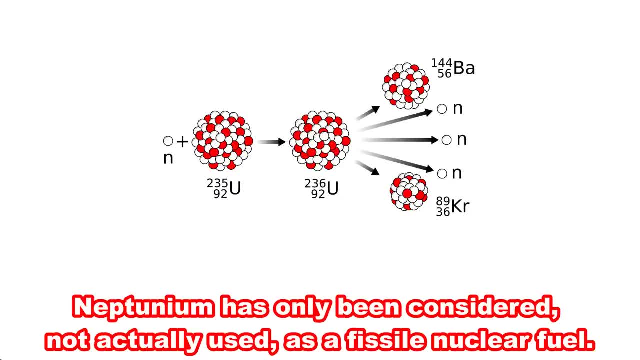 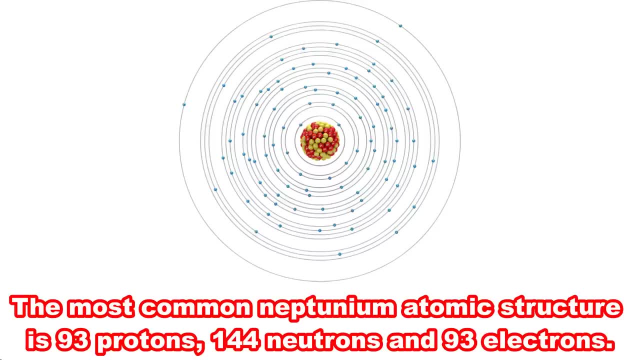 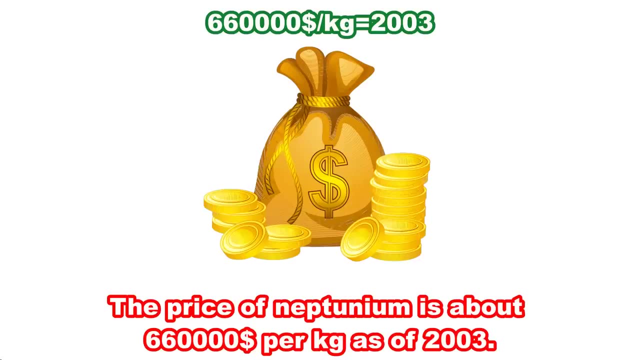 Neptunium has only been considered, not actually used, as a fissile nuclear fuel. The most common Neptunium atomic structure is 93 protons, 144 neutrons and 93 electrons. The price of Neptunium is about $660,000 per kilogram as of 2003.. 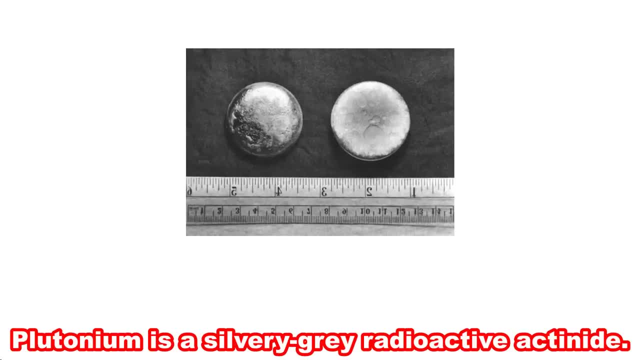 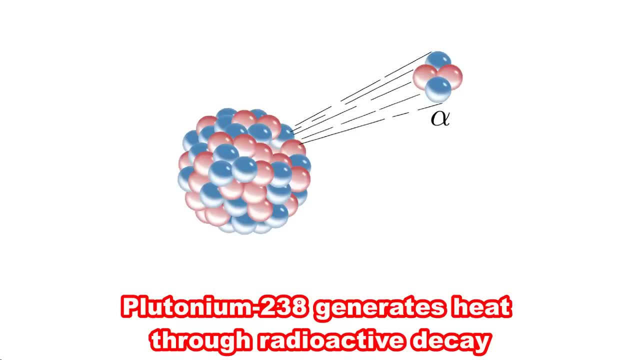 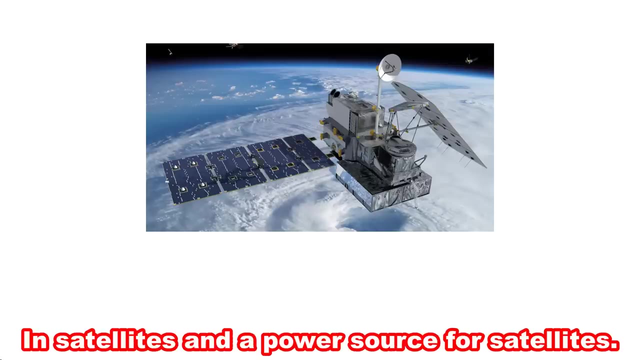 Number 94.. Plutonium. Plutonium is a silvery-gray radioactive actinide. Plutonium-238 generates heat through radioactive decay, which makes it useful as a heat source for sensitive electrical components in satellites and a power source for satellites. 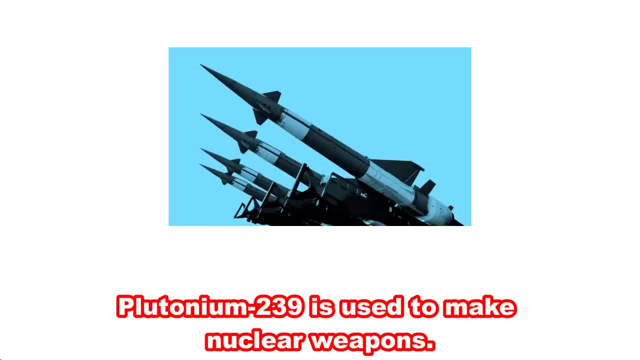 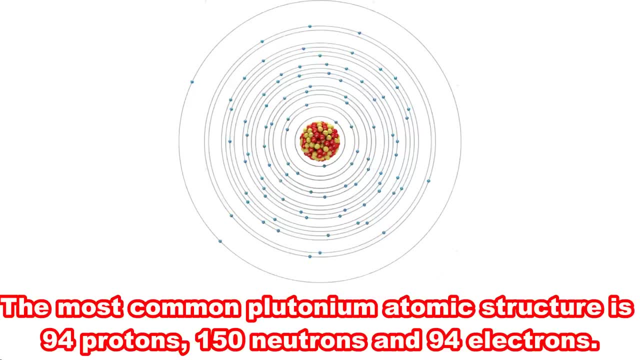 Plutonium-239 is used to make nuclear weapons. The most common Plutonium atomic structure is 94 protons, 150 neutrons and 94 electrons. The price of Plutonium-239 is about $660,000 per kilogram as of 2003.. 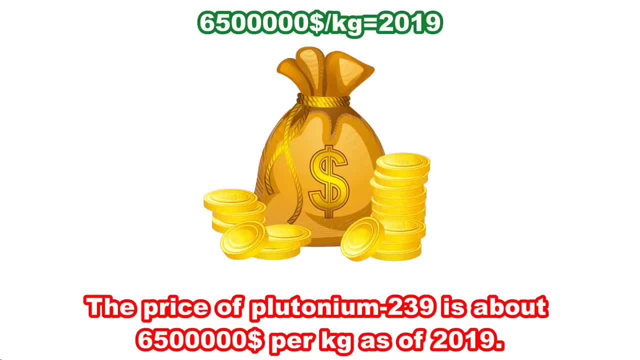 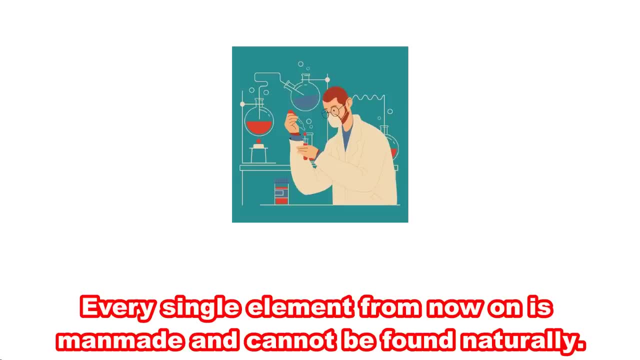 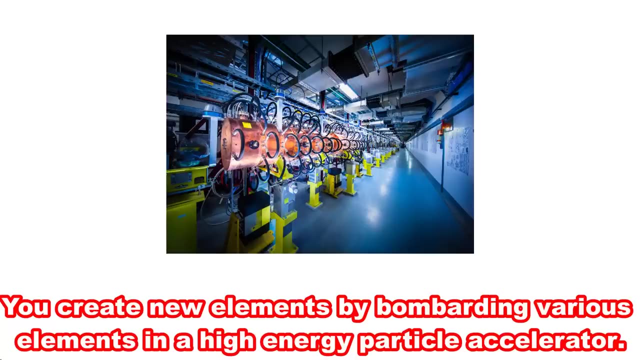 The price of Plutonium-239 is about $6,500,000 per kilogram as of 2013.. Every single element from now on is man-made and cannot be found naturally. You create new elements by bombarding various elements in a high-energy particle accelerator. 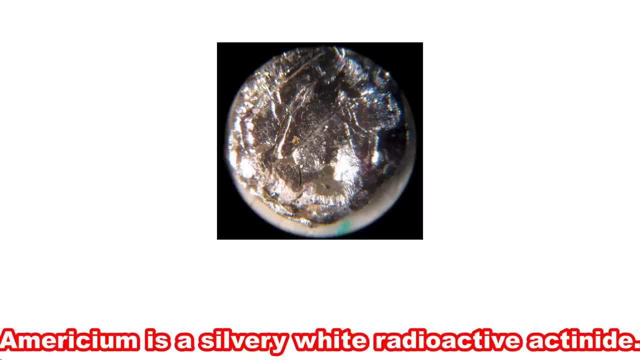 Number 95. Americium. Americium is a silvery-white radioactive actinide. Americium is used in smoke alarms, fluid density gauges and nuclear weapons. Plutonium-239 is the most common Plutonium atomic structure. 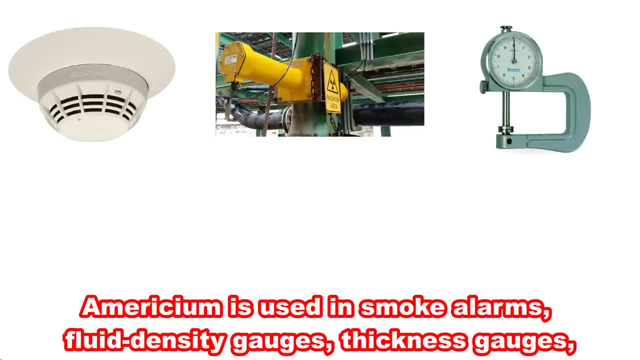 The price of Plutonium-239 is about $6,500,000 per kilogram as of 2013.. Number 95. Curium Curium is a radioactive hard dense, silvery-white nuclear weapon. The price of vakum vapur is about $7,000,000 per kilogram as of 2004.. 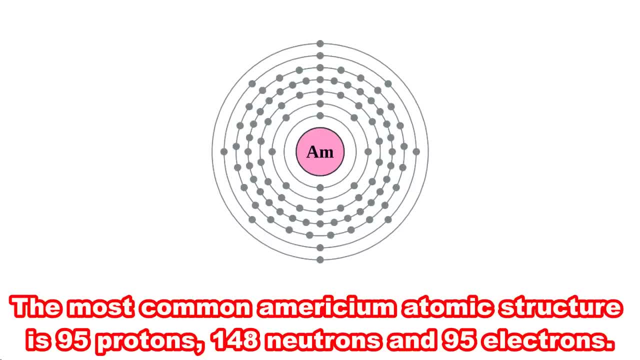 The price of vakum vapur is about $7,500,000 per kilogram as of 2004.. Number 96.. Plutonium-239 is used to make normal nuclear weapons, samen with several weapons that can be used to make launch-to-release stations, such as: firecrackers, safety-cars and air-firing missiles. It is called a Plutonium atomic structure because it is heavy and heavy and is able tolynium-239 to downsize a weapon and is capable of destroying any weapon. 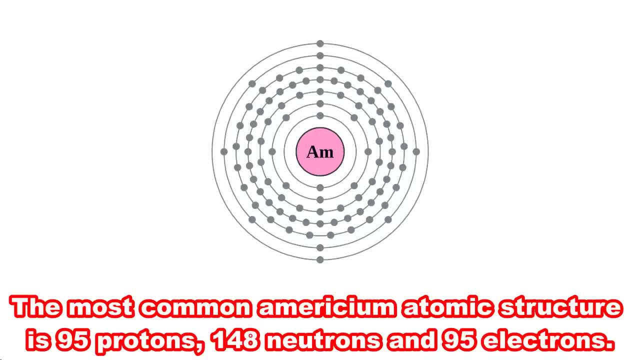 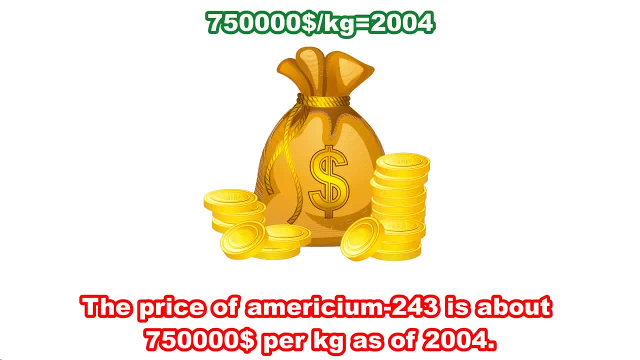 However, it is still very high. that is why it is called a Plutonium atomic structure: 148 neutrons and 95 electrons. The price of americene-243 is about $750,000 per kilogram as of 2004.. 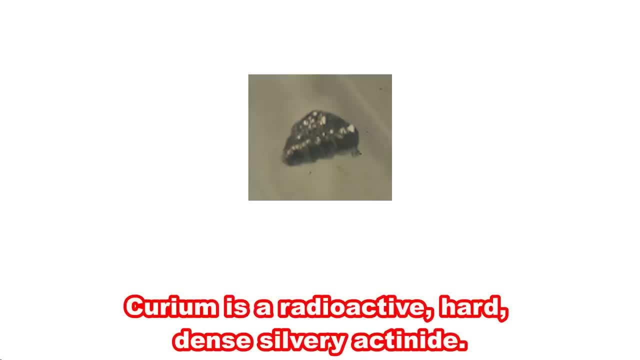 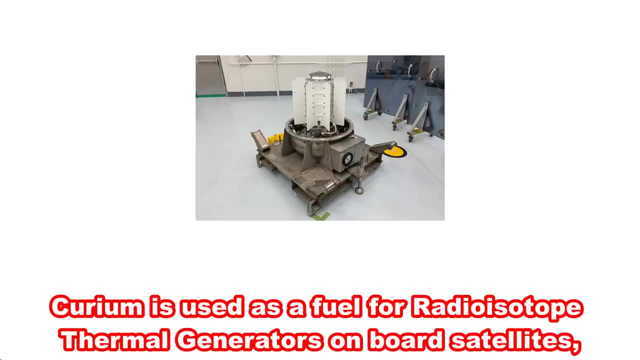 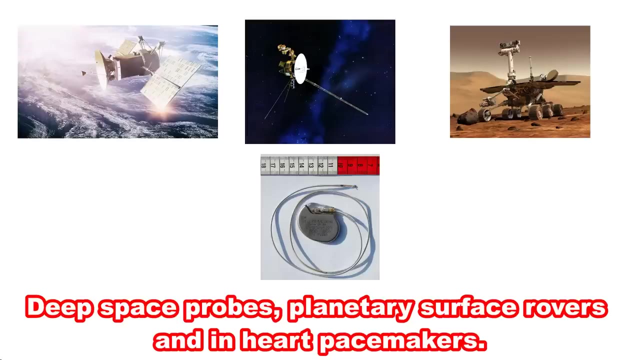 Number 96.. Curium. Curium is a radioactive, hard dense silver reactinide. Curium is used as a fuel for radioisotope thermal generators on board satellites, deep space probes, planetary surface rovers and in-heart pacemakers. 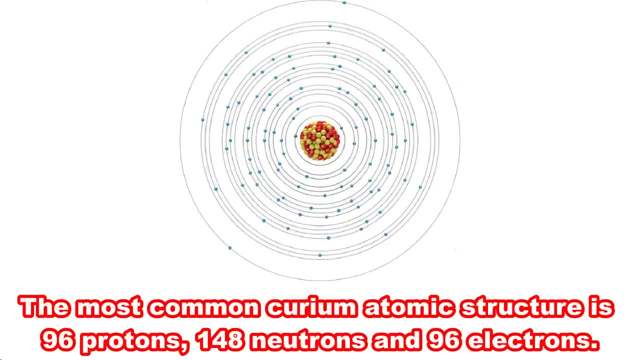 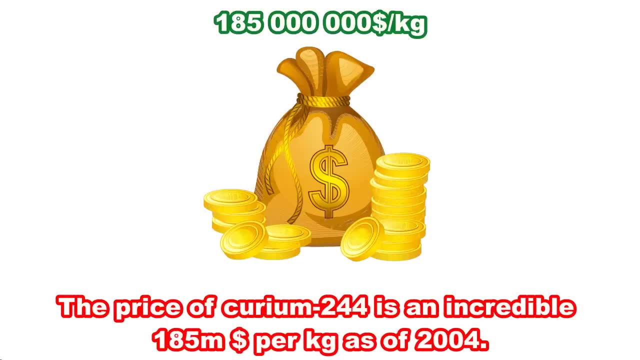 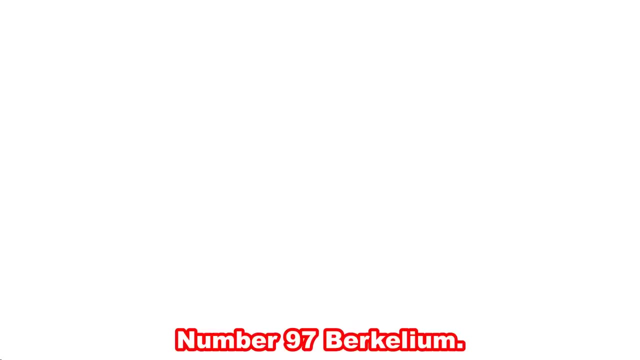 The most common curium atomic structure is 96 protons, 148 neutrons and 96 electrons. The price of curium-244 is an incredible $185,000,000 per kilogram as of 2004.. Number 97.. 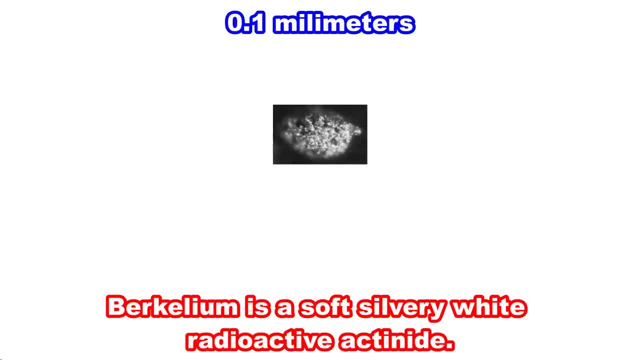 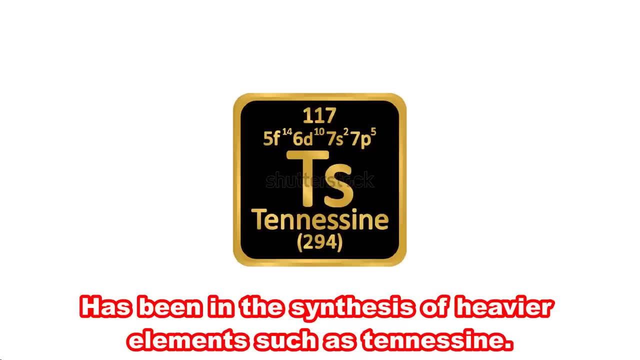 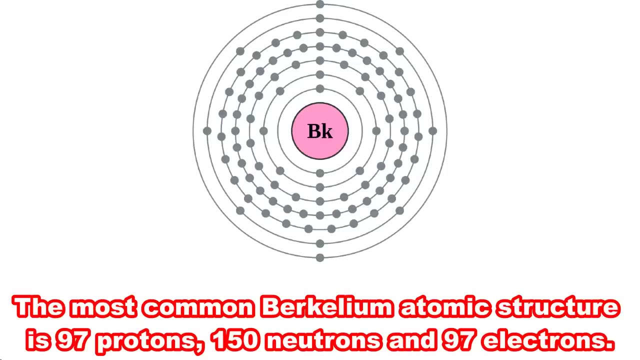 Bacillium. Bacillium is a soft, silvery, white radioactive actinide. The only use of Bacillium has been in the synthesis of heavier elements such as Tennessene. The most common Bacillium atomic structure is 97 protons, 150 neutrons and 97 electrons. 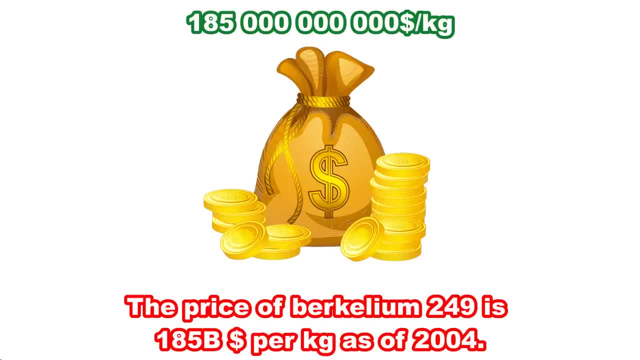 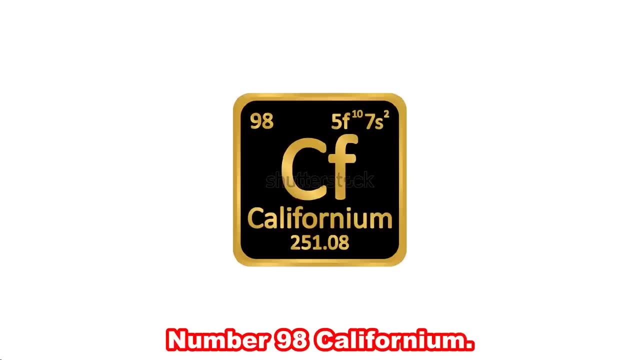 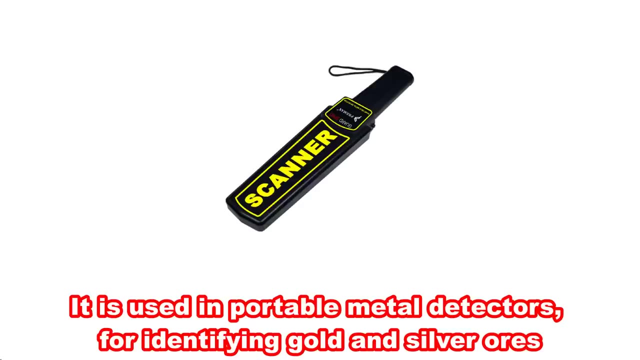 The price of Bacillium-249 is $185,000,000 per kilogram as of 2004.. Number 98. Californium. Californium is a silvery radioactive actinide. It is used in portable metal detectors for identifying gold and silver ores, and also. 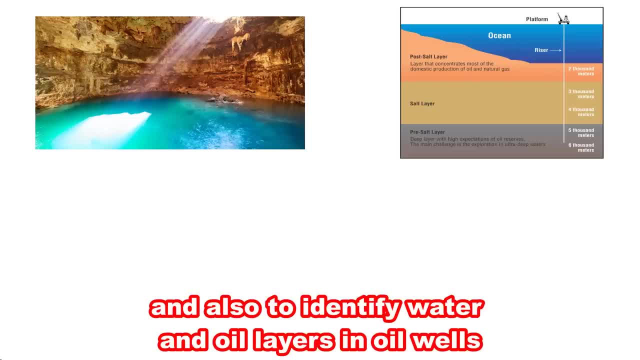 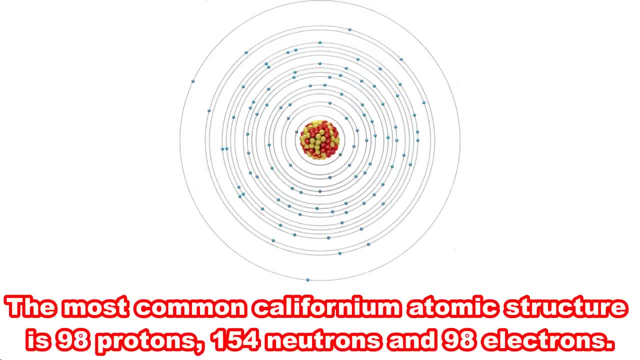 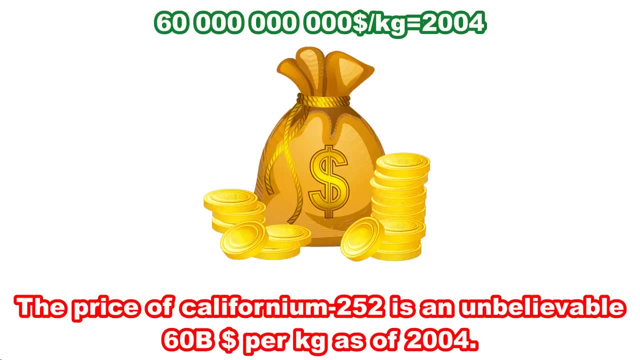 to identify water and oil layers in oil wells And to detect metal fatigue and stress in aeroplanes. The most common Californium atomic structure is 98 protons, 154 neutrons and 98 electrons. The price of Californium-252 is an unbelievable $60,000,000,000 per kilogram as of 2004.. 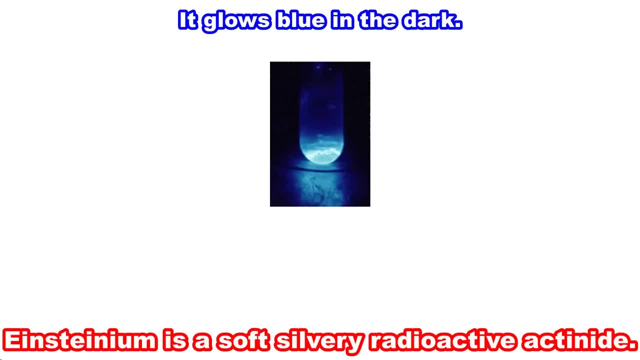 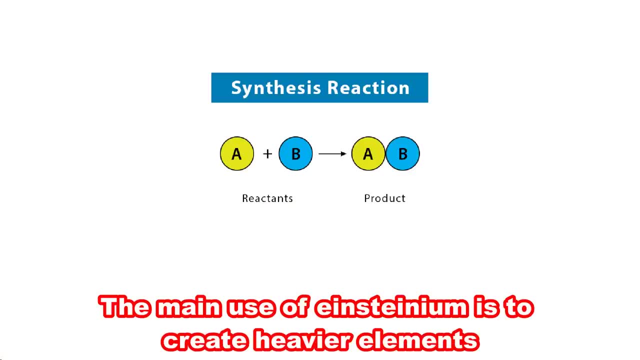 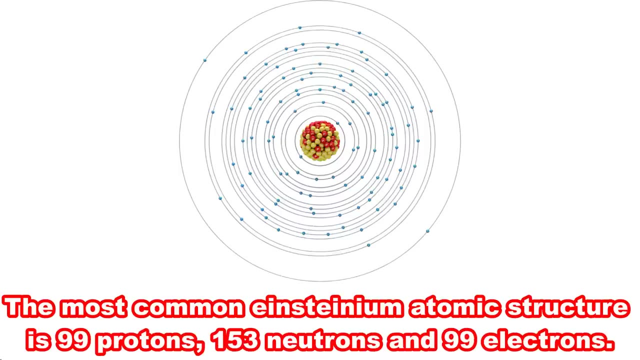 Number 99. Einsteinium. Einsteinium is a soft, silvery radioactive actinide. The main use of Einsteinium is to create heavier elements, including Mendelevium, and also for research. The most common Einsteinium atomic structure is 99 protons, 153 neutrons and 99 electrons. 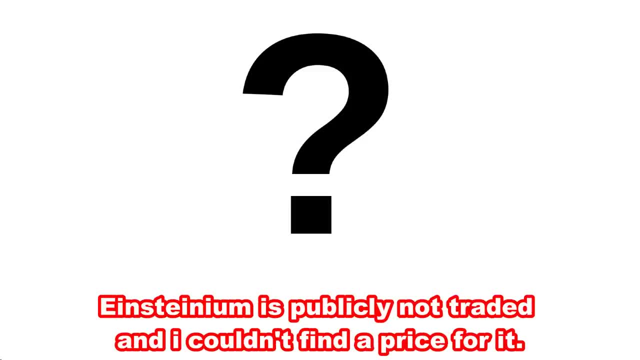 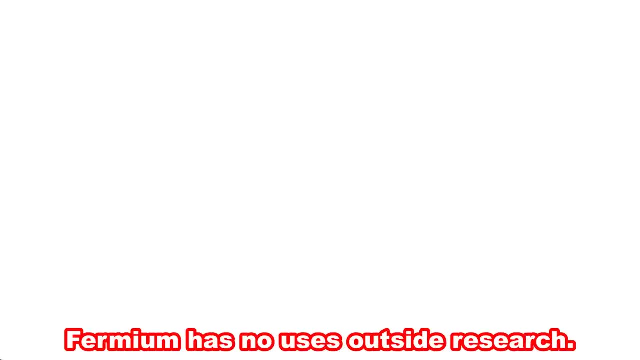 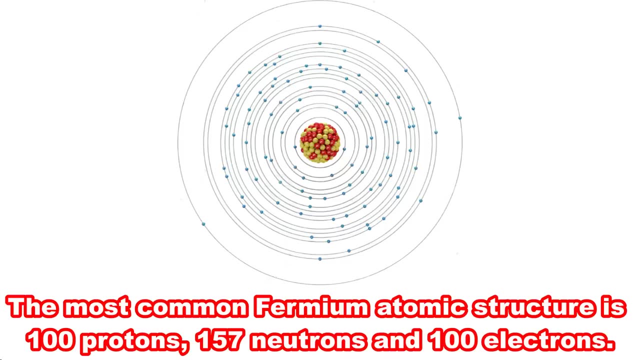 Einsteinium is publicly not traded and I couldn't find a price for it. Number 100. Fermium: Fermium is a radioactive actinide. Fermium has no use as outside research. The most common Fermium atomic structure is 100 protons, 157 neutrons and 100 electrons. 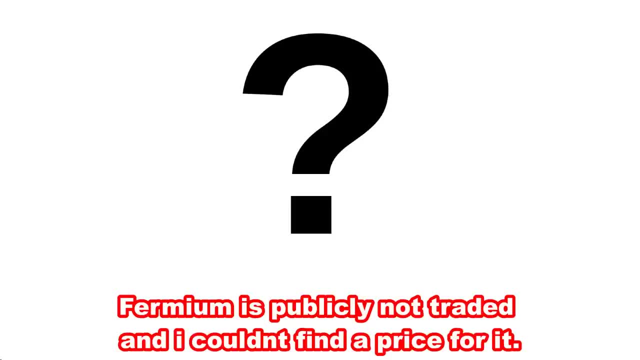 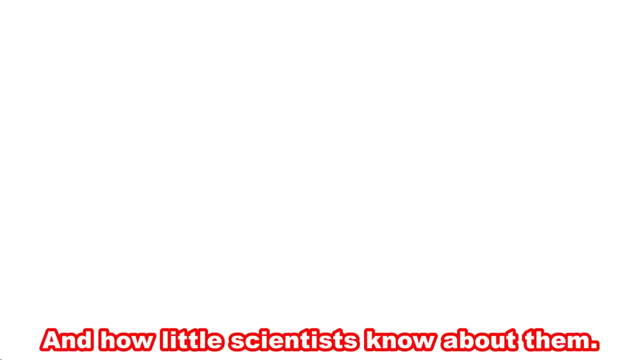 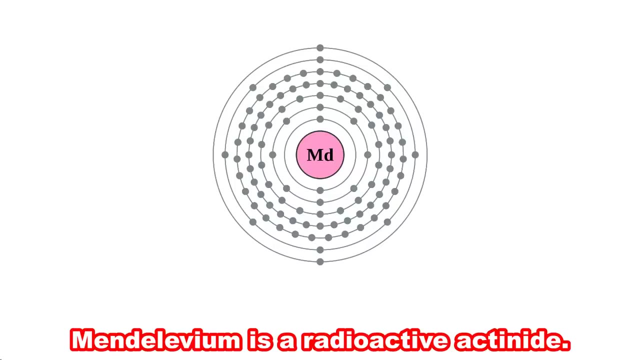 Fermium is publicly not traded and I couldn't find a price for it. A lot of the elements we have left won't have anything special about them because of their very short half-life and how little scientists know about them. Number 101.. Mendelevium. 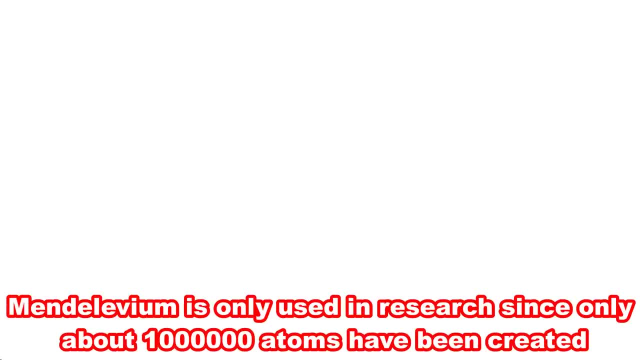 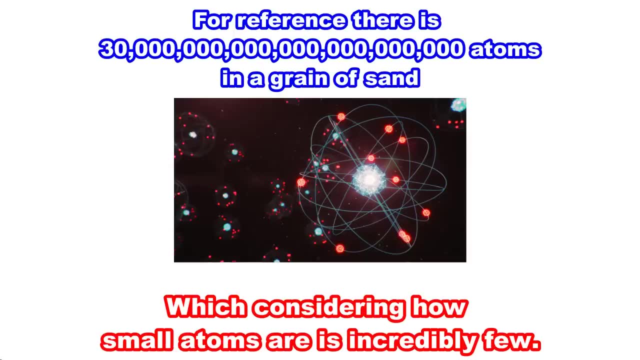 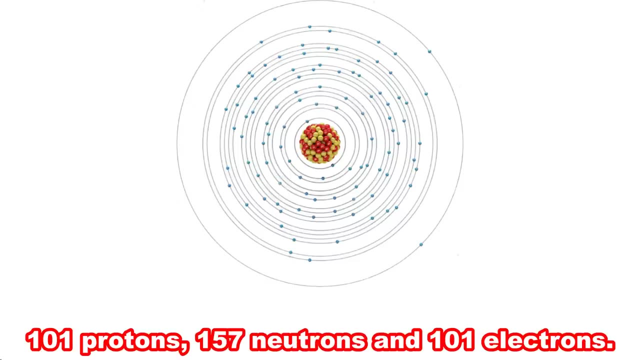 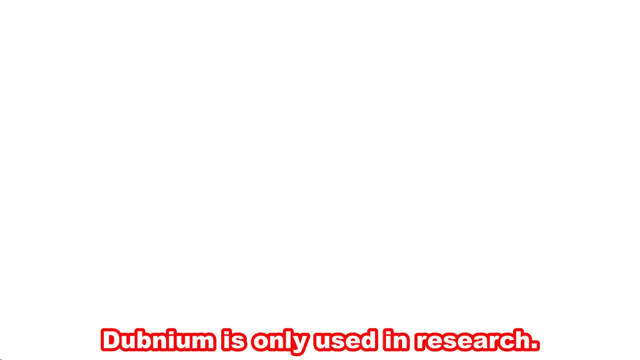 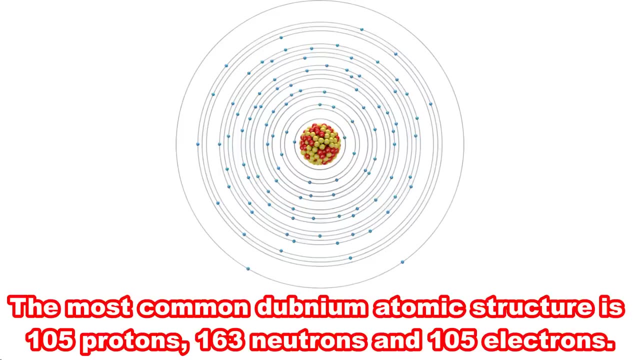 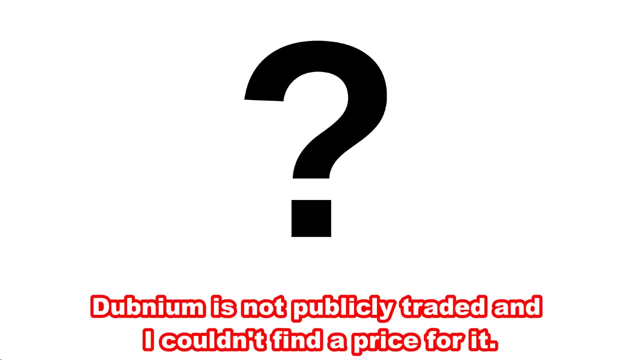 The highly radioactive transition metal, Dubnium, is only used in research. The most common Dubnium atomic structure is 105 protons, 163 neutrons and 105 electrons. Dubnium is not publicly traded and I couldn't find a price for it. 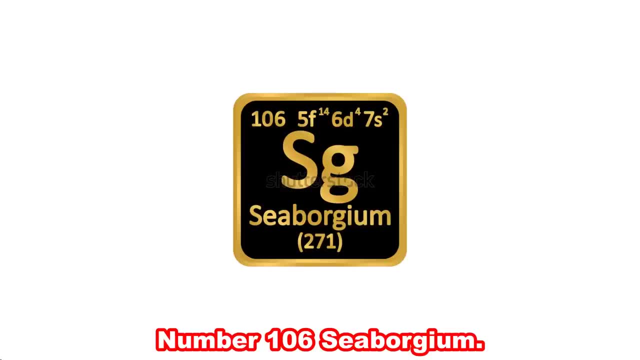 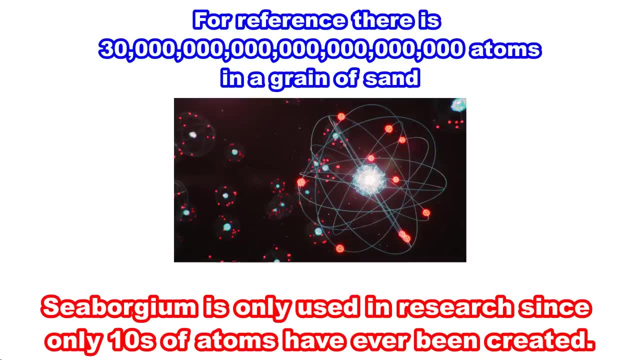 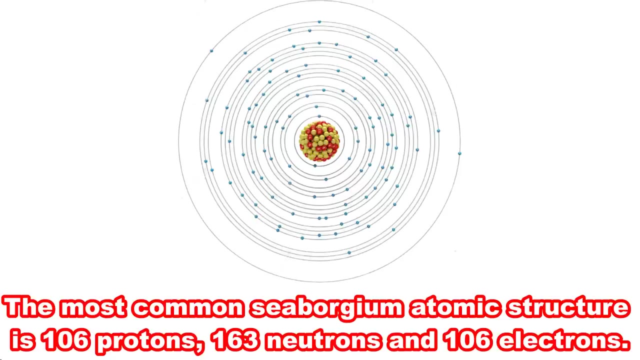 Number 106.. Cyborgium. Cyborgium is a radioactive transition metal. Cyborgium is only used in research, Since only tens of atoms have ever been created. The most common Cyborgium atomic structure is 106 protons, 163 neutrons and 106 electrons. 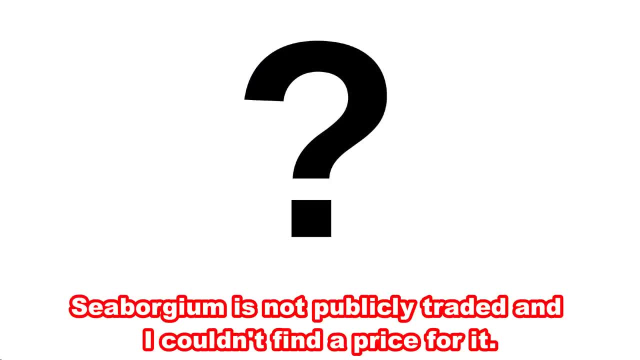 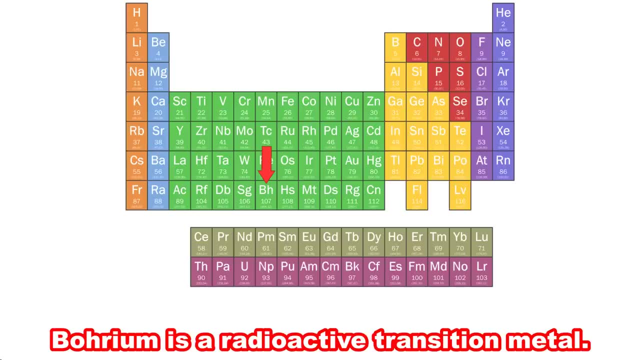 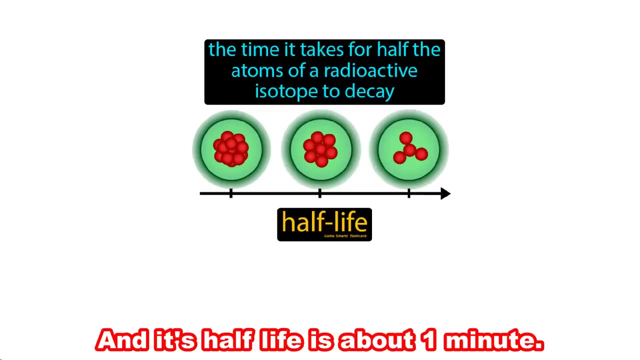 Cyborgium is not publicly traded and I couldn't find a price for it. Number 107.. Borium. Borium is a radioactive transition metal. Borium is only used in research, Since only tens of atoms have been created And its half-life is about 1 minute. 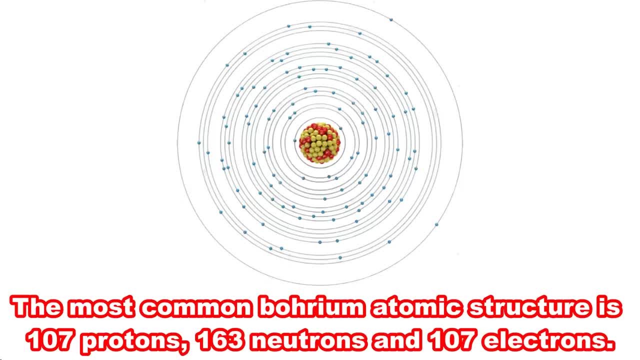 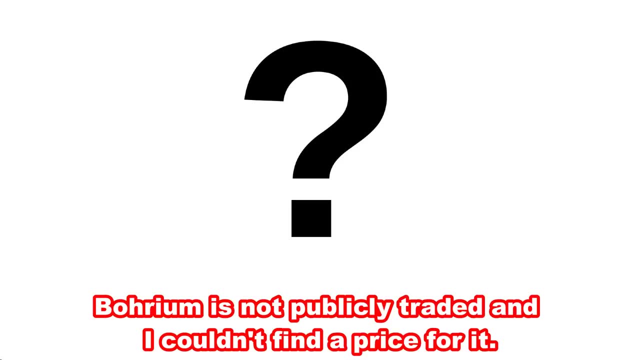 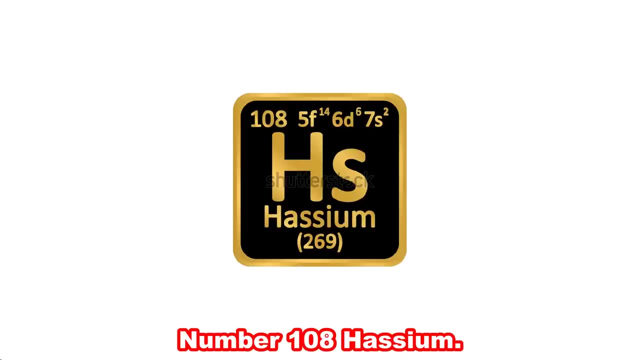 The most common Borium atomic structure is 107 protons, 163 neutrons and 107 electrons. Borium is not publicly traded and I couldn't find a price for it. Number 108. Hassium: Hassium is a highly radioactive transition metal. 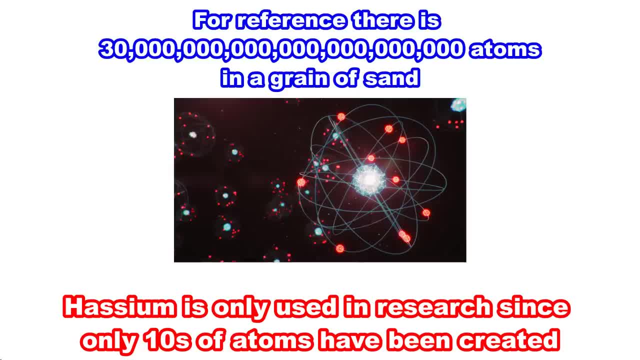 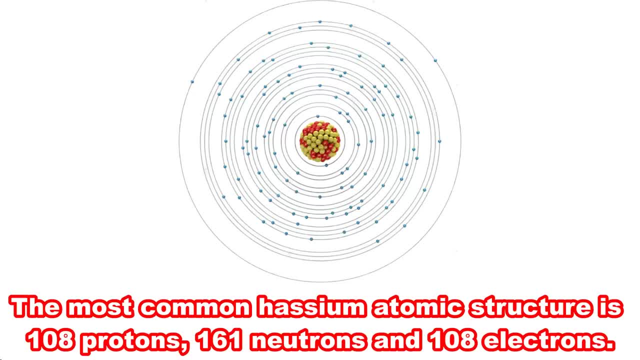 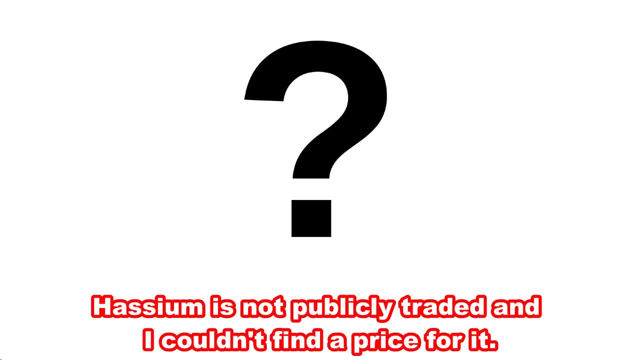 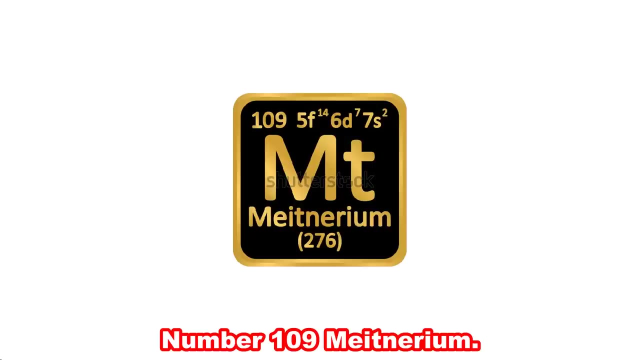 Hassium is only used in research, Since only tens of atoms have been created And its half-life is about 15 minutes. The most common Borium atomic structure is 108 protons, 161 neutrons and 108 electrons. hasium is not publicly traded and I couldn't find a price for it. 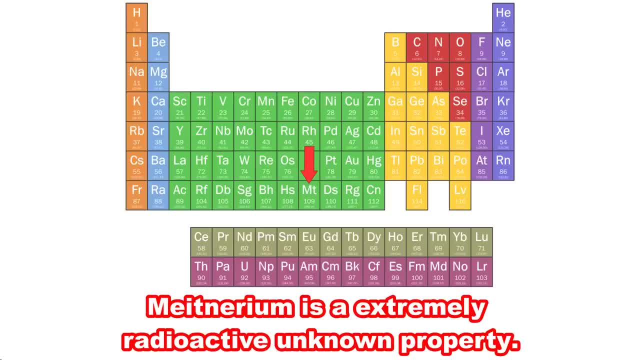 Number 109.. Mitenerium. Mitenerium is a extremely radioactive, unknown property. Mitenerium is only used in research, Since only a few atoms have been created And its half-life is about 1 second. The most common Hassium atomic structure is 108 protons, 161 neutrons and 108 electrons. 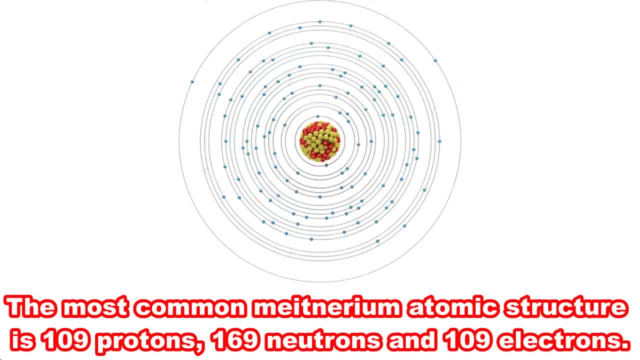 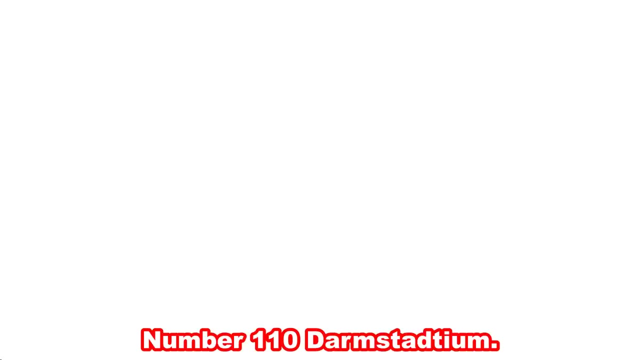 life is about 1 second. The most common mitonarium atomic structure is 109 protons, 169 neutrons and 109 electrons. Mitonarium is not publicly traded and I couldn't find a price for it. Number 110.. Darmstatium. Darmstatium is an extremely radioactive unknown. 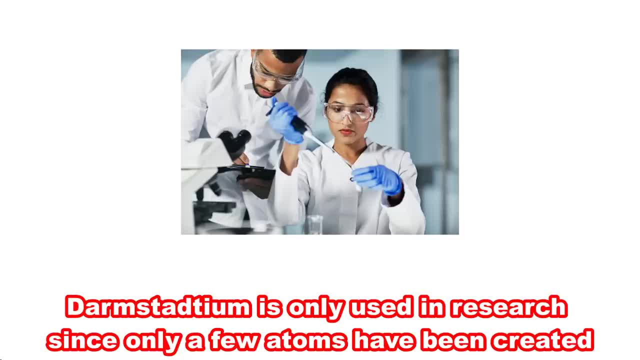 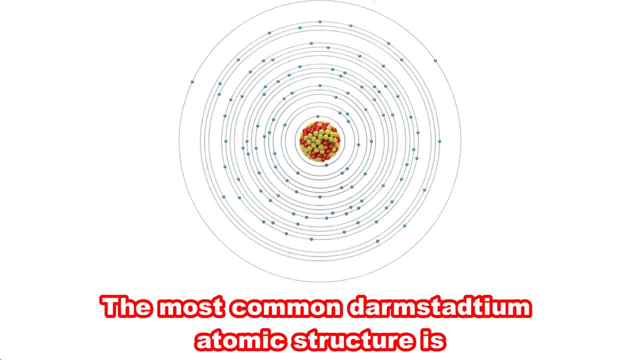 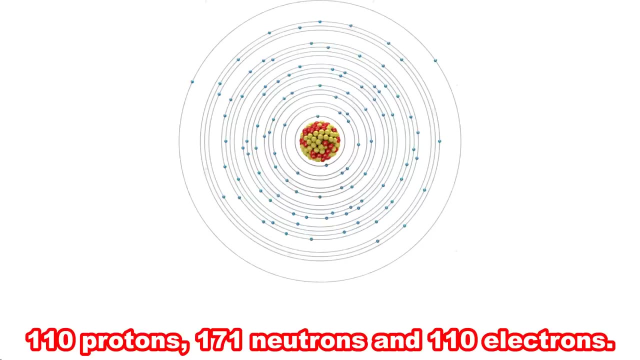 property. Darmstatium is only used in research, since only a few atoms have been created and its half-life is about 10 seconds. The most common Darmstatium atomic structure is 110 protons, 171 neutrons and 110 electrons. Darmstatium is not publicly traded and I couldn't find 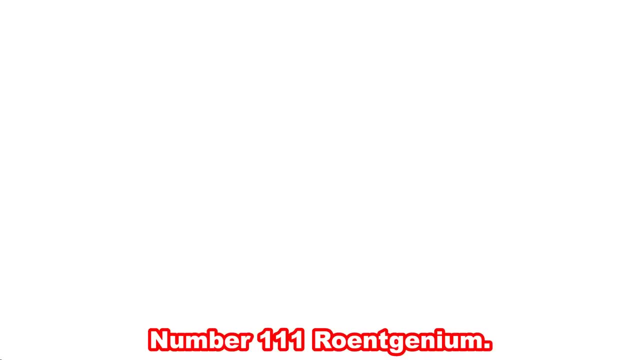 a price for it. Number 111.. Runtgenium. Runtgenium is an extremely radioactive, unknown property. Runtgenium is only used in research, since only a few atoms have been created and its half-life is about 10 seconds. The most common Darmstatium atomic 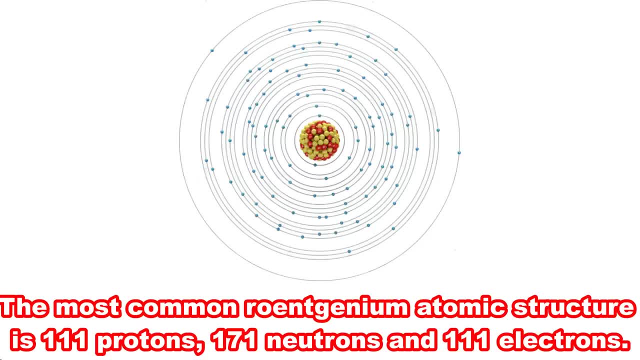 structure is 108 protons, 172 neutrons and 119 electrons. The most common Runtgenium atomic structure is 110 protons, 171 neutrons and 119 electrons. The most common Runtgenium atomic structure is 112 protons, 171 neutrons and 119 electrons. 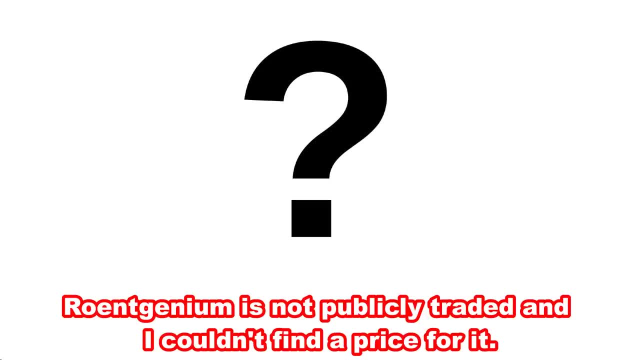 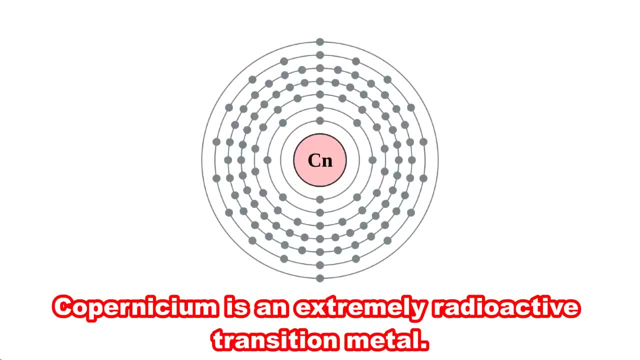 Runtgenium is not publicly traded and I couldn't find a price for it. Number 112. Copernicium. Copernicium is an extremely radioactive transition. middle Copernicium is only used in research, since only a few atoms have been created, and only 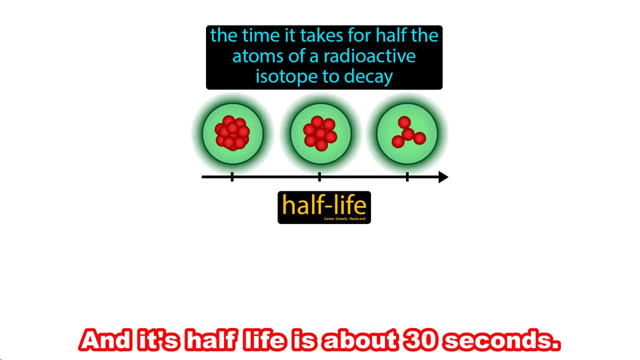 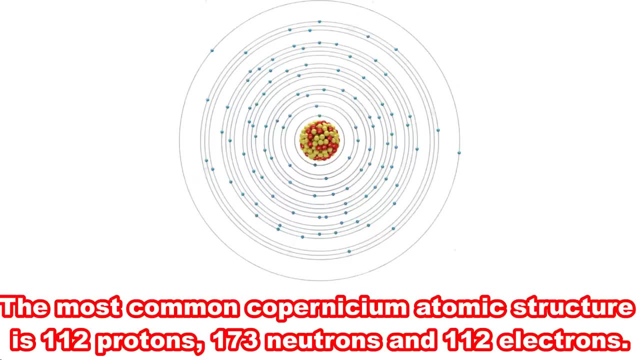 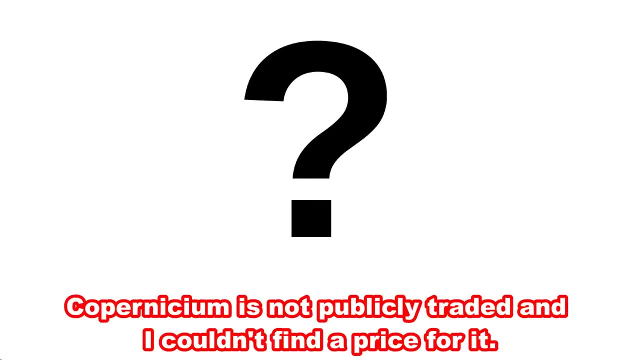 tens of atoms have been created. created and its half-life is about 30 seconds. The most common Copernicium atomic structure is 112 protons, 173 neutrons and 112 electrons. Copernicium is not publicly traded and I couldn't. 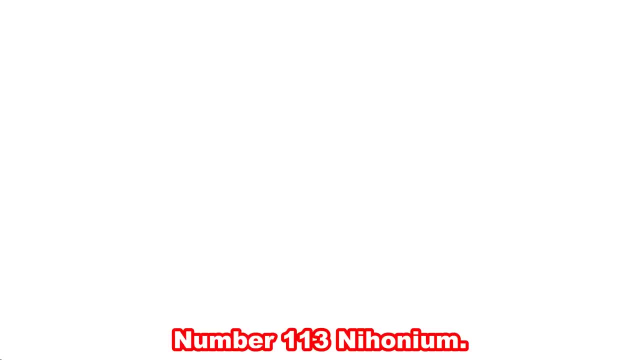 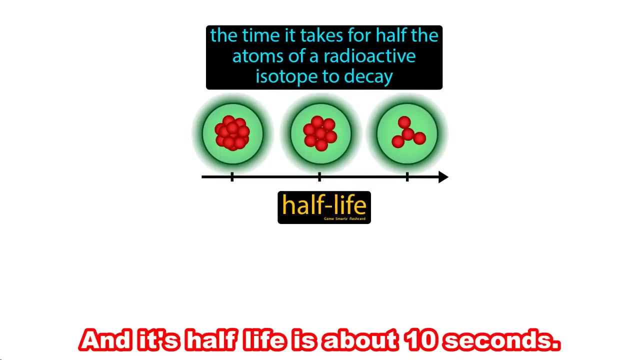 find a price for it. Number 113.. Nihonium: Nihonium is an extremely radioactive, unknown property. Nihonium is only used in research, since less than 100 atoms have been created and its half-life is about 10 seconds. The most common 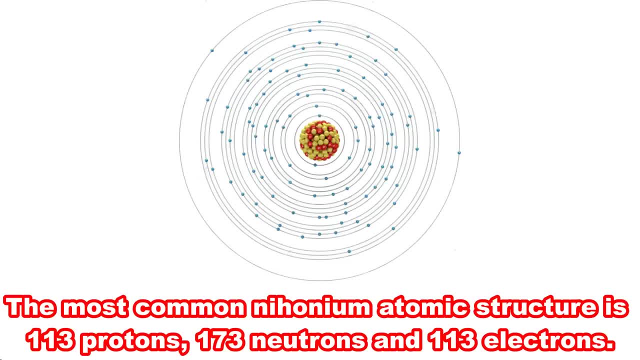 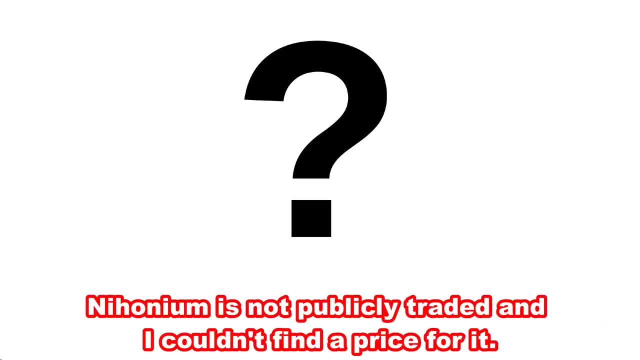 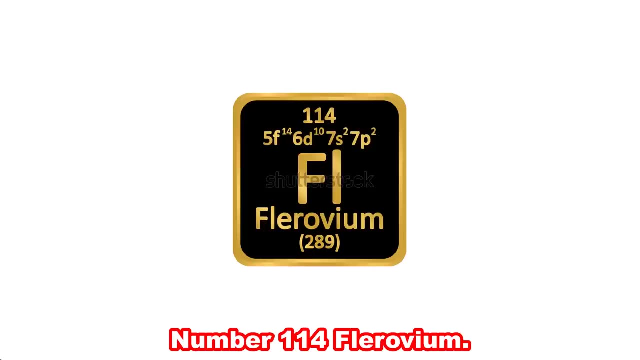 Nihonium atomic structure is 113 protons, 173 neutrons and 113 electrons. Nihonium is not publicly traded and I couldn't find a price for it. Number 114. Fluorovium. Fluorovium is an extremely radioactive, unknown property. Fluorovium is only used in research and research. Nihonium is only used in research and research. Fluorovium is an extremely radioactive, unknown property. Fluorovium is only used in research and research. Nihonium is only used in research and research. Nihonium is only used in research, since. 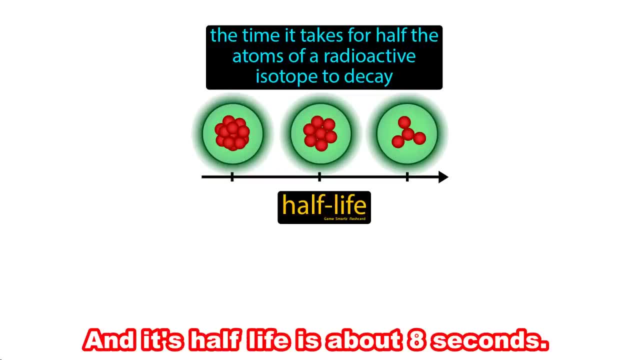 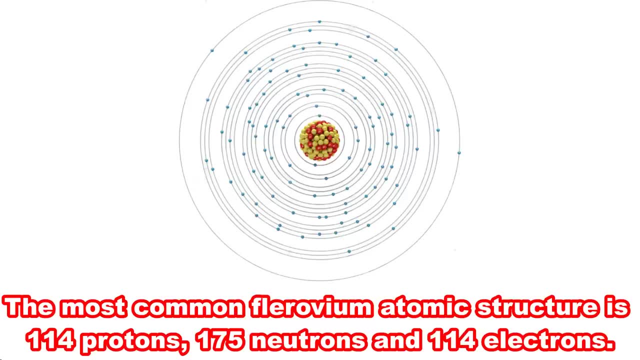 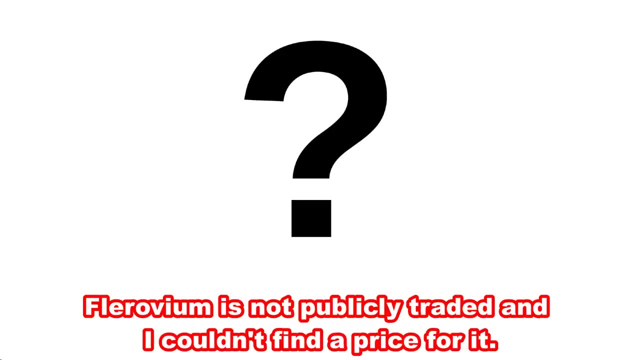 less than 100 atoms have been created and its half-life is about 8 seconds. The most common Fluorovium atomic structure is 114 protons, 175 neutrons and 114 electrons. Fluorovium is not publicly traded and I couldn't find a price for it- Number 115.. Moscovium. 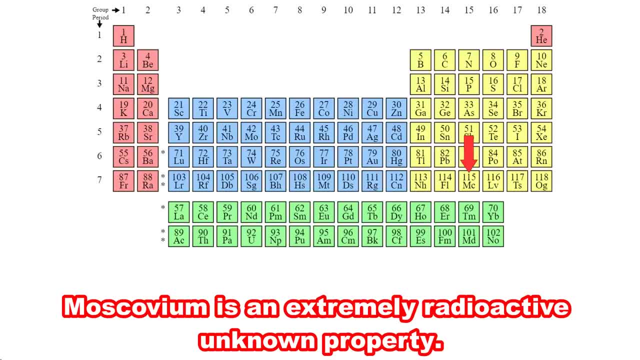 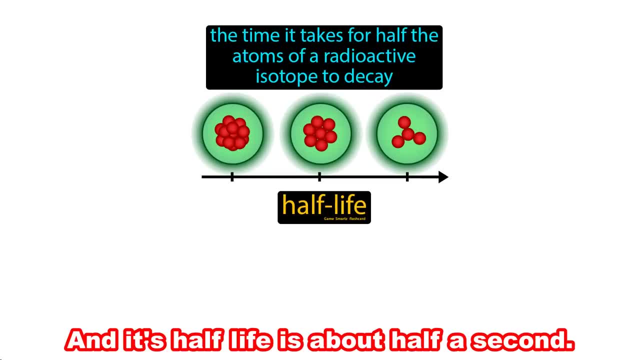 Moscovium is an extremely radioactive, unknown property. Moscovium is only used in research, since less than 100 atoms have been created and its half-life is about half a second. The most common Moscovium atomic structure is 115 protons. 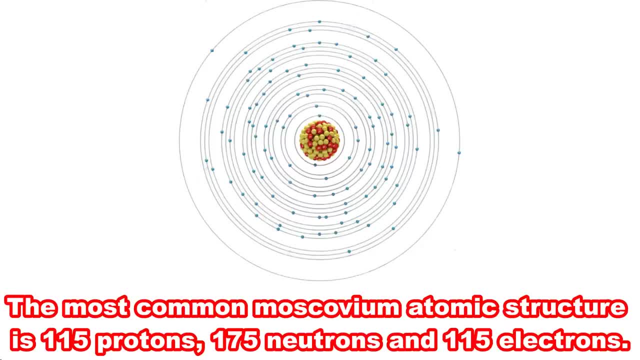 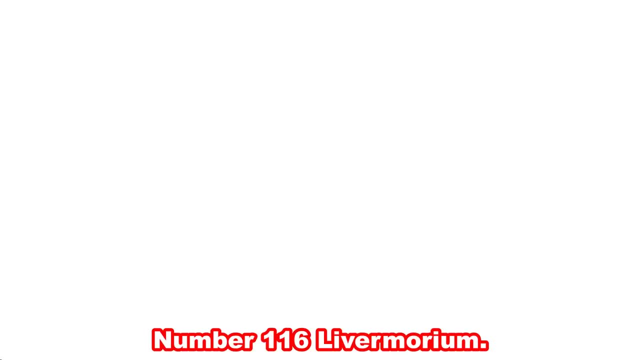 175 neutrons and 115 electrons. Moscovium is not publicly traded and I couldn't find a price for it. Number 116.. Livermorium: Livermorium is an extremely radioactive unknown property. Livermorium is an extremely radioactive, unknown property. Livermorium is an extremely radioactive. 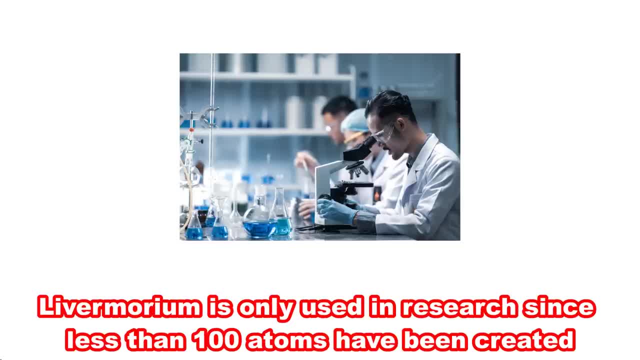 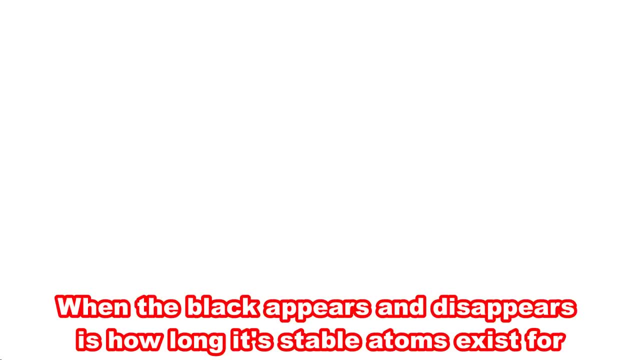 unknown property. Livermorium is only used in research, since less than 100 atoms have been created and its half-life is about 50 milliseconds. When the black appears and disappears is how long its stable atoms exist, for That is how short-lived it is. The most common Livermorium atomic structure. 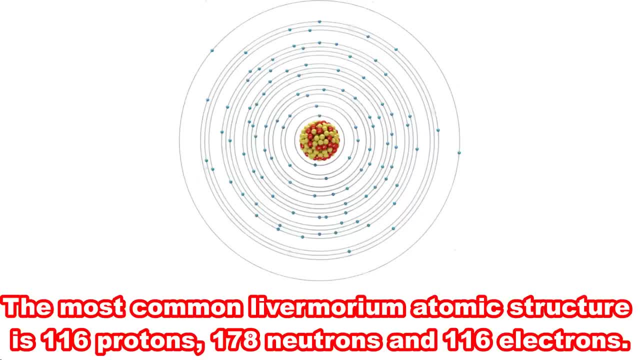 is 116 protons, 178 neutrons and 116 electrons Number 117. Nihonium. Nihonium is an extremely radioactive, unknown property. Livermorium is not publicly traded and I couldn't find a price for it. Moscovium is not publicly traded and I couldn't find a price for it. Livermorium is not publicly traded and I couldn't find a price for it. Livermorium is not publicly traded and I couldn't find a price for it. Livermorium is not publicly traded and I couldn't find a price for it. Nihonium is an extremely radioactive, unknown property. Livermorium is only used in research, since less than 100 atoms have been created and its half-life is about 50 milliseconds. and again, this is how fast it is. 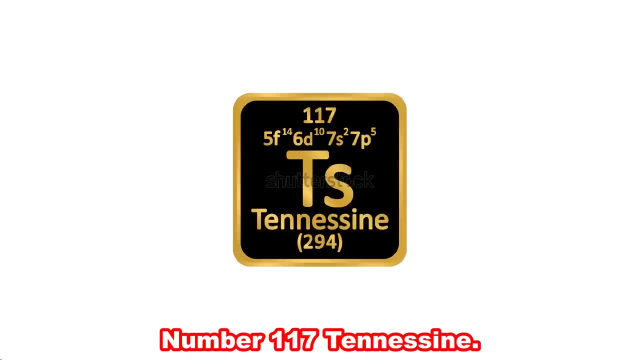 Livermorium is an extremely radioactive unknown property. Livermorium is only used in research, since less than 100 atoms have been created and its half-life is about 50 milliseconds. and again, this is how fast it is. Livermorium is an extremely radioactive unknown property. Livermorium is an extremely radioactive, unknown property. 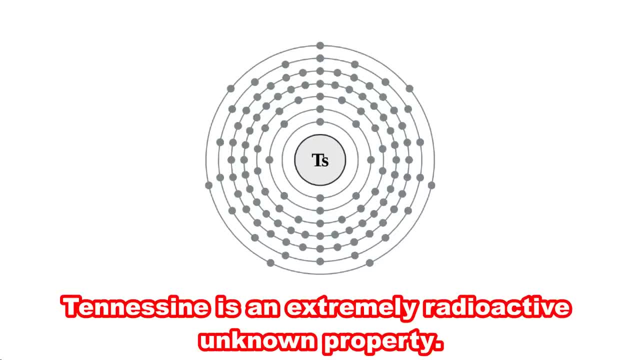 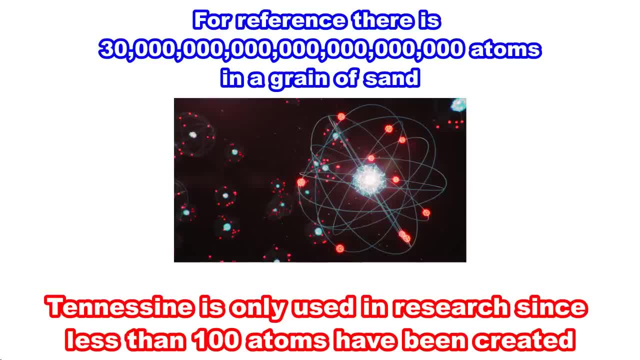 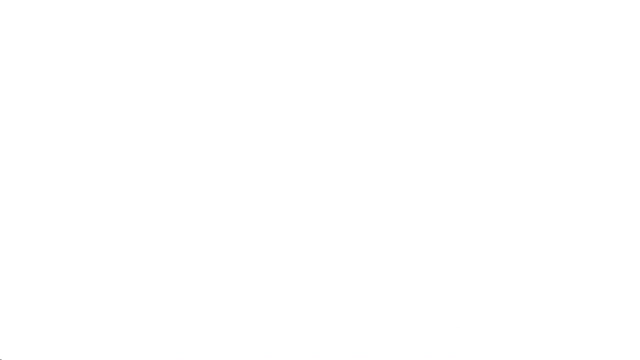 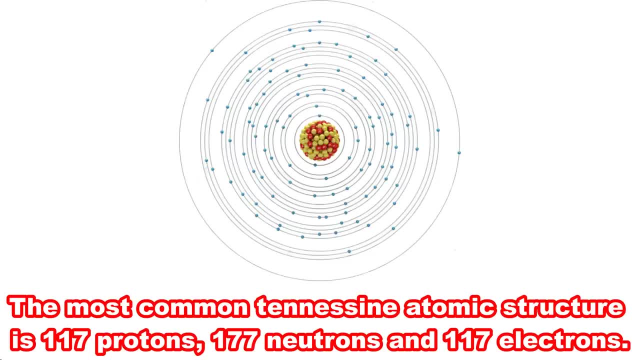 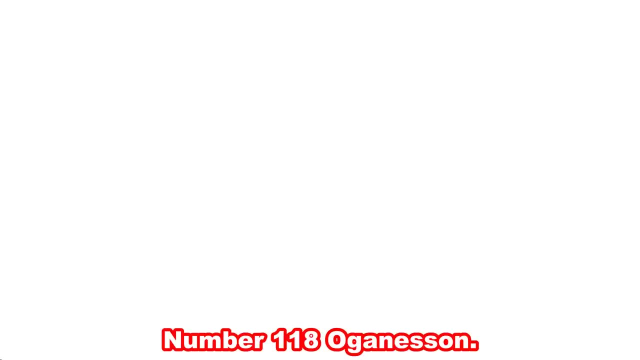 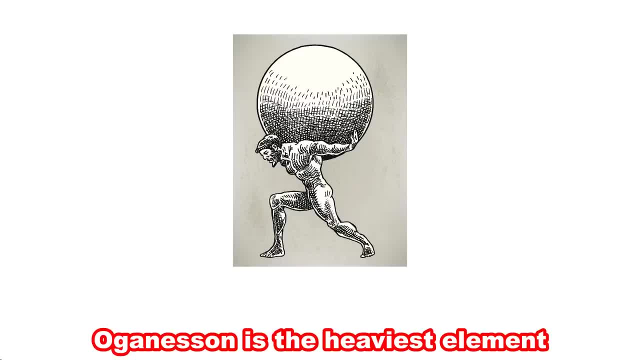 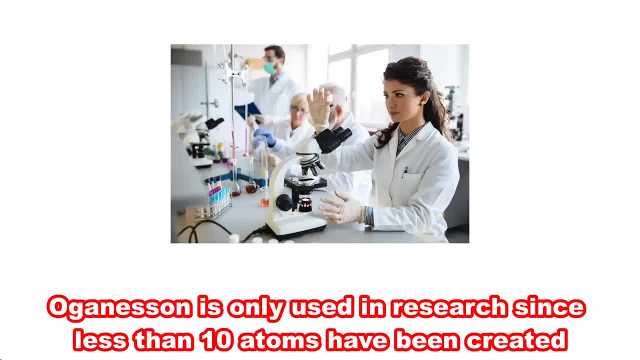 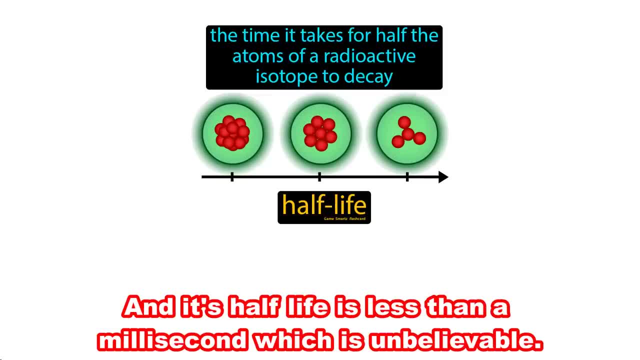 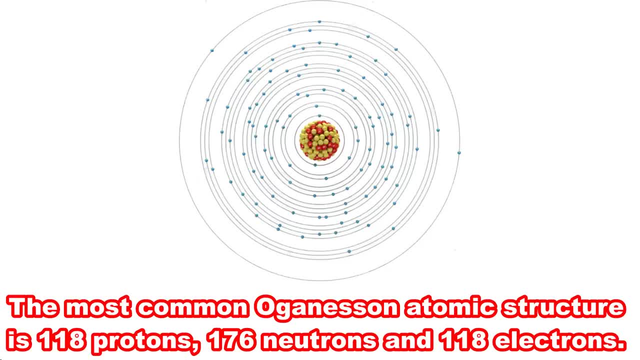 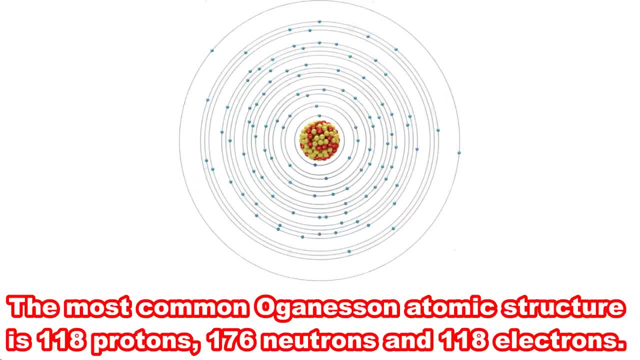 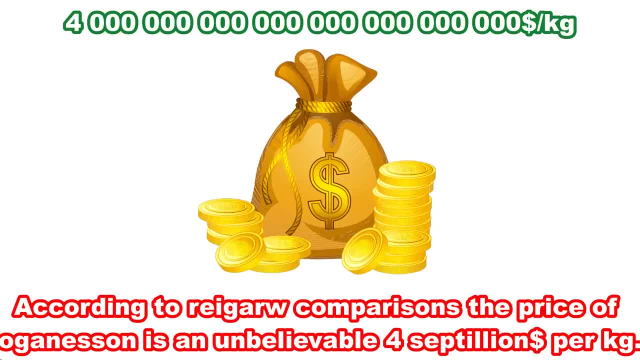 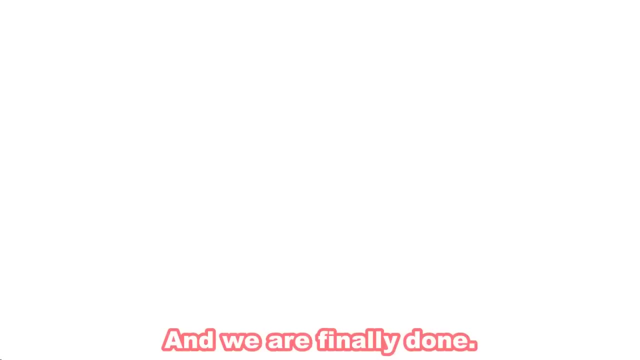 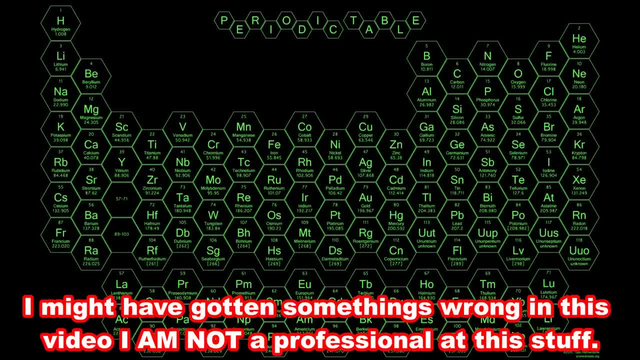 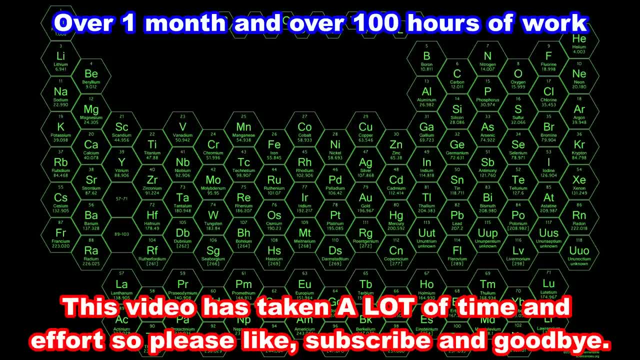 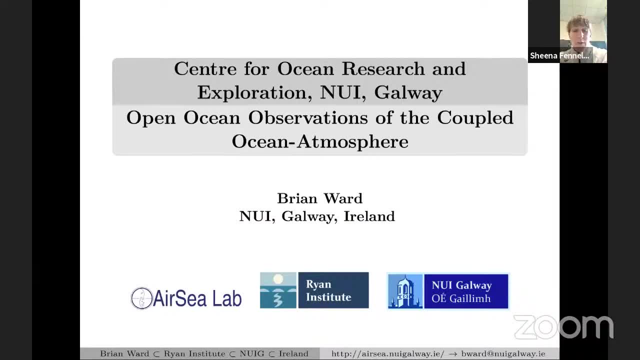 I'll just give a couple of minutes there for everyone to join in. My name is Sheena Fennell and I am hosting this webinar today, So we'll just give a couple of minutes there and we'll get going with Dr Brian Ward's presentation. 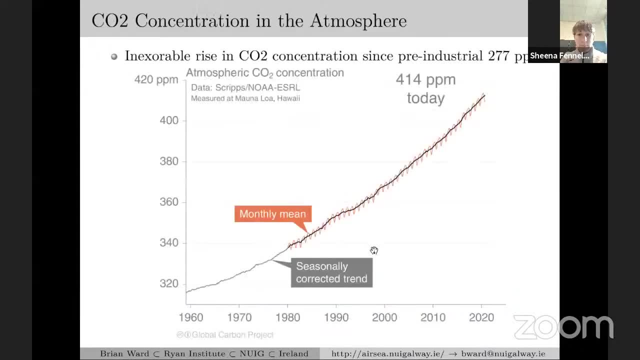 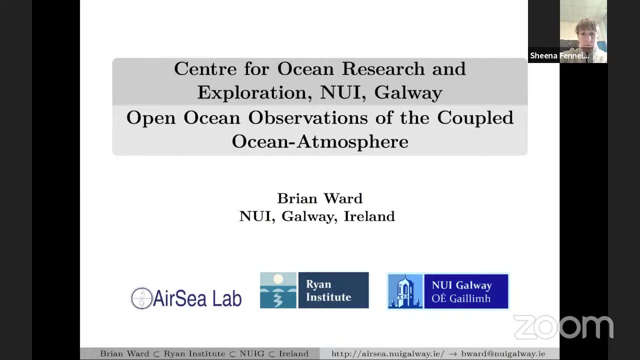 Okay, so welcome everyone to CORE-X's seminar series, as we've just started for this year. And it's CORE-X- for those of you that haven't heard of us- is the Centre of Ocean Research and Exploration here in NUIG in Galway. 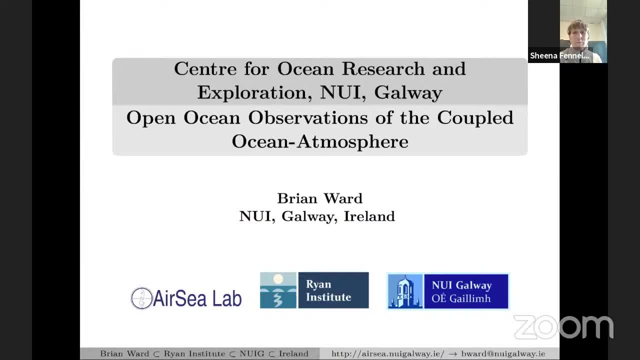 And it's a basically brings together all of the PIs that are involved with any marine research, And so, without further ado, we'll go on to our guest speaker, which is Dr Brian Ward. He is a senior lecturer here in the School of Natural New School of Natural Sciences.